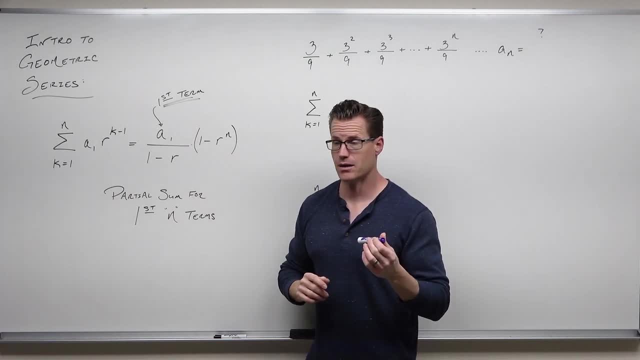 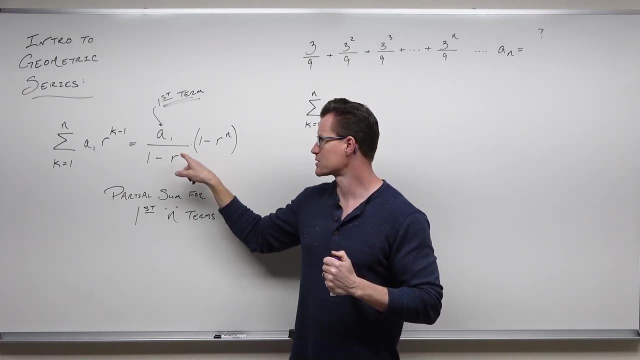 r and multiply times one minus r to the n, whatever that n is. Also, you might notice at this point that most textbooks show this differently. Most textbooks have a sub one and then this divided by that. I'm not doing that. I'm not doing it for a very specific reason that you're going to see. 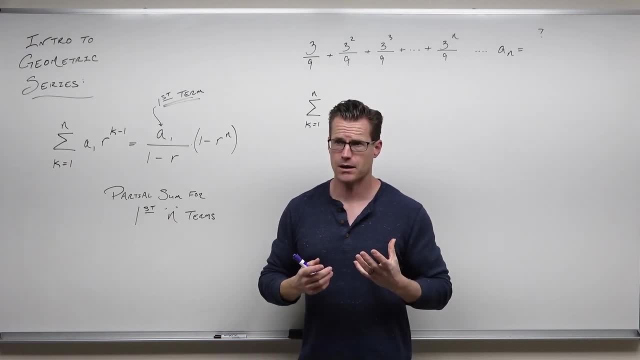 when we get to infinite series in the last half of this video. So we'll talk about infinite series. You know what do you mean? Can we add up the terms of a series forever and get something out Wildly? the answer is: sometimes, Not all the time, but if our common ratio is between a certain two, 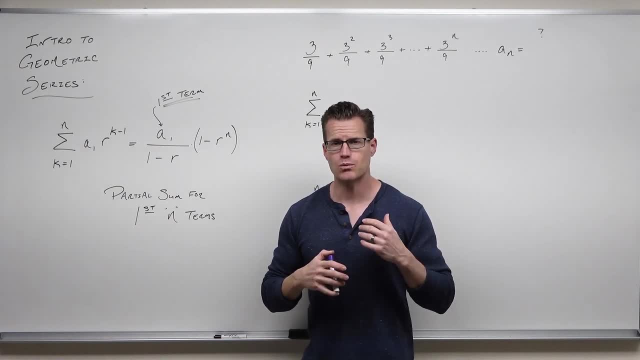 numbers negative one to one. the answer is yes, it converges, It will add up to a certain value. It's very fascinating. You're all very smart and you've made this far. You're going to be just fine. Some of your brains are going to hurt a little. 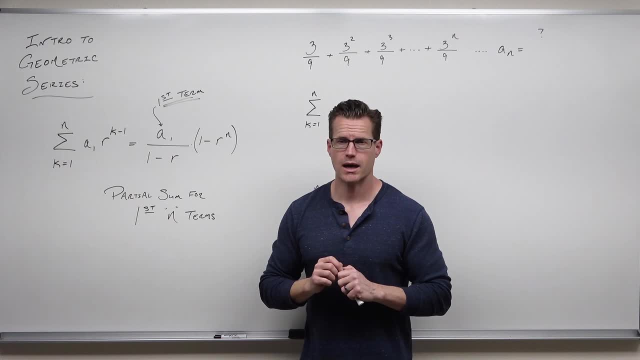 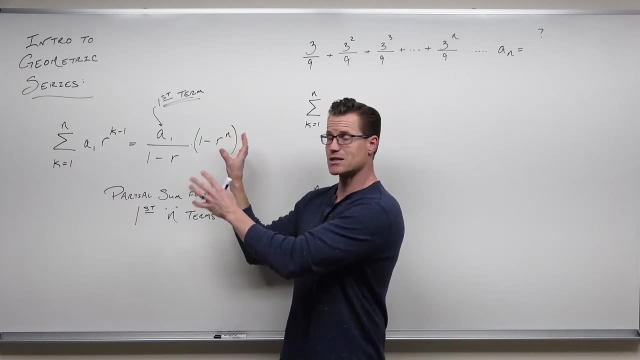 A little bit, because we're going to talk about taking a value to infinity, And sometimes it hurts our heads when we talk about infinity. so much So I'm going to teach that to you, but this is going to be much better for that. 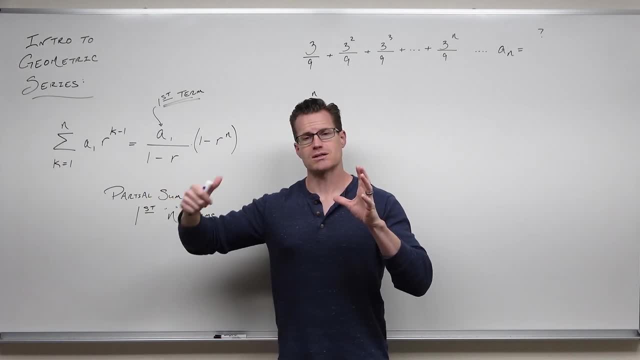 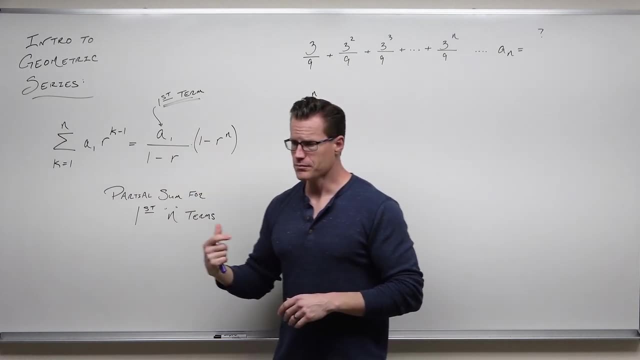 So what we're learning is we're taking a geometric sequence as a common ratio and a starting value. We're adding the terms up, and this is the formula for how to do that. So what we're going to do is we're going to take that series. This is a geometric sequence. 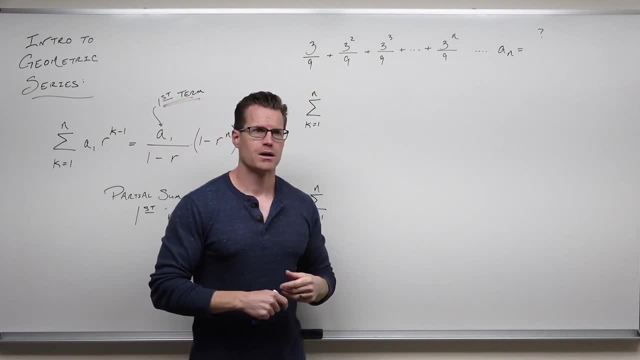 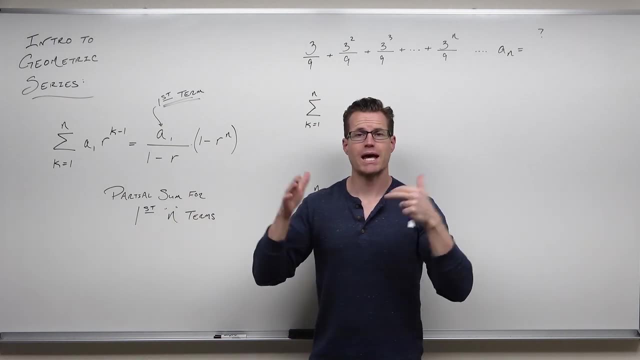 Maybe you can see it- and we're going to add up the terms terms. Well, now, what we get out of that, when we add it up, is called a partial sum. Why partial? Well, because you're adding for the first n terms, You're not adding to infinity, and therefore we 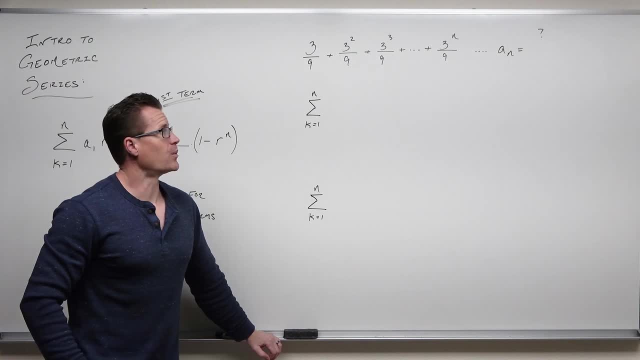 consider that a partial sum. So let's take a look at this example Now. firstly, how do we determine whether something is geometric, at least a sequence on what the series is built, or not? Well, we have to have a starting term. We see that 3, 9ths and conveniently they haven't re-simplified it made. 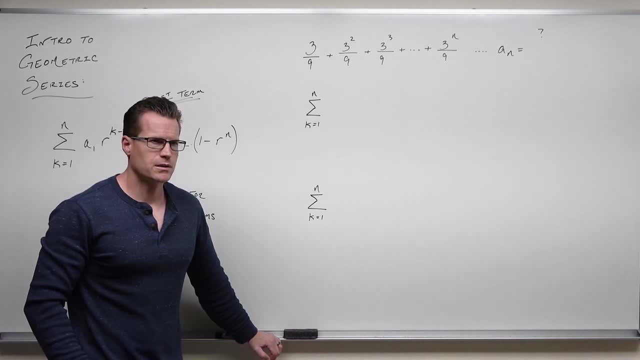 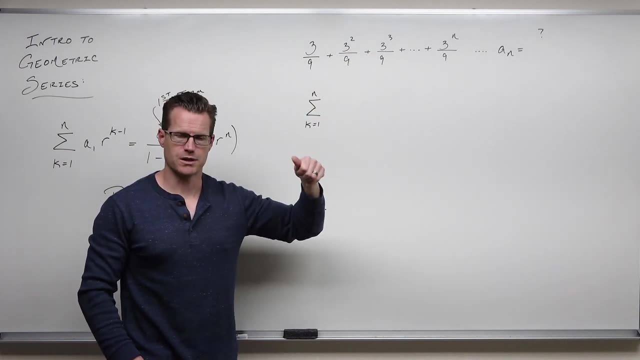 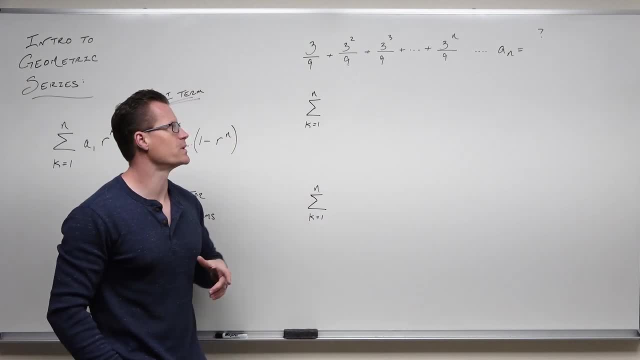 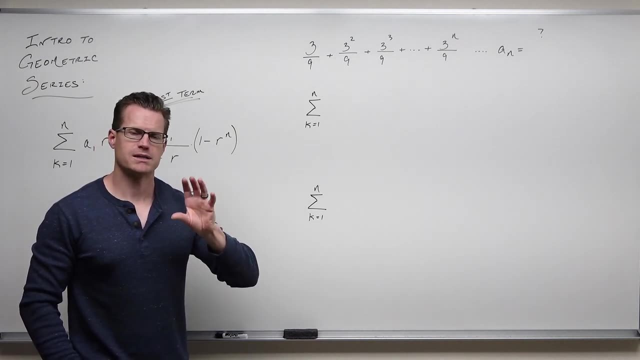 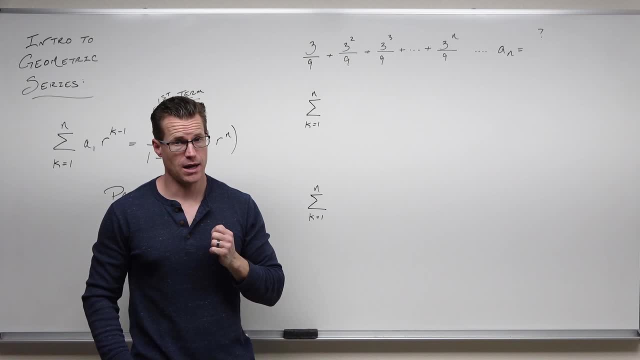 with a term that's based on n. you do not have a lot of work to do. Your sequence is 3 to the n over 9.. You go wait a minute. is that easy It is. You don't have to do the. 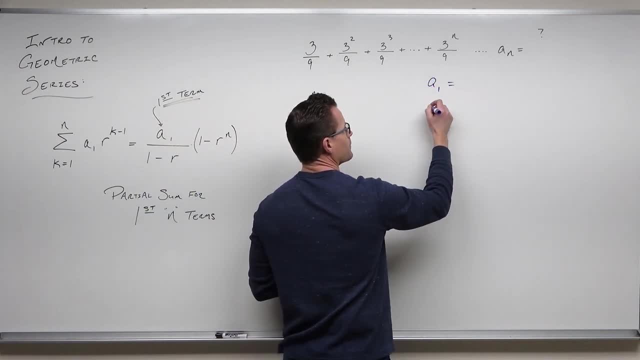 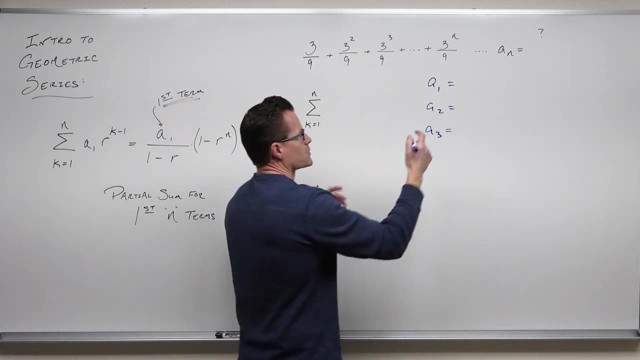 following: If you do, if you repeat what I showed you a long time ago with your sequences, you go. well, what's the first term? First term is 3- 9ths and the second term is 3 squared over 9,. 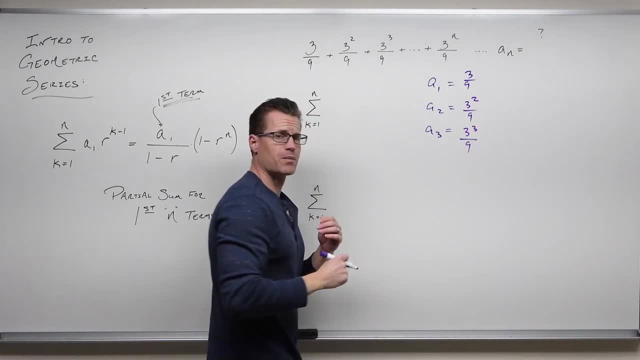 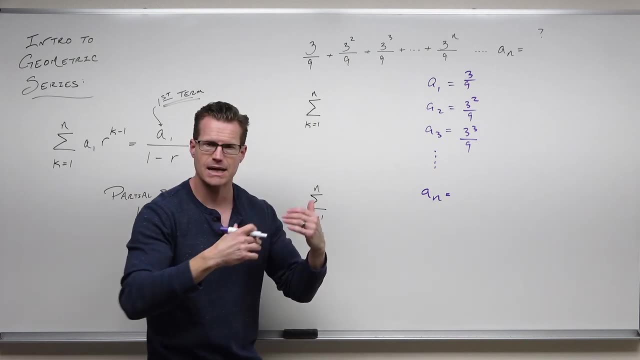 and the third term is 3 cubed over 9.. And if you remember that the whole goal was to get down to what the nth term is, It's to get down to that, And what we did a long time ago is we said: okay. 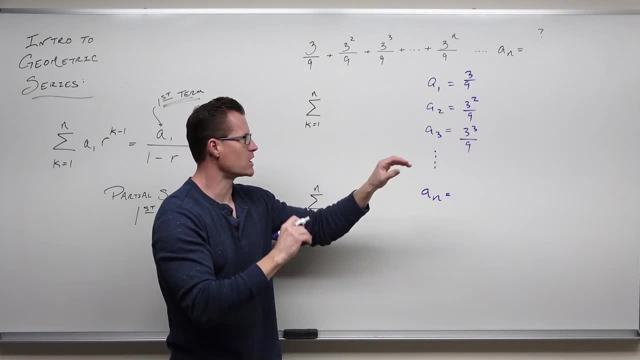 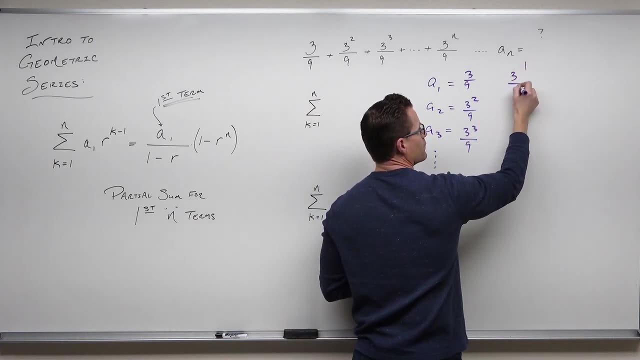 well, what's not changing? Remember, we wanted the same form: find out what's not changing. What's not changing? Well, the 3 is not changing and the 9 is not changing. So this would be 3 to the 1st over 9, and 3 to the 2nd over 9, and 3 to the 3rd over 9.. And we'd say whatever's not. 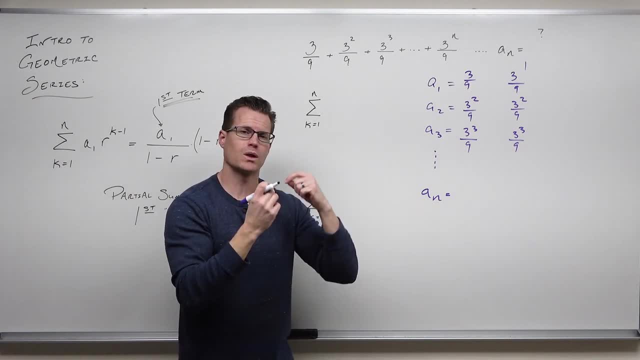 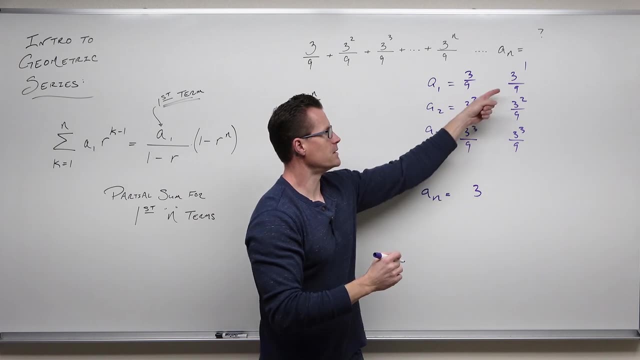 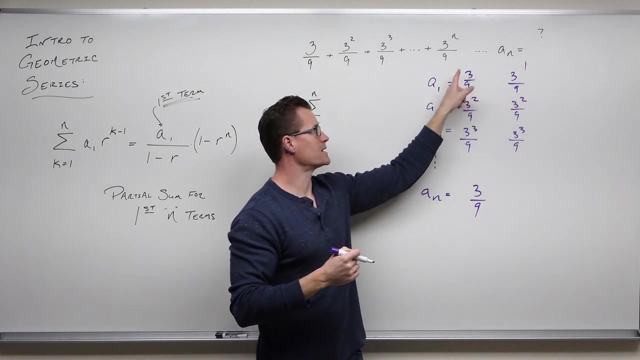 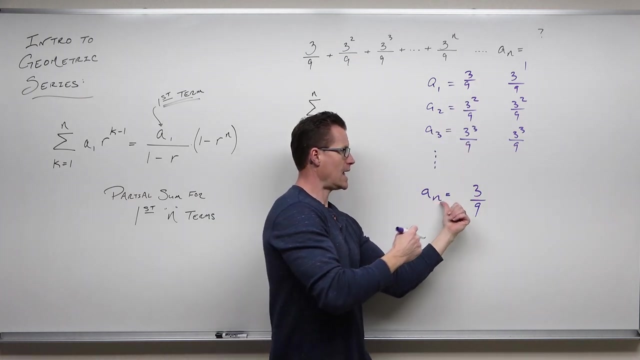 changing is going to end up in your formula and relate what is changing to your index. So what's not changing? 9 is not changing And our whatever is changing, our exponent here. our exponent is exactly what our index is every time, So 3, 3, 2, 2, 1, 1, n, n, But that's exactly what they're. 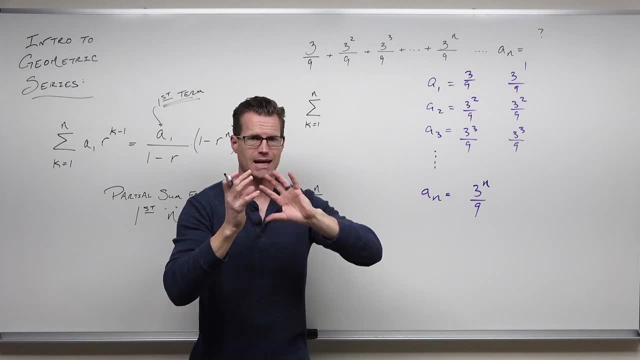 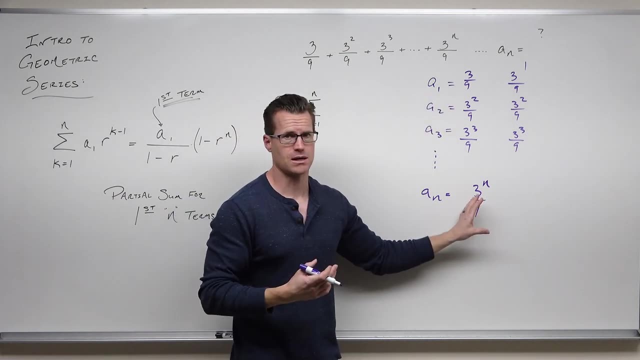 telling you there. So if they give you your sequence or your series and it ends with the nth term- that nth term is your geometric sequence- It's telling you that And you'd get exactly the same thing. It's very convenient. And so when we do this, we say hey. 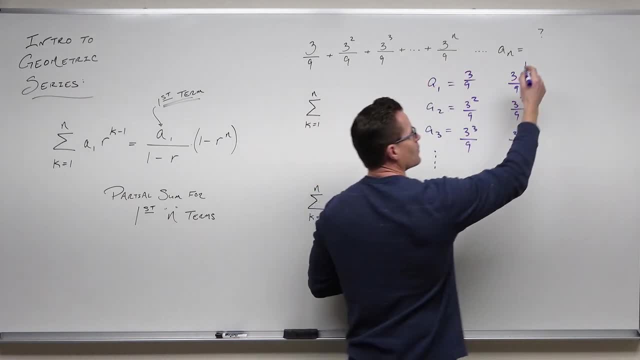 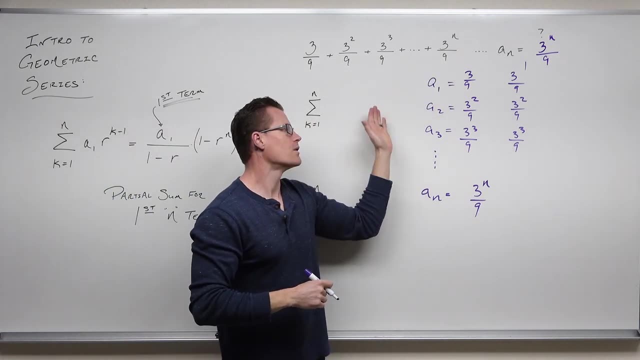 what's our, what's our, what's our formula for the sequence on which a series is built? Well, it's just your nth term, if it's in terms of n. Now, if they didn't give this to you, then, yeah, you'd have to go through and do exactly what I've shown you. But I've shown. 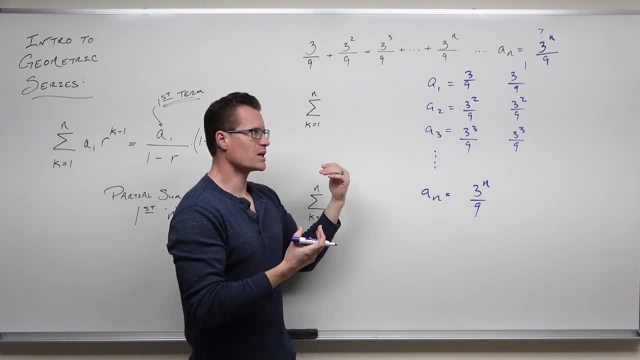 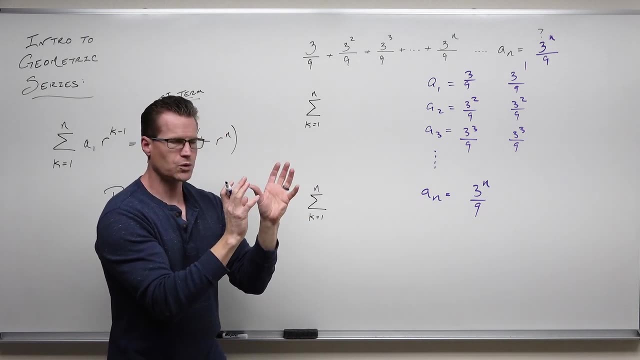 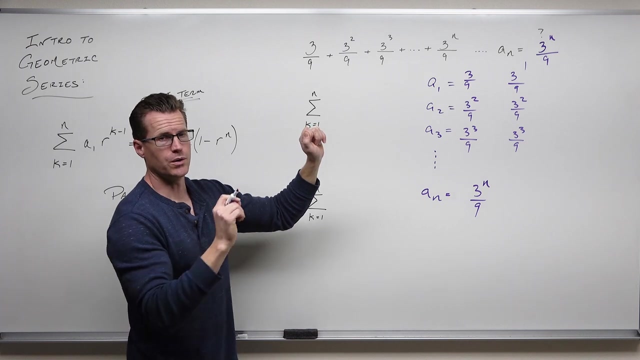 you that already It's, it's, it's the same thing that we've been doing as far as our series are concerned. So we're going to take that, We're going to write it with the appropriate index. Crucial nuance step is that if our sequence is the nth term is 3 to the n over 9, notice number: 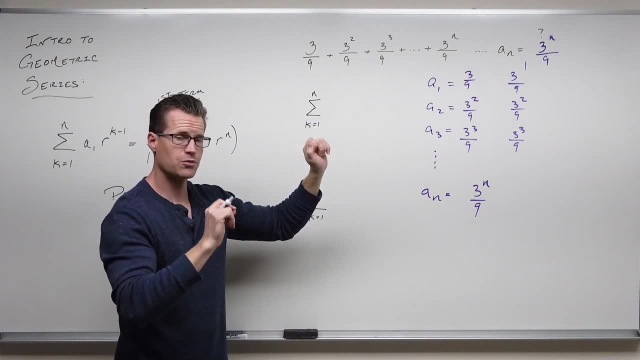 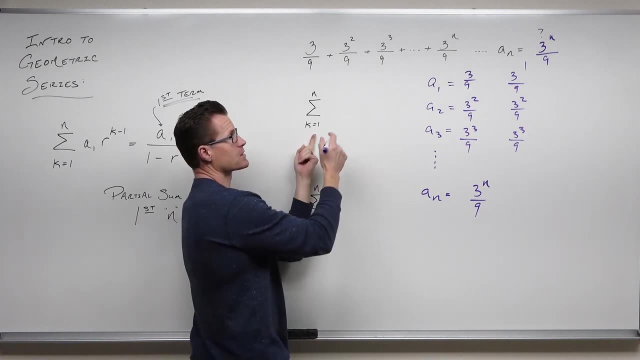 number 1, the 9 is not being raised to nth term, It's just 3 to the nth over 9.. Then if that's to the nth term, remember that we have to match whatever this says. So we need to say this: 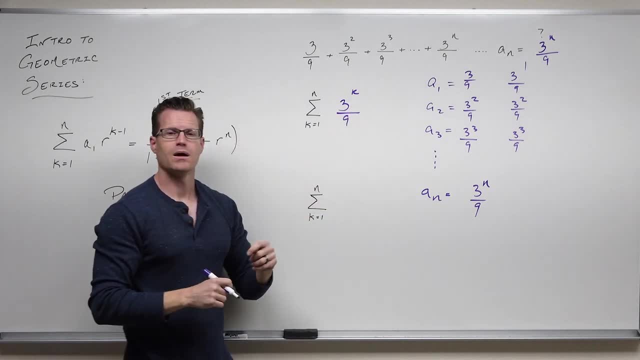 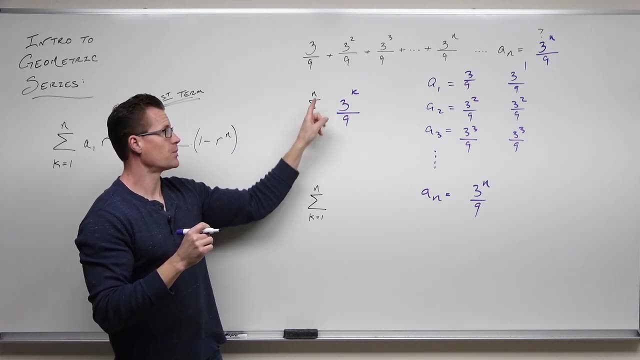 sequence is 3 to the k over 9.. Why? why that? Because you'd start at 1.. Now imagine this: plug in 1. You're going to get 3 to the 1st over 9.. That's that Plug in 2, 3 to the 2nd over 9.. 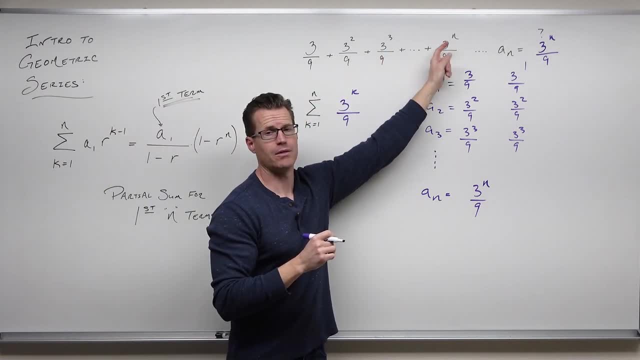 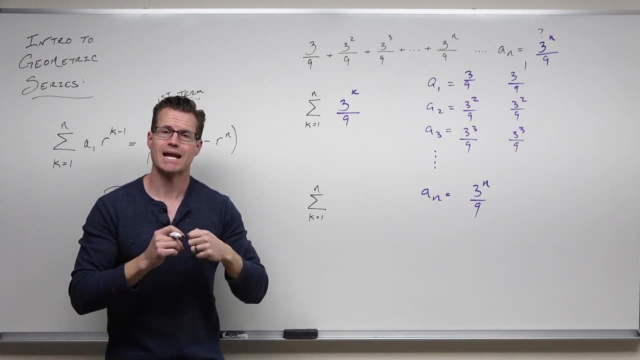 That's that Plug in n 3 to the 9,, 3 to the nth over 9.. That's why we have this as a different variable or index, so that we're allowed to plug in something different to it And we can end with. 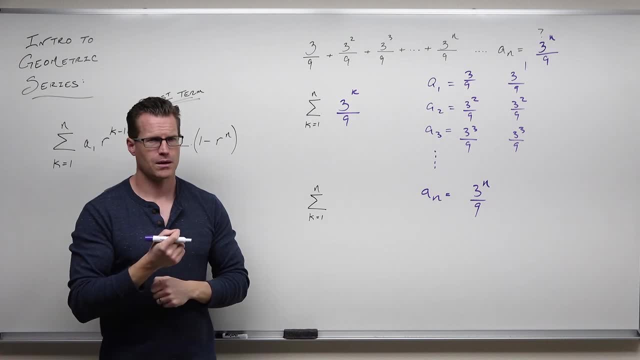 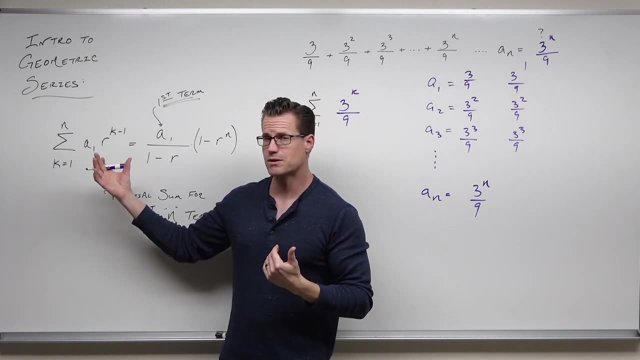 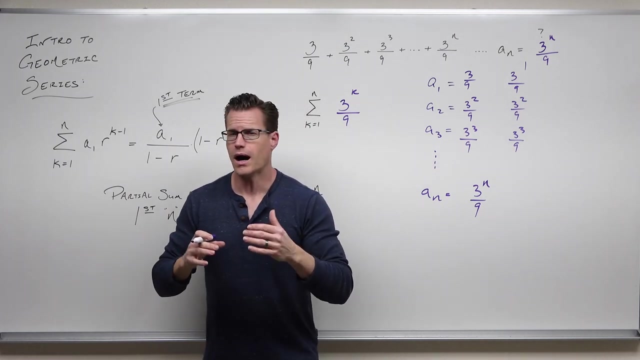 that nth term. Now, if you're thinking of that, this looks different than that It does. It looks a little bit different than how a geometric sequence normally does. It's not what we're used to. I really need this to make sense to you. I said that this is the first term and not necessarily. 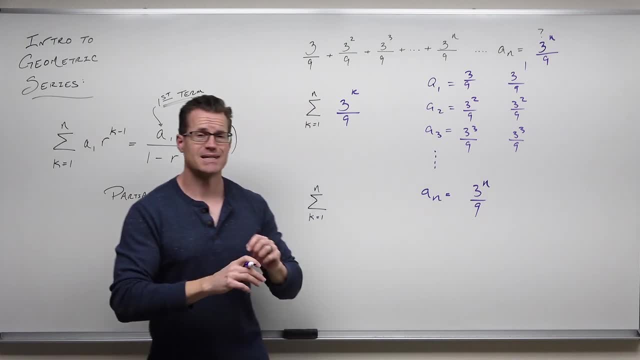 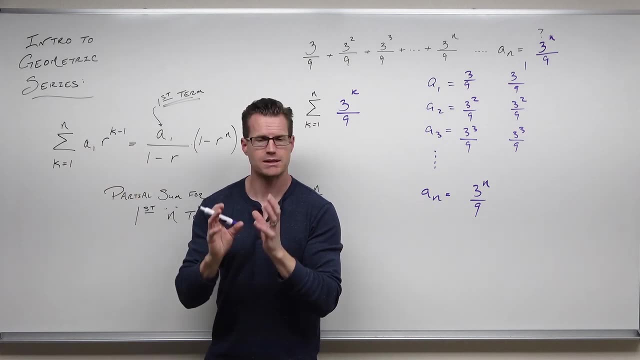 just a sub 1 for a reason, And here's the reason. It does not matter at all if this looks exactly like this. This makes it easier a little bit, but it doesn't matter. All you have to be able to do. 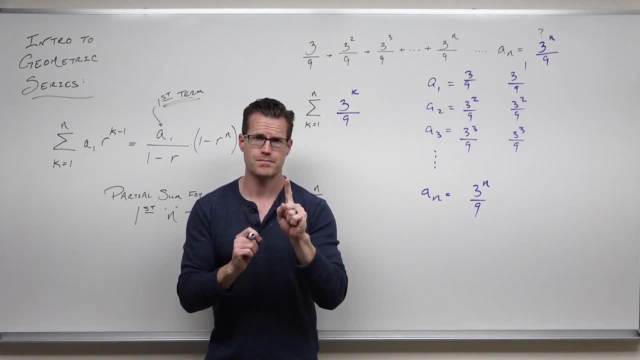 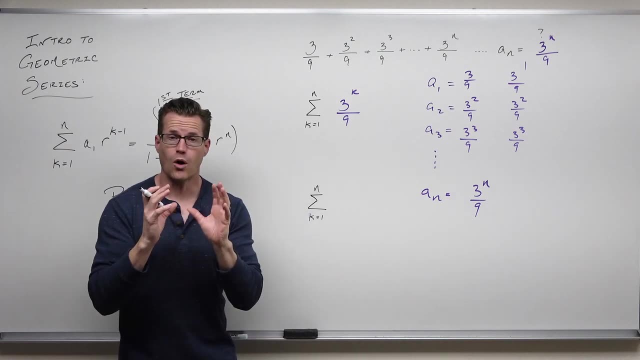 promise is the case is: identify your first term and identify your common ratio. So let's start with the first term. How would you identify the first term? The first term is 1. It's always identifiable by taking this and plugging it in, So even though it doesn't look. 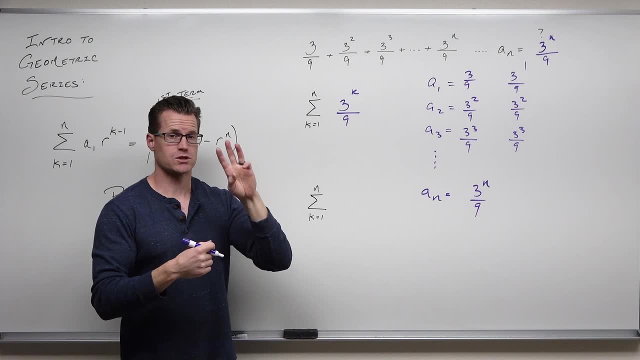 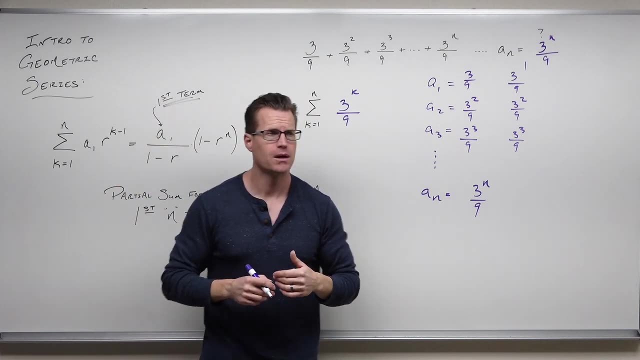 like that: take 1, plug it in here. 3 to the 1st is 3 over 9 is 3- 9ths. That's exactly what we have here And that's exactly how you can fill out this partial sum, which is kind of nice Now. 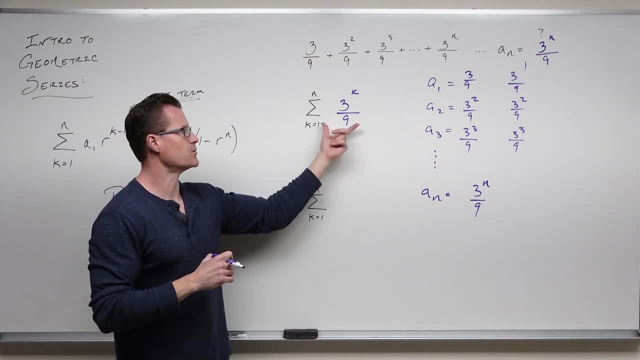 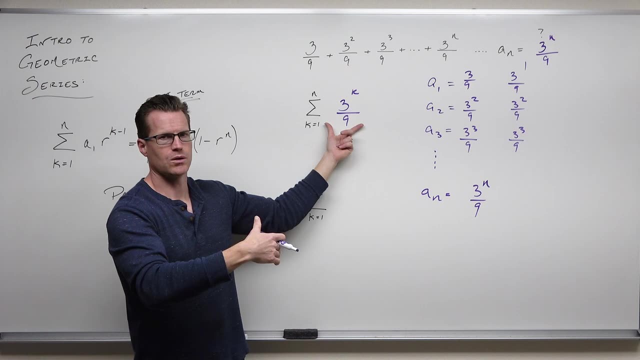 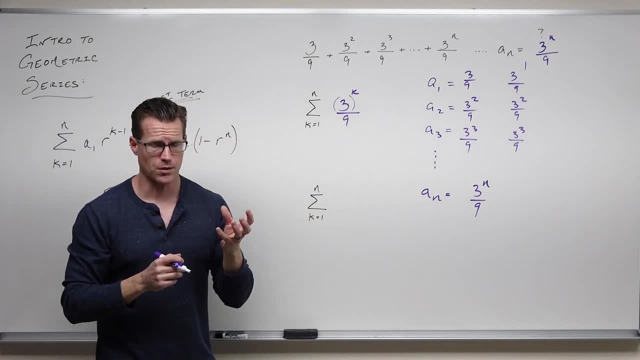 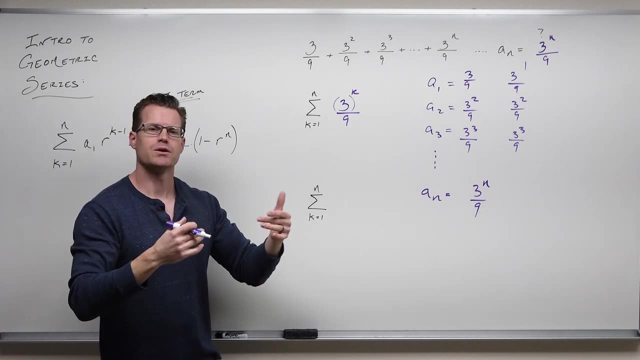 inside of the thing being raised to the power. Well, it's 3.. 3 is your common ratio. So your first term is 3- 9ths. You can find it by plugging it in 1 every single time. Your common ratio is: 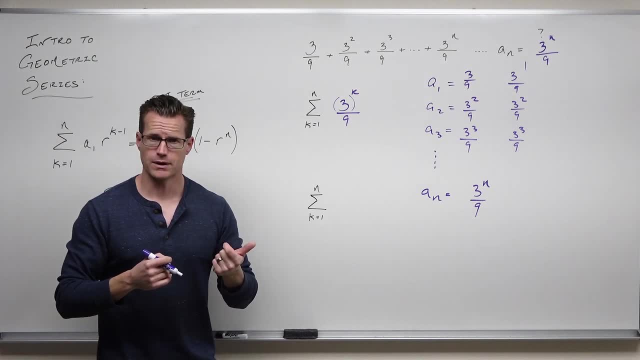 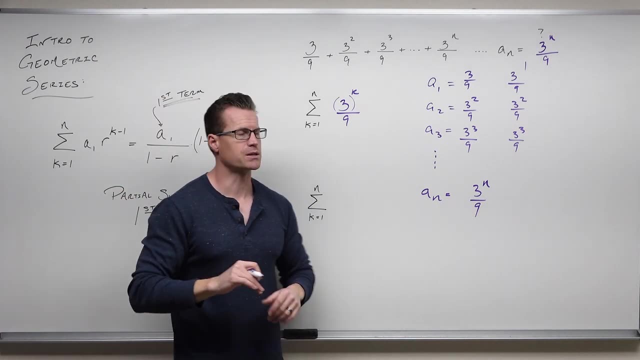 3.. Now could you write it differently? Yes, and that's why I have a different example here. So here's what you would do if you really needed to match up. First thing is you'd strip off that 1- 9th. that's in there. 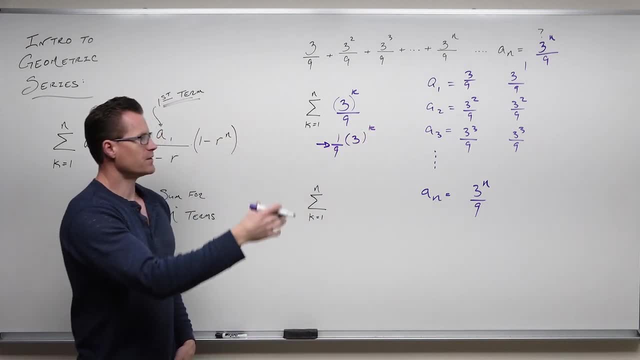 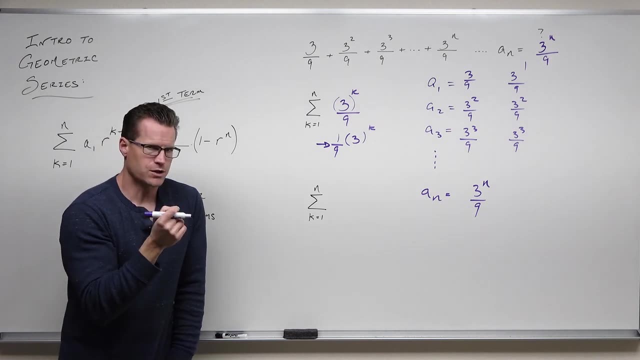 So that would give you 1 9th times 3 to the k, Because 9 is not being raised to the k power. that's perfectly appropriate to do. The other issue, though, is that that says k minus 1, and that one doesn't, So what are you going to do? Well, if that doesn't say: 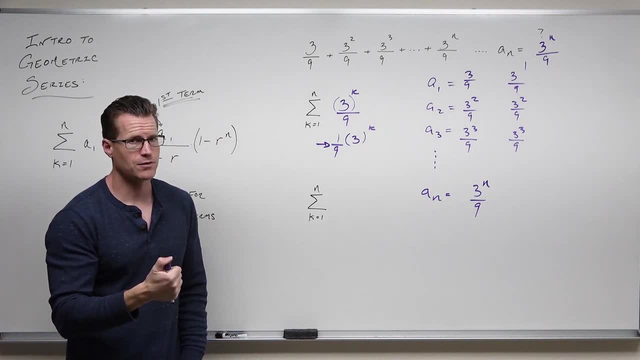 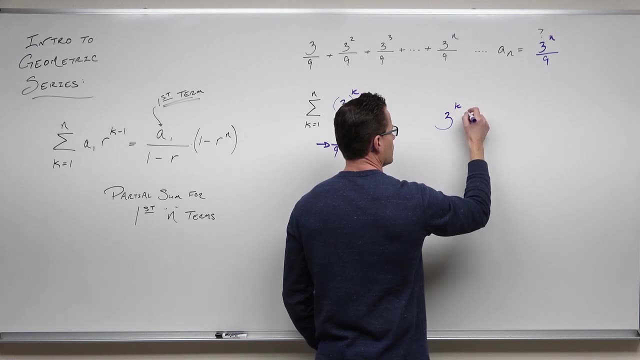 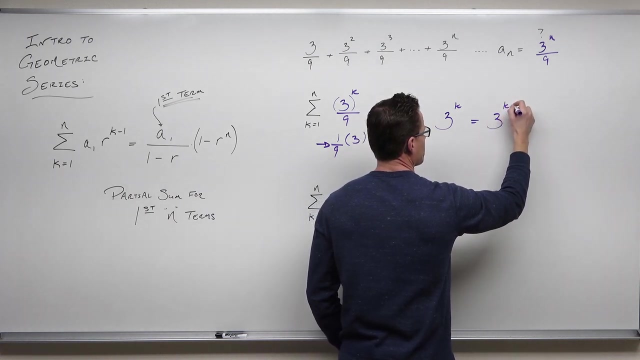 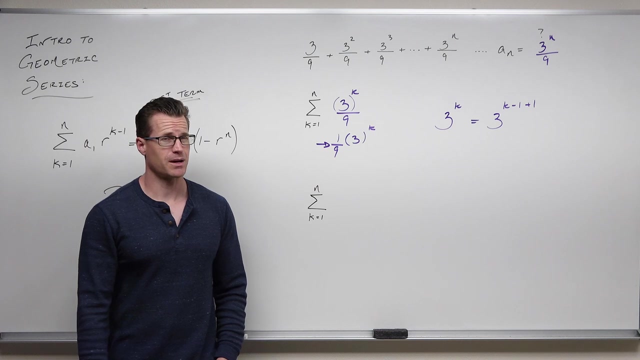 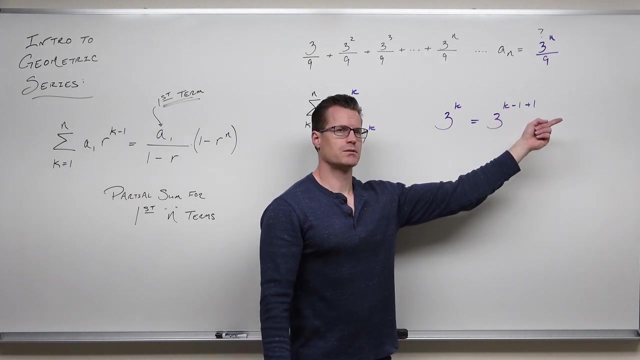 k minus 1,. you can change it, but you have to really think outside the box here. I know that looks funny, but I want you to really think about it. Is it true? Is it true that 3 to the k is the same thing as 3 to the k minus 1 plus 1? Well, k minus 1 plus 1 would just give you k. 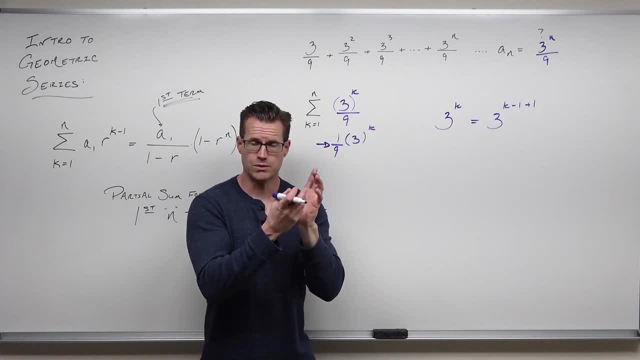 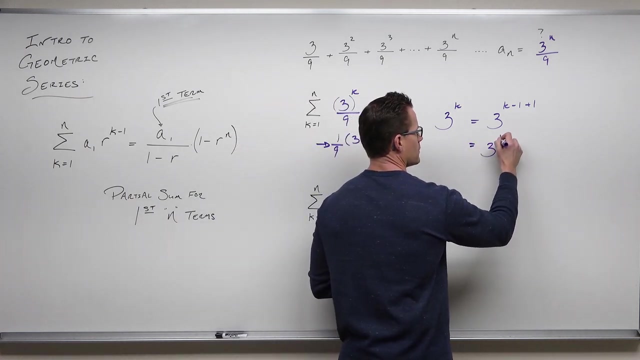 so again, it's true, This is the way that you reduce a power. So you write this as minus 1, plus 1 and think: how do you connect addition of exponents? Well, that has to happen via some sort of multiplication. So the only way exponents are. 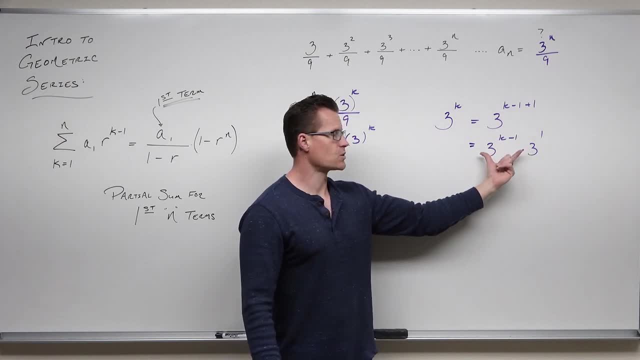 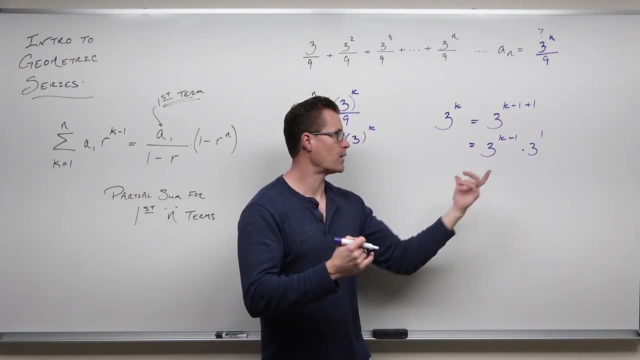 added is if they came from k in common. This is being multiplied, So think backwards on this. 3 to the k minus 1 times 3 to the first, You would add k minus 1 plus 1. That would give you k minus. 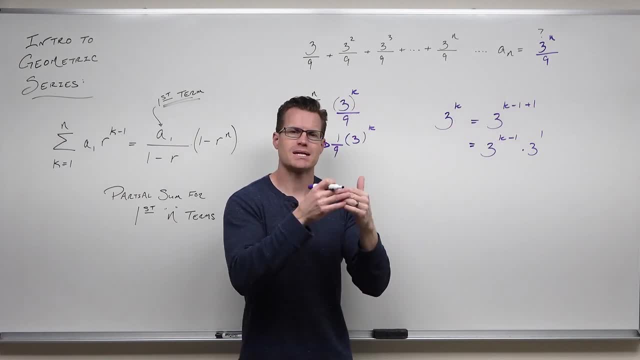 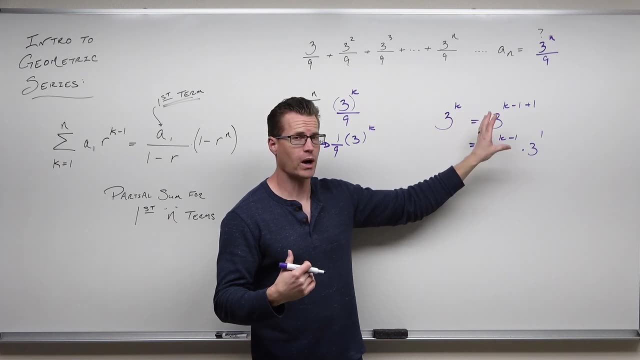 1 plus 1.. This would give you k. This is the same, but it's taken and stripped off of power And you can always do that. It's not as hard as what I've explained it to you. This is explaining why it. 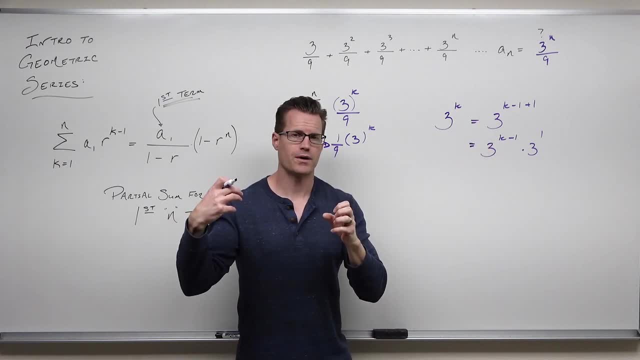 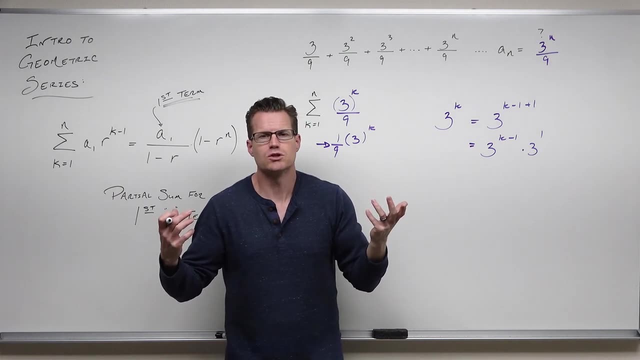 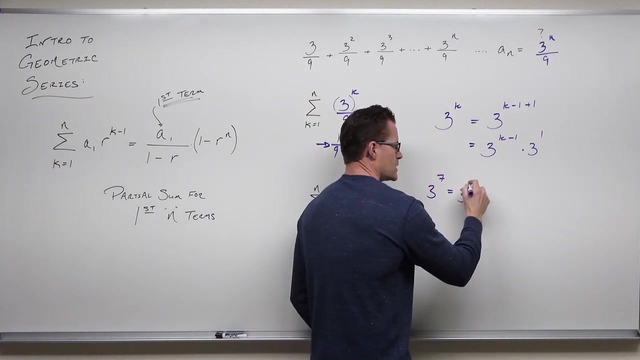 works, But it's really not that bad to strip off one factor from any sort of exponent and reduce the exponent by one. We actually could do it all the time. Just think about it for a second: If you had 3 to the seventh, couldn't you write that as 3 to the sixth times 3 to the? 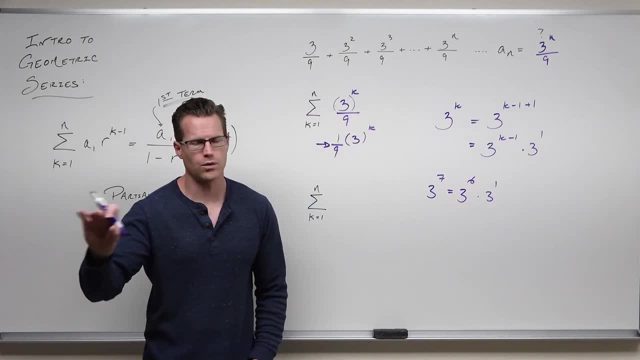 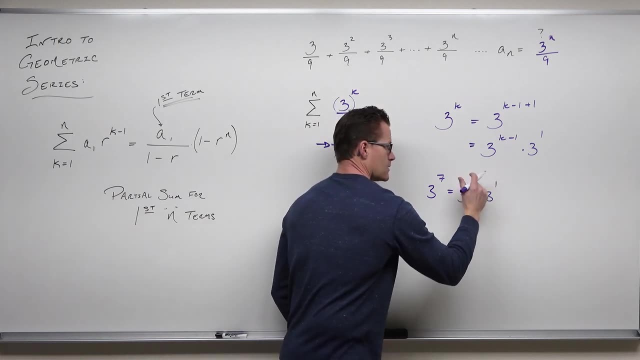 first: Yeah, we do it all the time. We do it when we factor all the time We just think, well, yeah, 7 is 6 plus 1, so it would be pretty easy. Well, isn't this 7 minus 1?? Yeah, that's exactly. 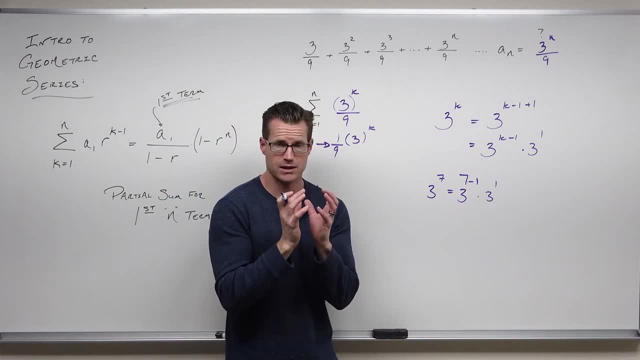 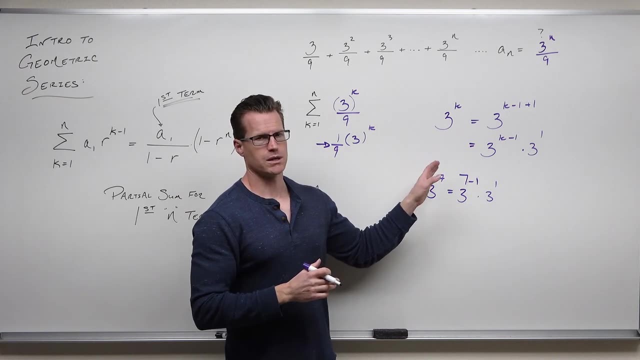 what that is. You're subtracting 1 from the x of the power, the exponent, and then you're using one of those powers to represent some sort of a constant. And that's exactly what we're doing here. So we can take this and say: hey, this right here, that 3 to the k. 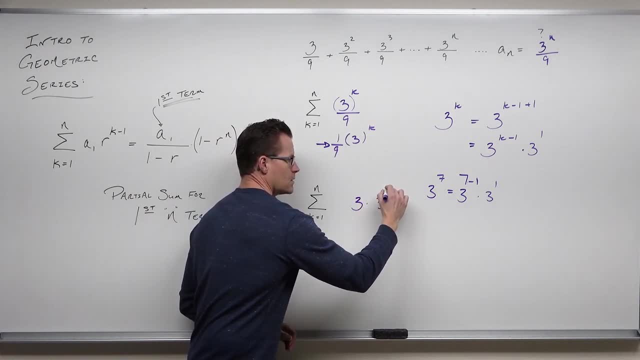 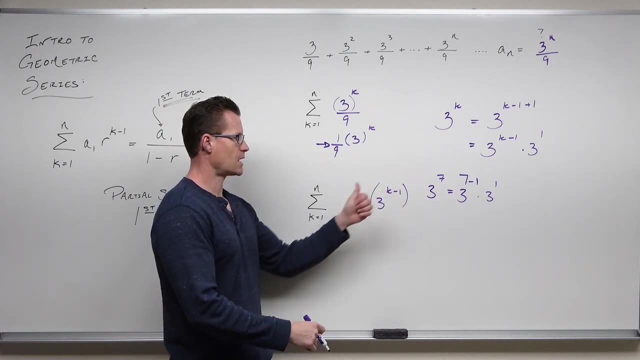 you could write it as 3 times 3 to the k minus 1.. That's exactly what we've done here: 3 to the first times 3 to the k minus 1.. If we put that one ninth back, so one ninth here. 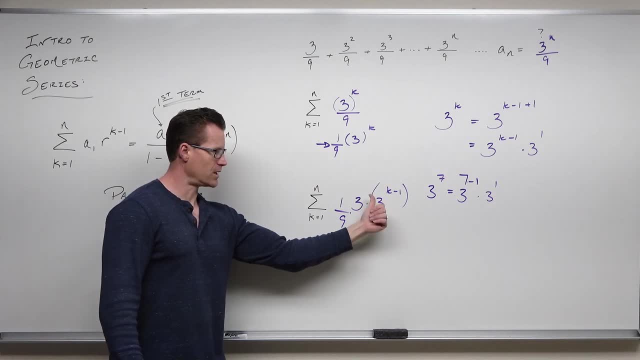 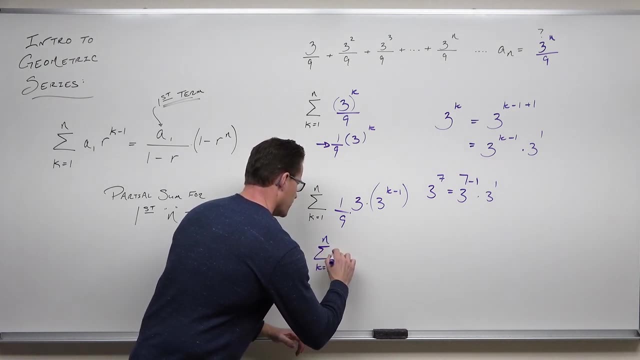 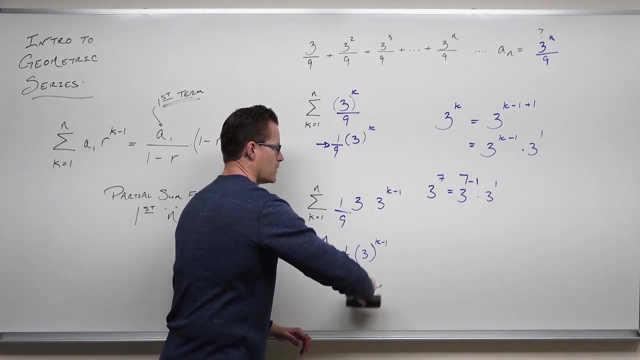 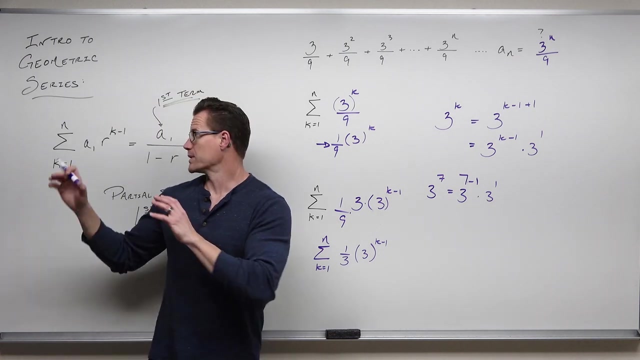 this is written as 3 times 3 to the k minus 1.. And if you simplify that, yeah, these really should be written a little bit better- I'm going to do this There. that's better. That matches what we have here. This is if you take a look at it. 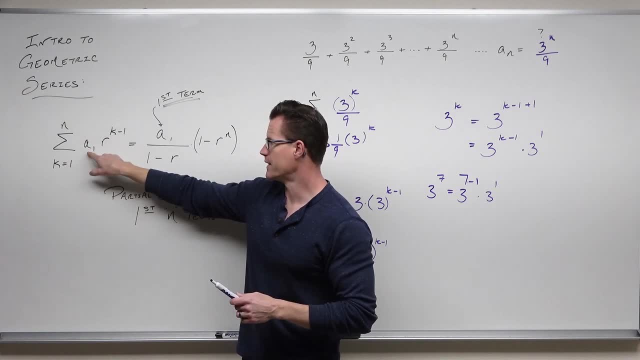 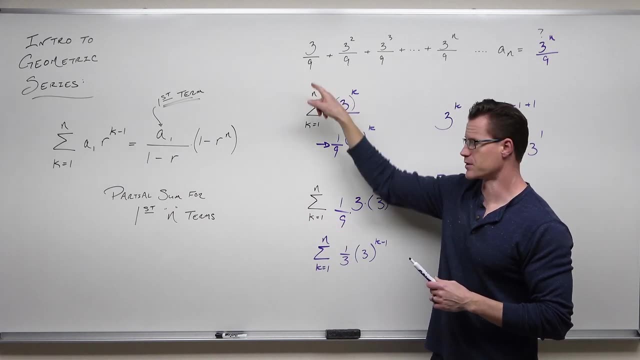 if you match it perfectly to this, where you start at 1, that's a sub 1, that's your common ratio to an exponent. It says: this should be your first term. Well, it is 3. ninths is one third. This should be your common. 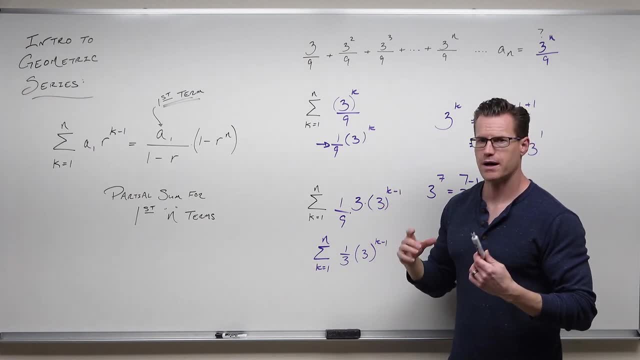 ratio. It is, It's 3.. Now could you find the same thing by just plugging in 1?? Yes, I've said that to you. If you plug in 1,, 3 to the first is 3 over 9, that is one third. 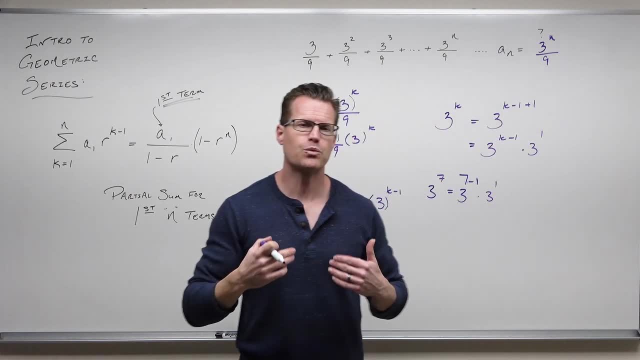 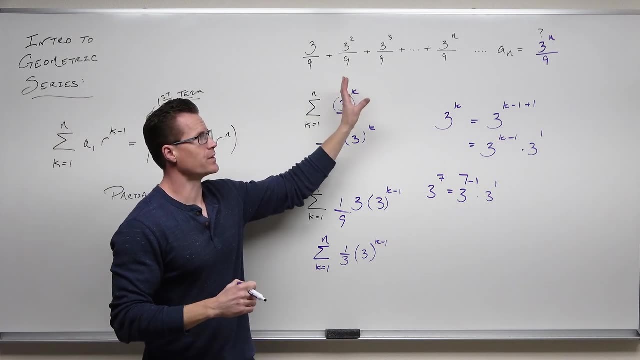 This is your common ratio of 3.. Now, which way is better, It doesn't really matter as far as finding the sum. So what we've done so far is we've identified what a geometric series is. We've gone through an example showing that if they give you an nth term, you can find your series. 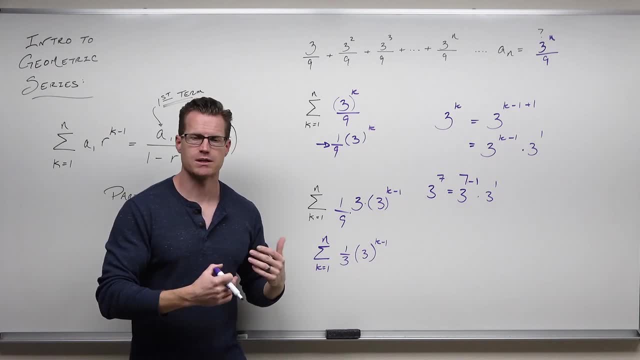 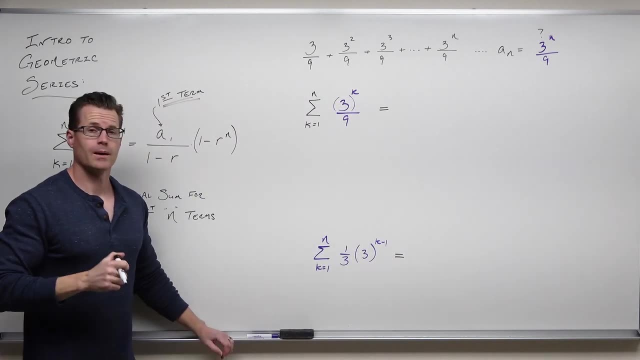 very easily. And now we're going to find the sum of the three. So we're going to find the sum of the series I'm going to show you. It gives you the same thing, no matter which of these you actually write. So let's give it a try. Here's what a geometric series adds up to in a partial sum. 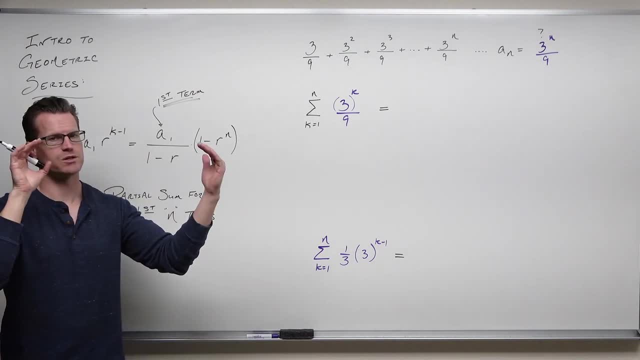 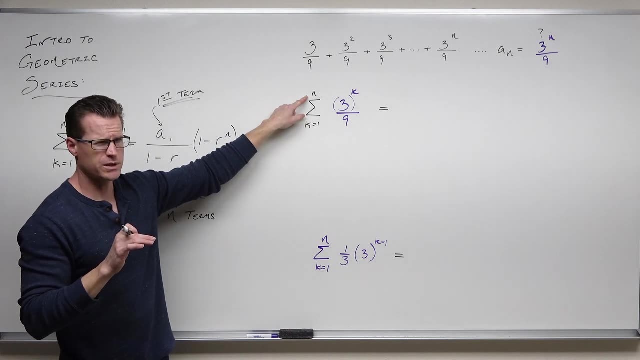 Again, partial means you're not going to infinity, And so you consider this to be up to a certain point. Now we're going to go from the first term all the way to the nth term. Well, what does that mean? You just leave the n, That's okay, And here's what this says. 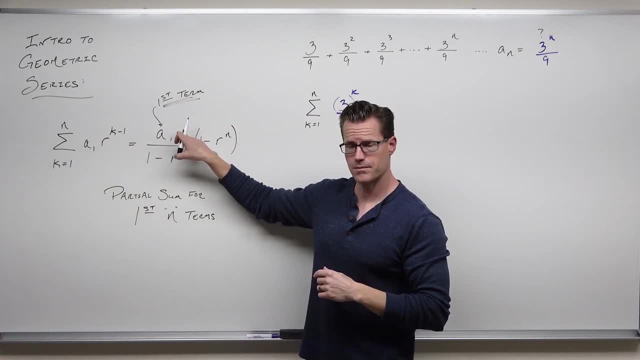 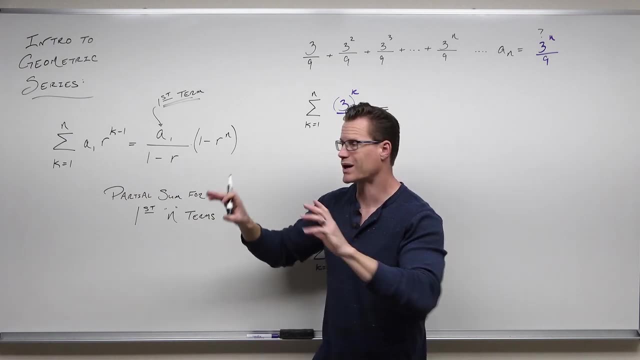 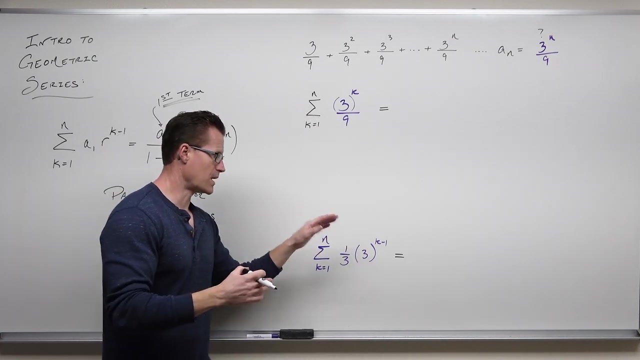 Find your first term, divide by 1 minus your common ratio, and then multiply 1 minus your common ratio to the nth power, whatever that power is. So let's identify the first term This way. it's pretty easy, because it matches up perfectly. Okay, your first term. 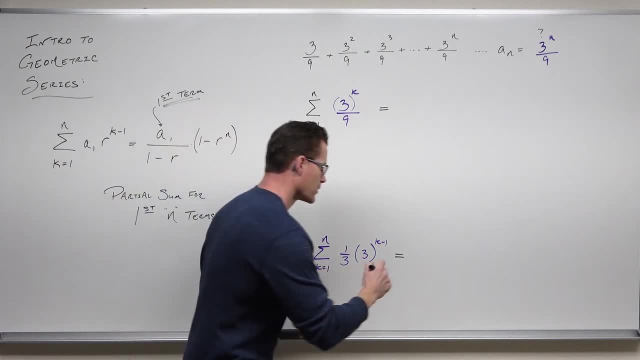 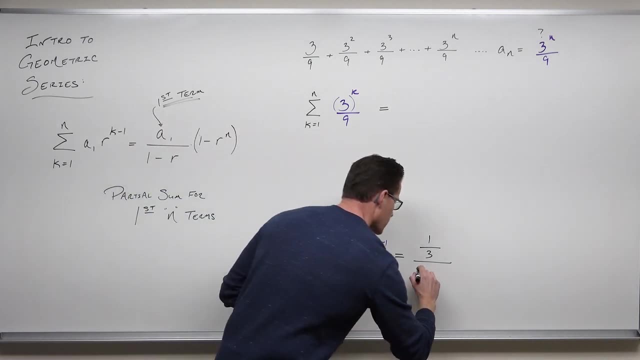 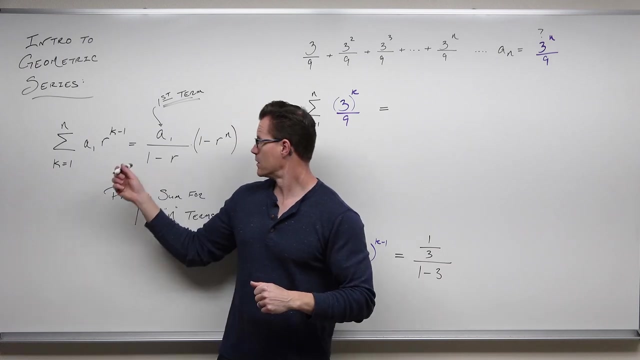 it fits the model perfectly. Your first term is 1 third divided by you. take 1 minus your common ratio, That's 1 minus 3.. So we have first term 1 third here, 1 minus common ratio, 1 minus 3,. 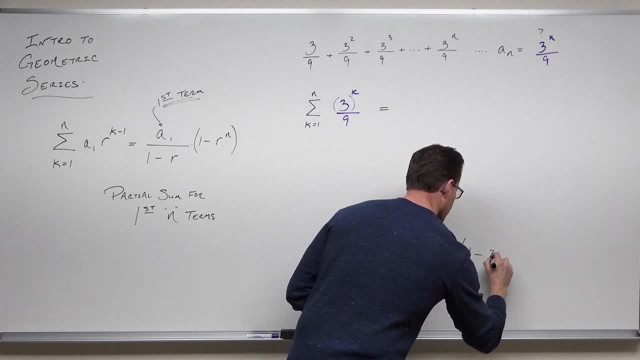 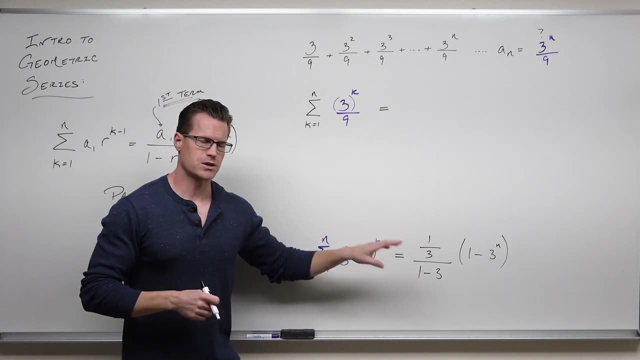 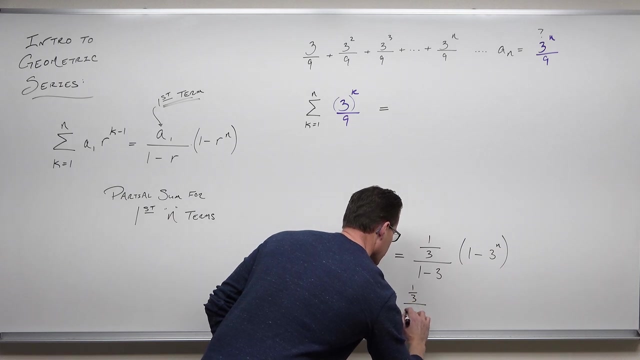 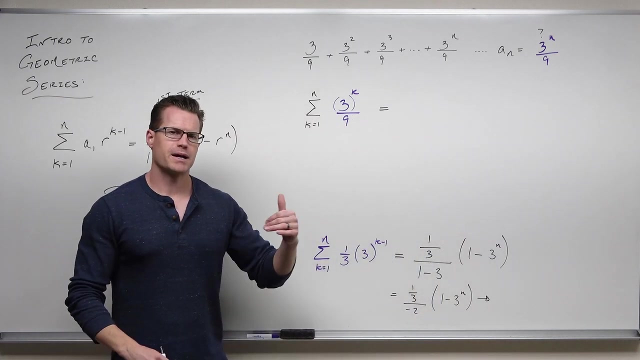 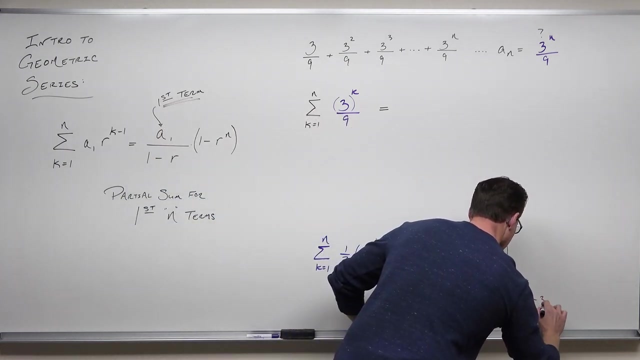 times 1 minus 3 to the n. This needs to be simplified So you don't leave it 1 third over 1 minus 3.. Just take a little bit of time and simplify that. So 1 third divided by negative 2 is negative 1. sixth times 1 minus 3 to the n. There's not. 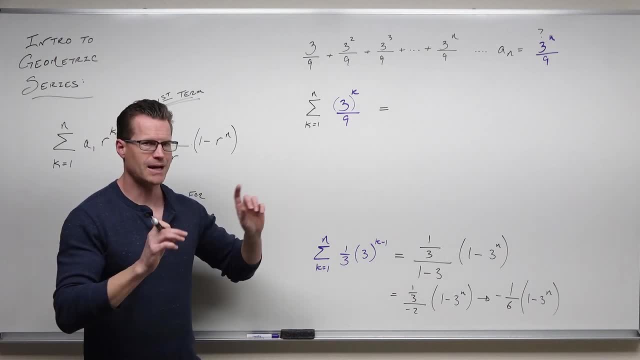 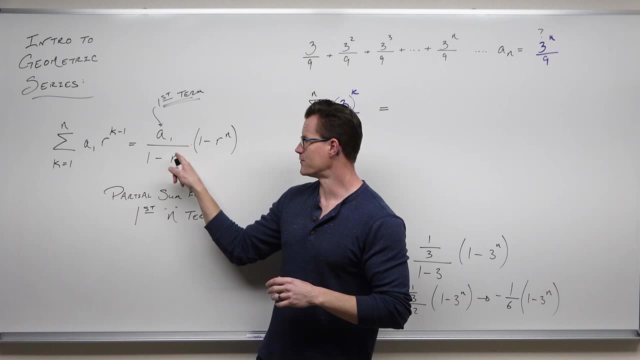 much you can do to simplify that. Let's see if we get the same thing here. Now remember, even though this is not fitting this model, all this means is find your first term and find your common ratio. Let's find the first term. How do you find the first term? Well, you find the first. 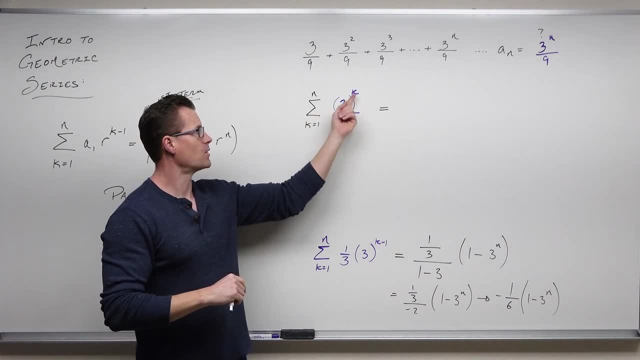 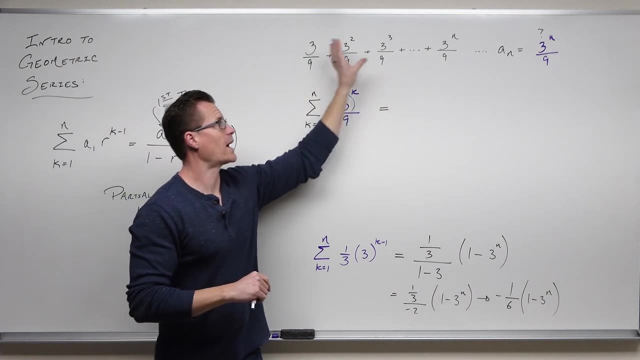 term is just plug in that number. If I plug in this number, will our first term be 3 to the first over 9?? Why I'm not going back to here is what if you're given this without this? What if you don't? 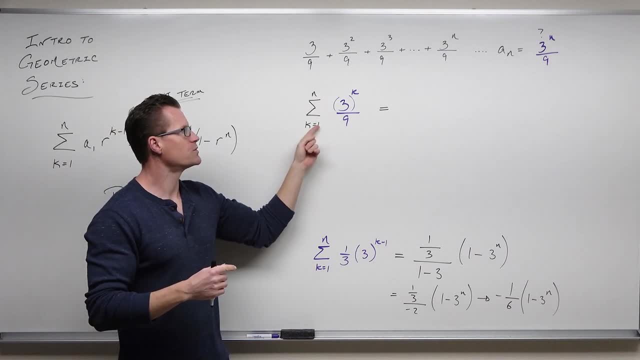 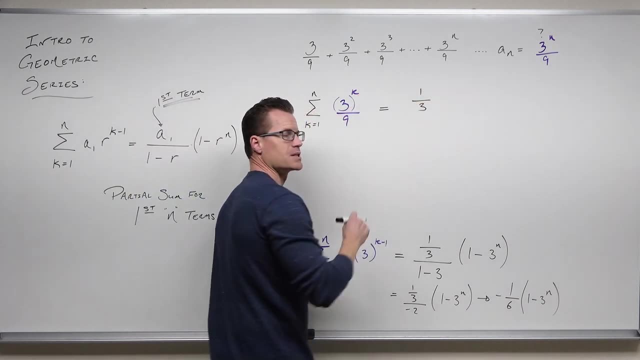 have that And you can't just say yeah. first term is 1. third: Plug in the value. So plug in 1, 3 to the first. is 3 over 9 is 1 third. Notice it's giving you the same thing. Identify what's. 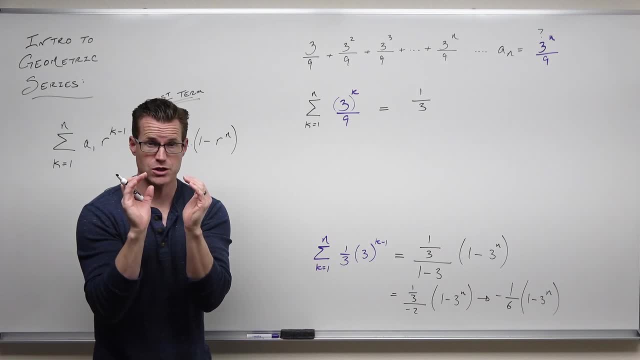 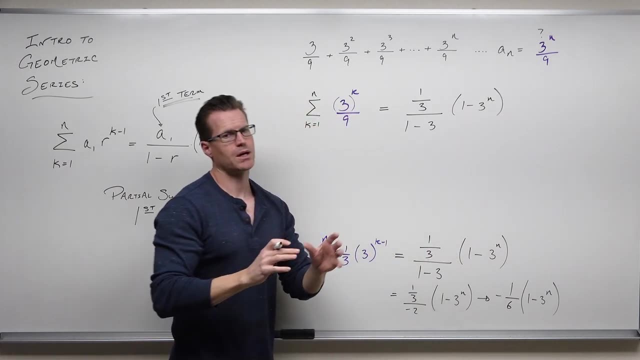 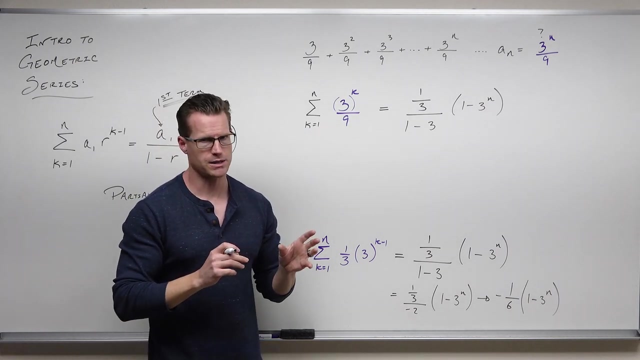 on the inside of your parentheses being raised to the power. That is your common ratio. So our common ratio is 3.. And if you simply understand that this really does stand for the first term and you can find it by just plugging in that value, it's going to save you a lot of time here and a lot of time in. 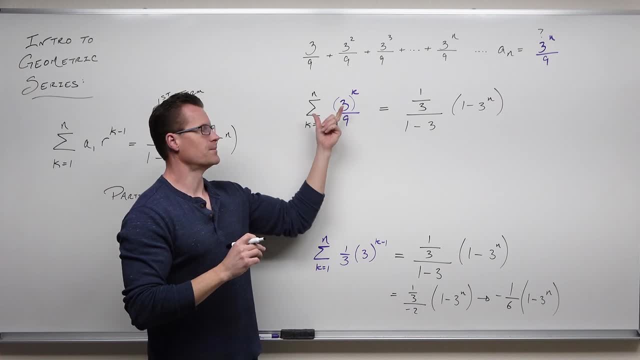 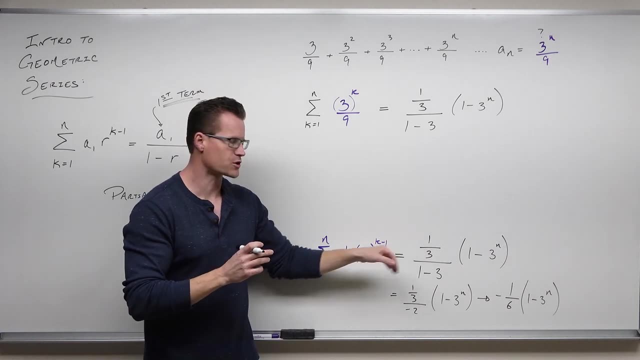 Captains 2. Because a lot of times we have to. if you don't realize that, you have to manipulate a lot of junk to get it to fit the exact model just to find out what the first term is when. it's very simple: You just plug that in, It's going to tell you your first term and you put it on your new. 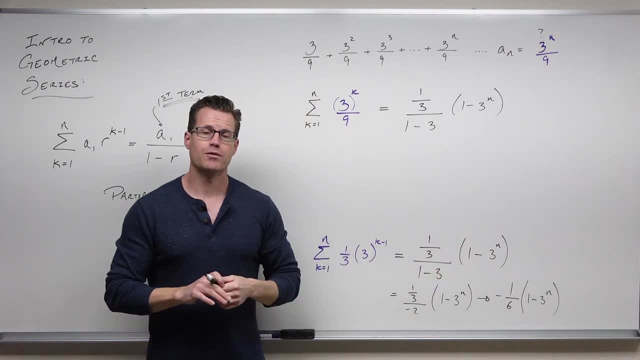 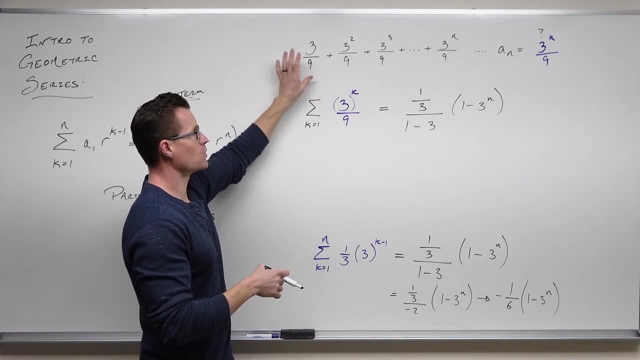 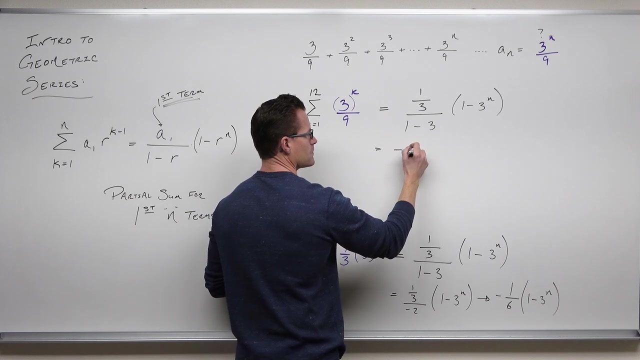 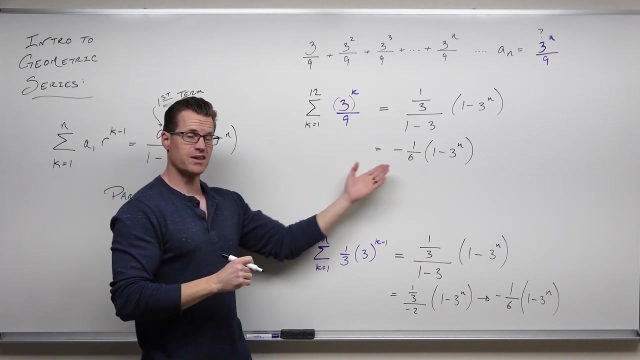 numerator. It's plain and simple. You can see it's exactly the same. Now this is adding up to a partial sum of the first n terms. What if we just wanted to add the first 12 terms? Well, what would you do? In either case, if you're going to a finite number of terms, this will add it. This says if: 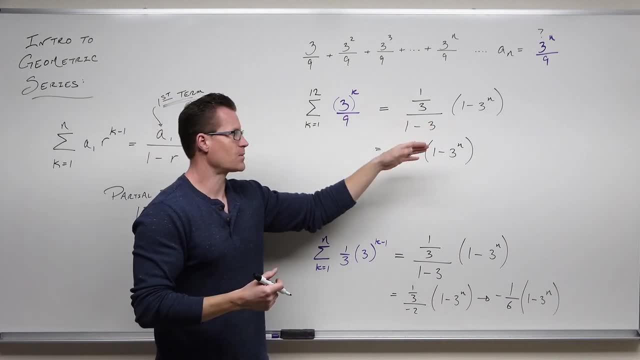 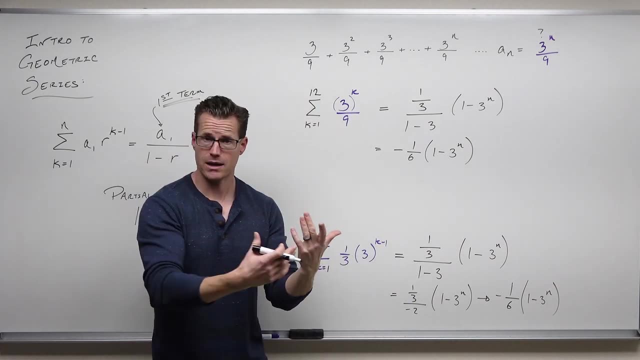 you're going to the 12th term, then you're going to do exactly the same thing. Your first term here: 1 minus your common ratio, that's what that says. And then 1 minus your common ratio to whatever your n is. In our case, we change this to negative. 1. sixth: 1 minus the 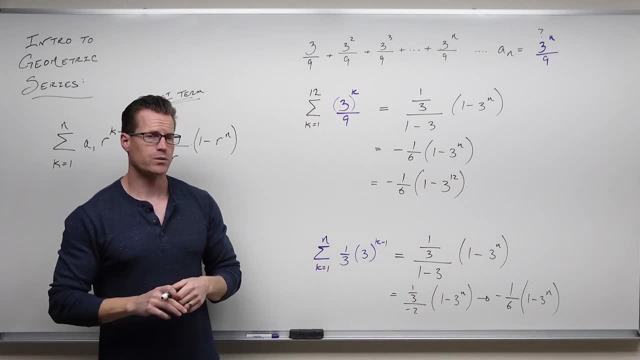 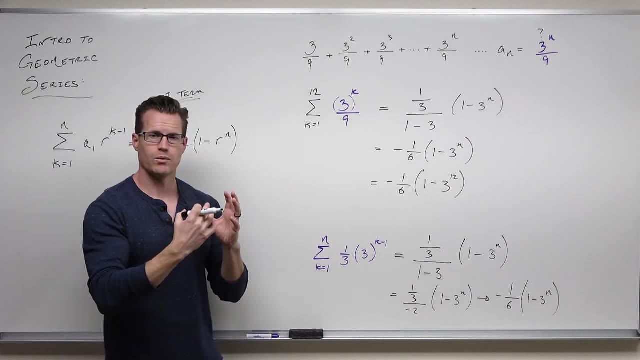 common ratio to the 12th power. That's all there would be to it. 3 to the 12th is fairly large, so I really don't want to do that. But you take 1 minus 3 to the 12th and then multiply whatever. 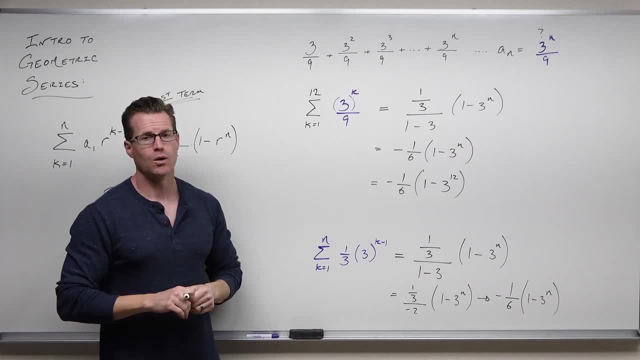 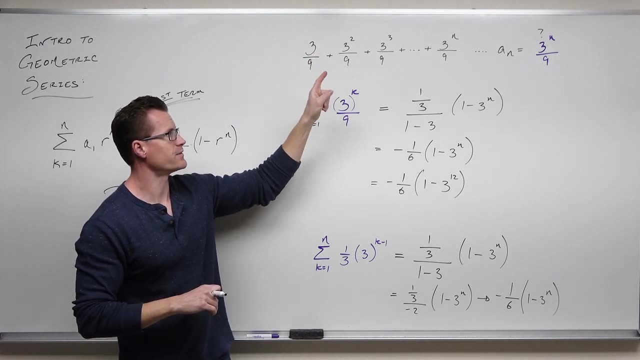 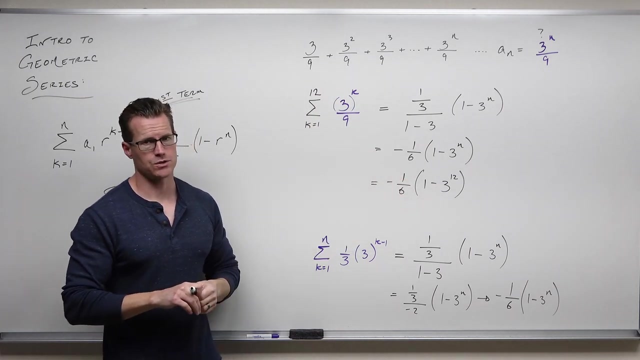 that is, times negative 1 sixth, It will give you whatever these terms add up to. That's pretty fascinating. So if you took 1 third and 9 ninths and 27 ninths and all of those things and added those fractions up for the first 12 terms, you're going to get exactly what this tells you. 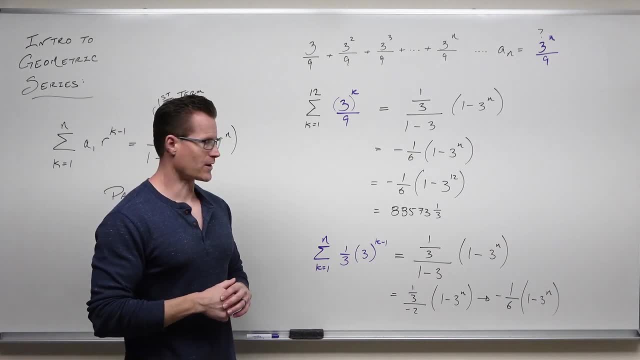 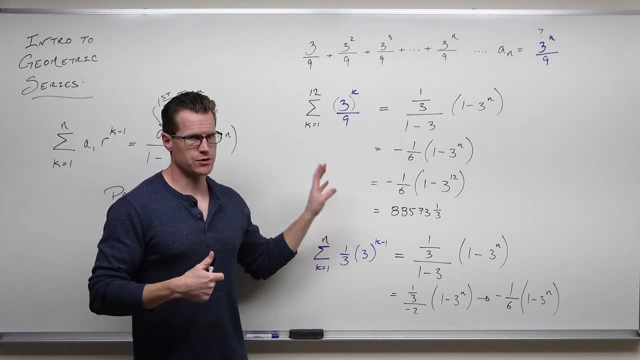 I ended up getting 88,573 and 1 third. I just couldn't leave it alone. I had to figure out what that was, So I hope that, admittedly, makes sense. I really hope that you're seeing that these two things are equivalent- I've shown that to you- and that you are ultimately going to get the same sum. 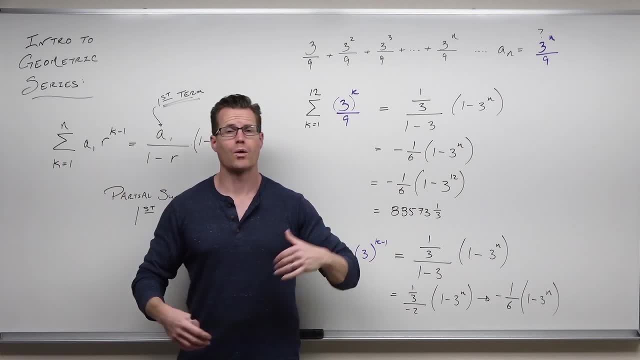 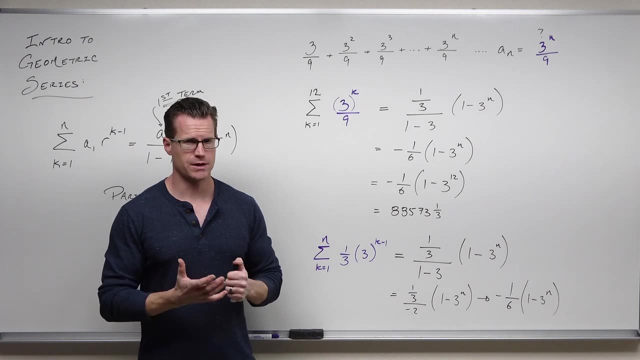 whether you write it in the same exact format or not, just realizing that all that's really asking for you is the first term. What we're going to do now is we're going to come back. We're going to talk about infinite series, These 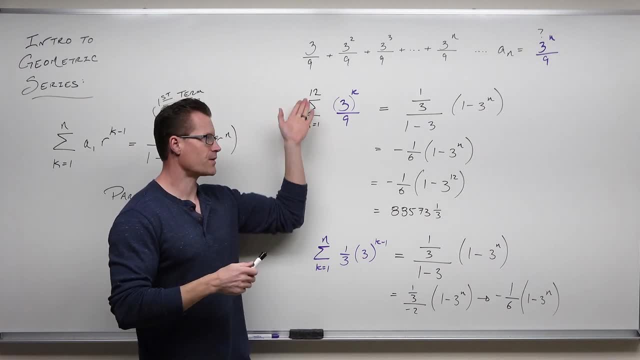 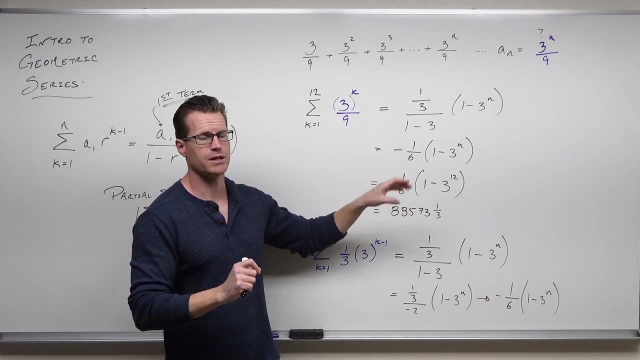 were partial. This was going up to a finite number. I could have stopped at 5.. I could have gone to 50.. It's in the same way. You're just plugging in whatever your excellent is. It's very nice because it's only in one spot. That's very convenient. So we'll come back and talk. 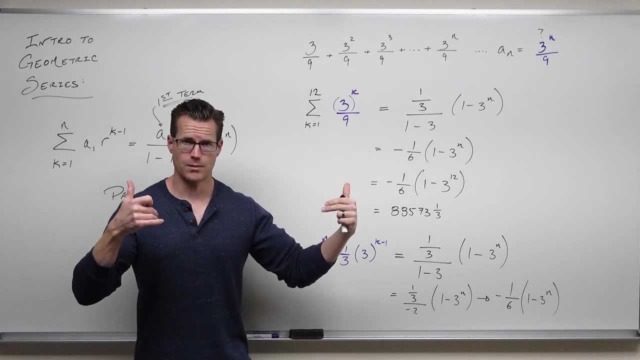 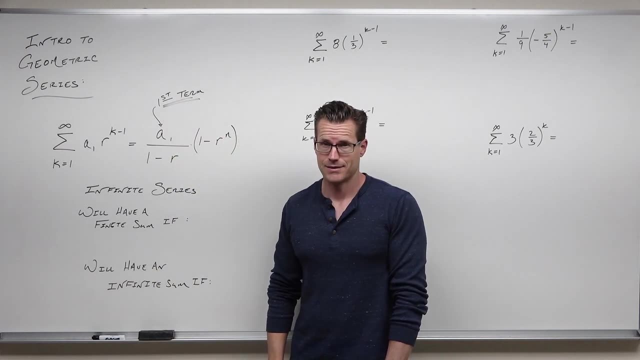 about when a geometric series will add up to a finite number with an infinite number of terms. Okay, here we go. Last little bit talking about infinite geometric series. What in the world those entail? What if I didn't stop and I just added up all the terms of this geometric series? 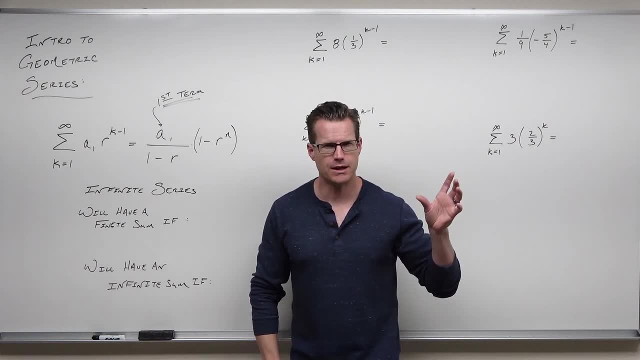 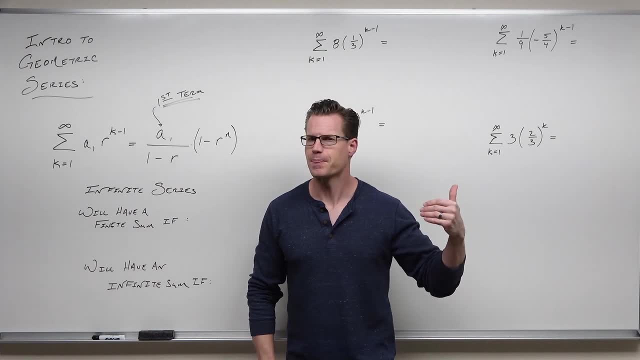 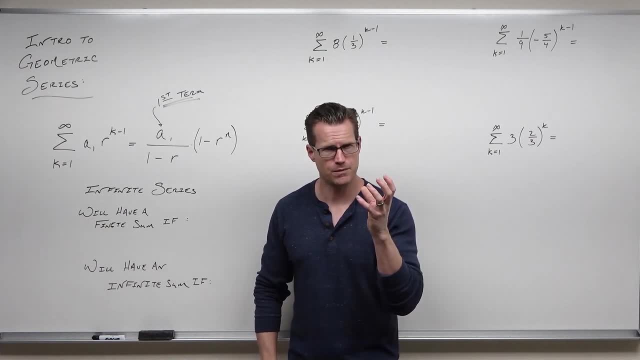 when a geometric series will what's called converge- add up to a finite number, or diverge- add up to either positive or negative infinity. It will be one of those two cases. That's the only two things that we can possibly have in the series: adding to a number or not. 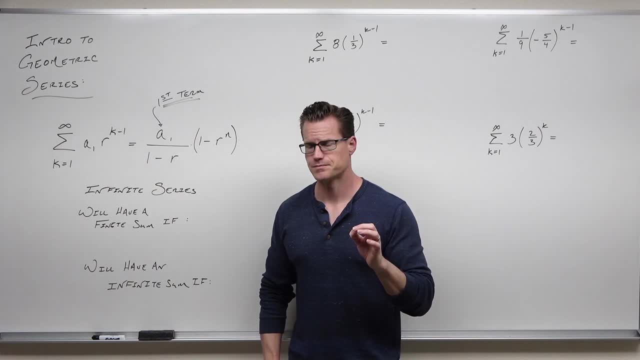 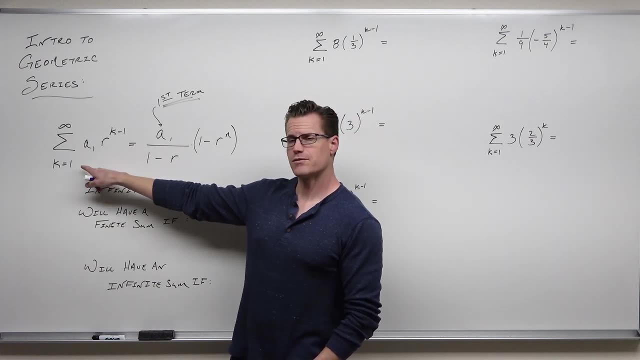 All right. well, let's figure out what in the world happens. I want you to look at the subtle changes I made between the last part of this video and this part, Instead of going from one and stopping at n. this is now an infinite series. I started the first. 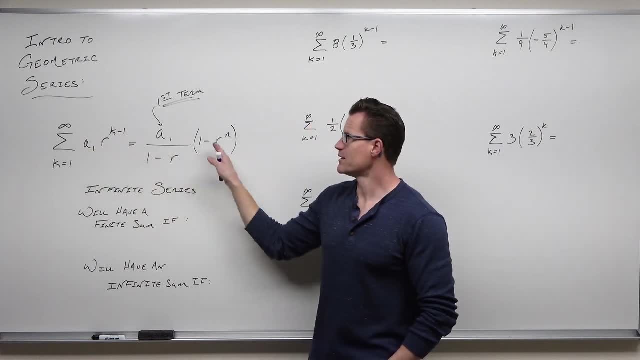 term, I don't n. that goes to infinity. Now we still have a sum. This is the sum of every single geometric series ever, and I know that if you see this in your textbook, that's not there. We're going to talk about why right now. So, on a partial sum, you have the ability to stop right, You have. 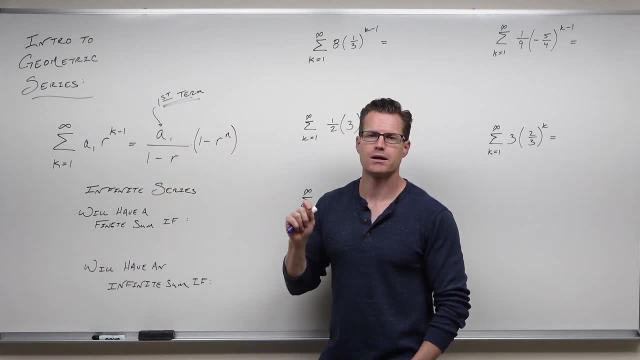 the ability to stop somewhere and say: all right, I can plug in a value here. Here's when you should know when this series is going to converge or diverge. I really need you to listen very carefully about this. Let's imagine that n goes to infinity. So we're starting to think. 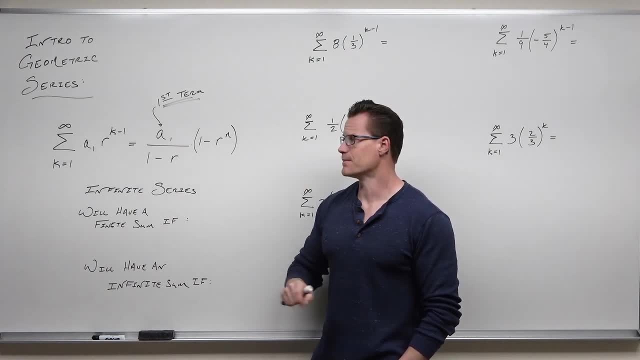 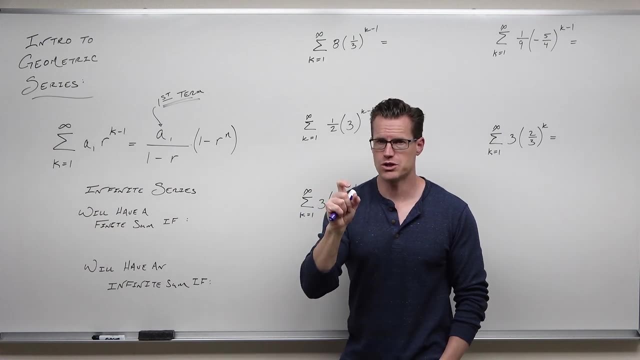 kind of a limit idea. What would happen if n goes to infinity? If I just don't n, what would that happen? Well, r your common ratio. this is key. your common ratio would be raised to a really, really, really big exponent: infinity. 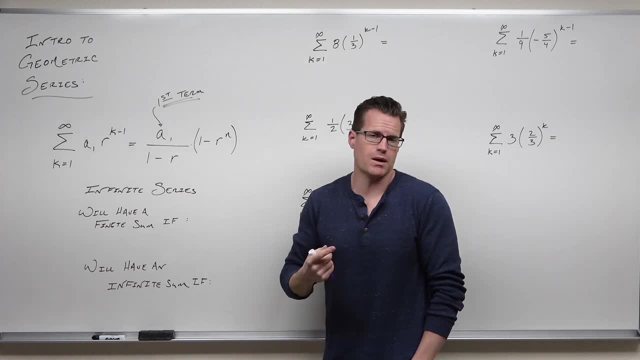 Is this always going to be infinity? Now, you might be thinking: well, man, if I take a constant common ratio and I just, you know, take the infinite power, it's just going to be really big, or maybe really negative, but it's just going to be really, really big, Is it, though? Let's think. 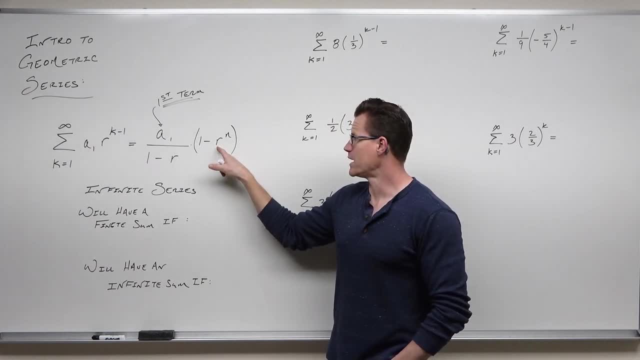 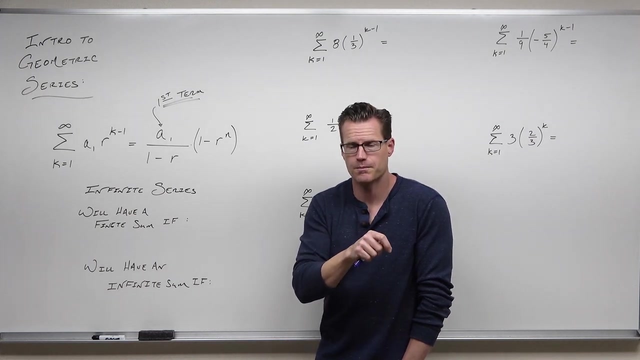 about this. What would happen if this value is- I don't know- two? Well then, two to the infinity would be infinity. But what would happen if that was one half? Think about the values of fractions when you start multiplying them. So one half times one half is one fourth. One half to the 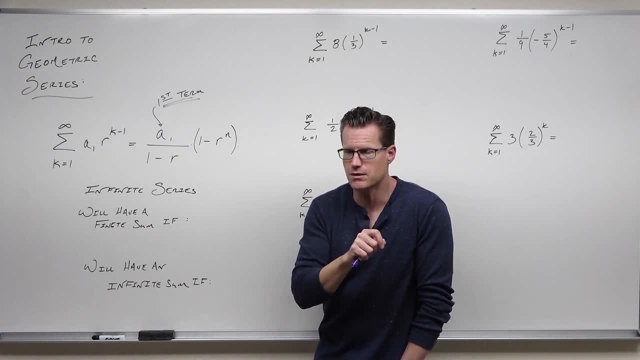 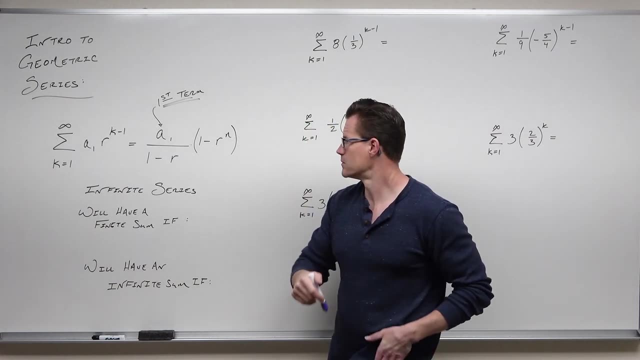 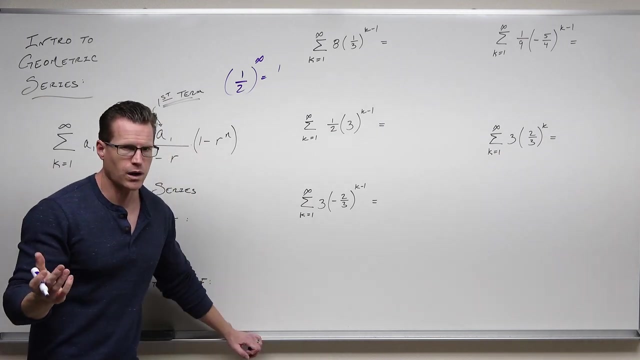 third power is one eighth. One half to the fourth power is one sixteenth. What would one half to the infinity power be? Well, that would be one. One to any power is one, But how about two? Two to the infinity power would be. 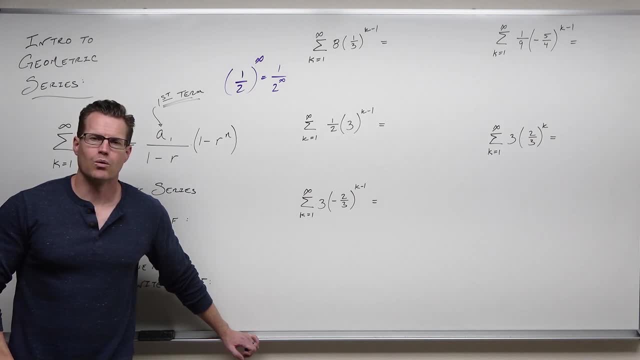 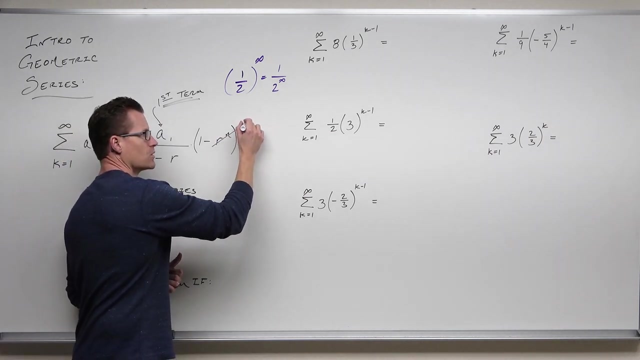 infinity. Now, this is the key. What would one divided by infinity be close to? Well, it would be close to zero. So wait a second. If I take certain values of common ratios, I take them to an infinite power. this part goes to zero, not infinity. What's one minus zero? 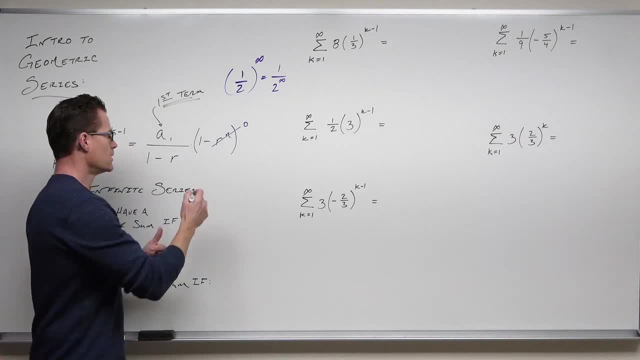 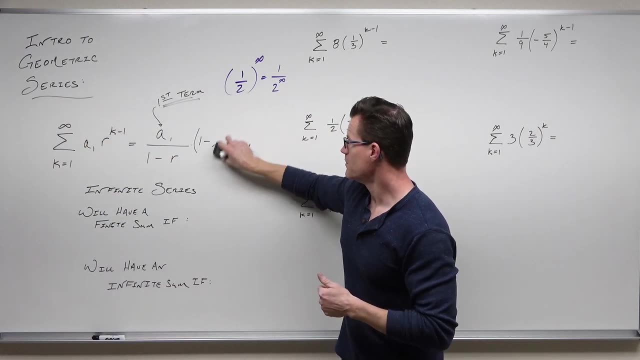 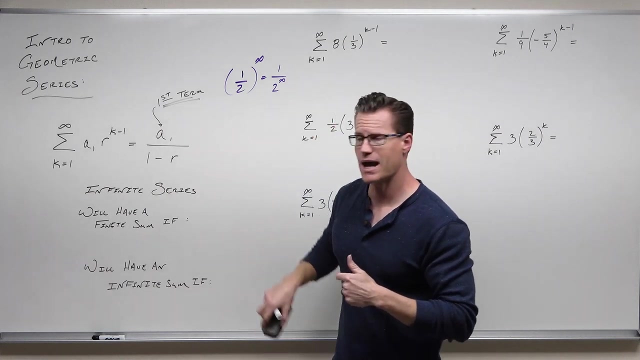 Well, one minus zero is just one. So if I have certain values of a common ratio, this part actually disappears. Why? Because that common ratio to infinity power would be zero. One minus zero would be one One times. whatever I have is whatever I have by the multiplicative. 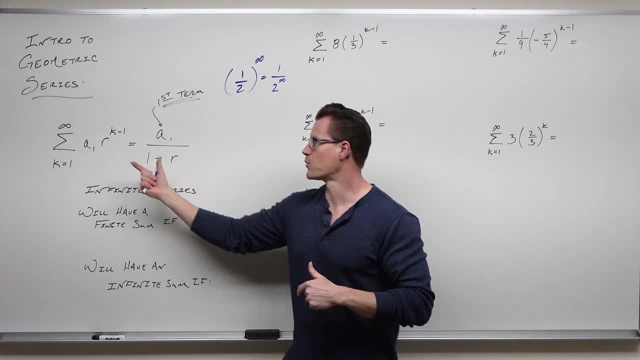 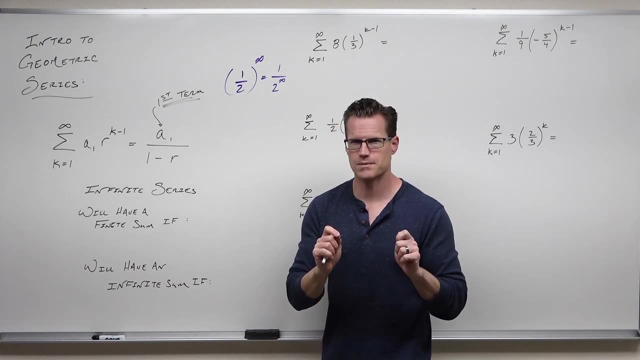 identity that one is. I would just get this for my infinite series, But only if get this, only if r is a certain range of numbers. What are those numbers? You can't just say fractions, because some fractions are greater than one, But one and negative one are the. 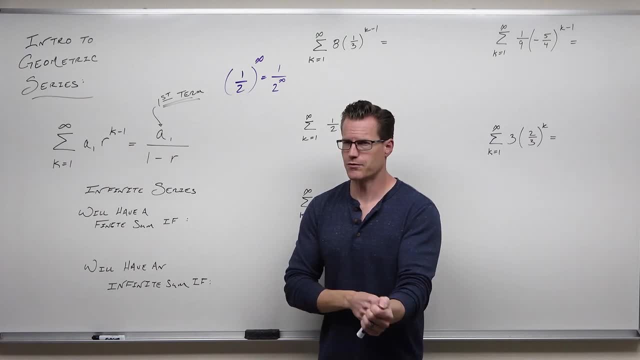 cutoffs here. Man, I hope I made that make sense to you. I kind of went through it fairly quickly. But the idea is, if r is between negative one and one, then when you take it to the infinite power you're going to get close to zero. 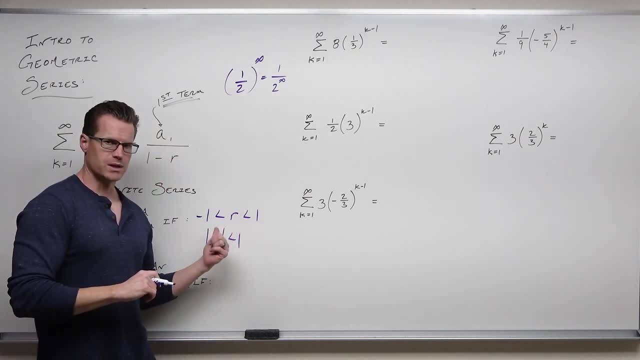 You can say that two ways. If r is a fraction between negative one and one, or if the absolute value of r is less than one, These two things need to be the same in your head. You go: yeah, okay, Absolute value-wise. 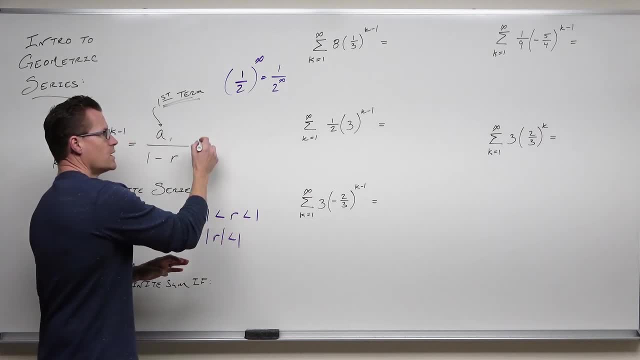 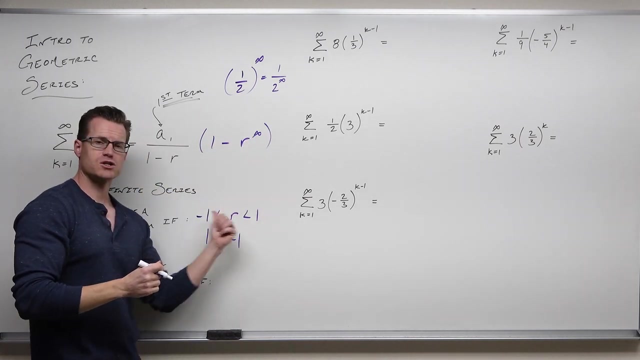 these make the same thing. If this is true, then your partial sum when I take r to the infinity. if we have a fraction, when you take fractions to exponents, as exponents get larger, those fractions get smaller. One minus r to the infinity. if r is a fraction between negative: 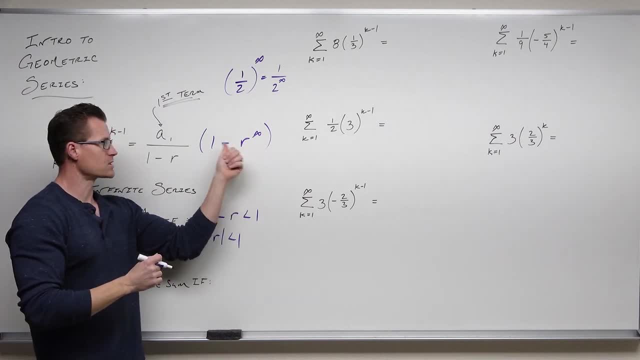 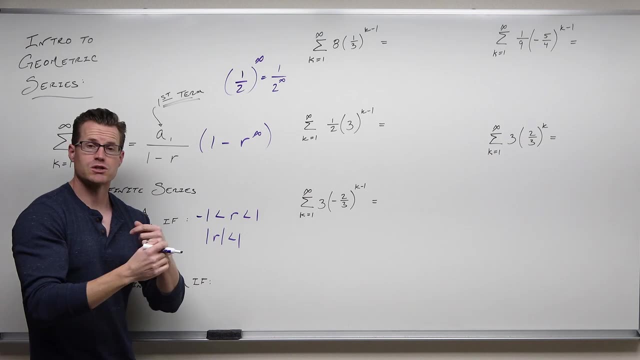 one and one, this is going to go to zero. If this goes to zero, one minus zero is one. This times, one gives you this Only if r is between these two values. So this, only what we call converges, has a finite sum if r is between negative one and one. 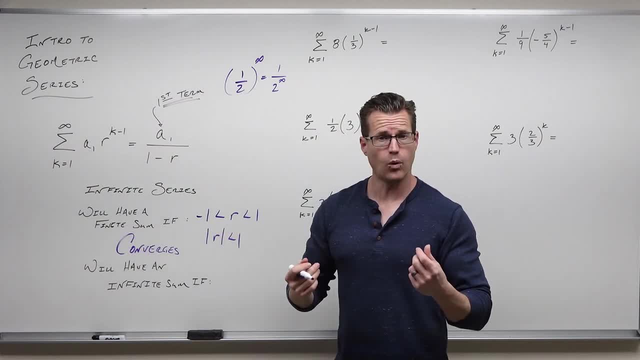 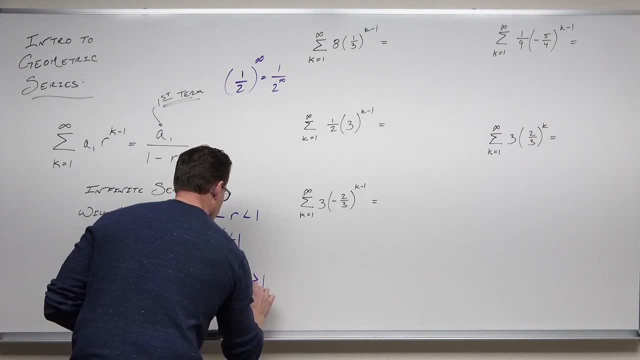 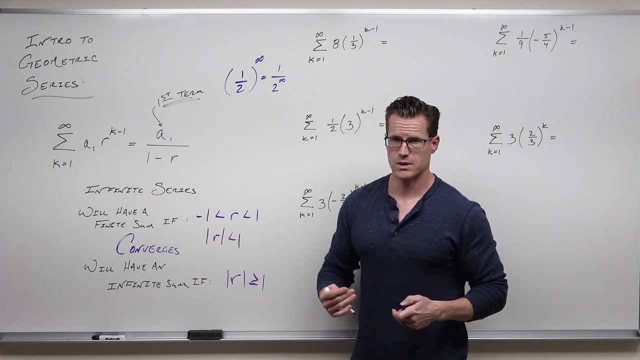 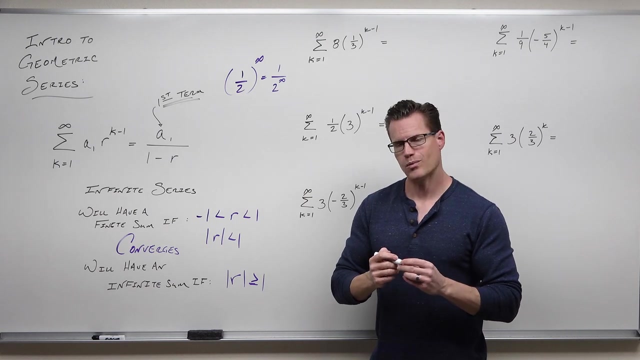 So what happens if r is one or more? So outside of this interval. so less than negative one or more than one, or equal to negative one or one. that's what this says. What if the absolute value of r is greater than one or equal to one? Well, if it's equal to one, then what we would get here is we: 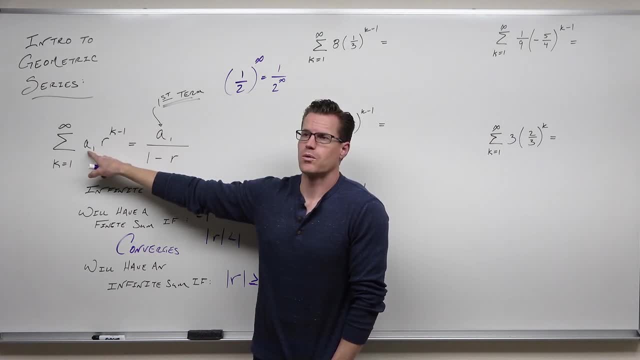 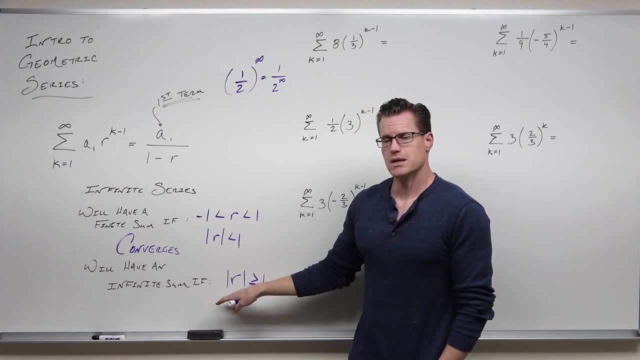 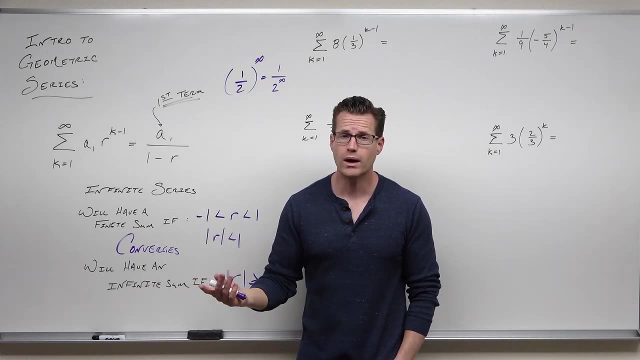 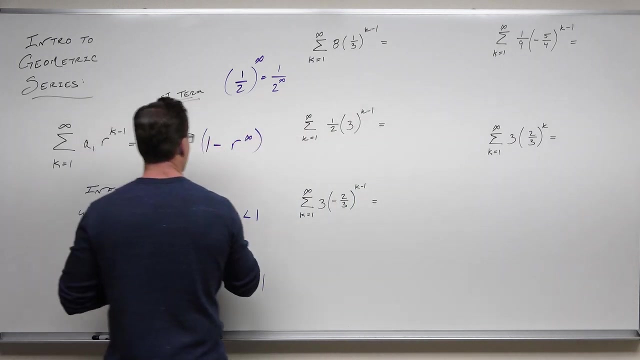 infinity times, you're going to get infinity. This would be diverge or this would diverge. What if r is more than that, like two? Well, it's going to diverge even quicker. So if r is outside that interval. so imagine that. Imagine r is a number like two. Two to infinity. 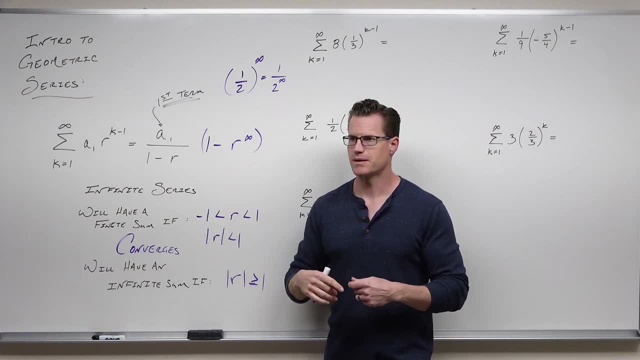 is infinity. You're smoked, You're done, Because one minus something- that's infinity- is negative infinity. I don't care what you have here, It's not going to be zero. Something times negative infinity is going to be negative infinity. unless it's negative, It's positive. 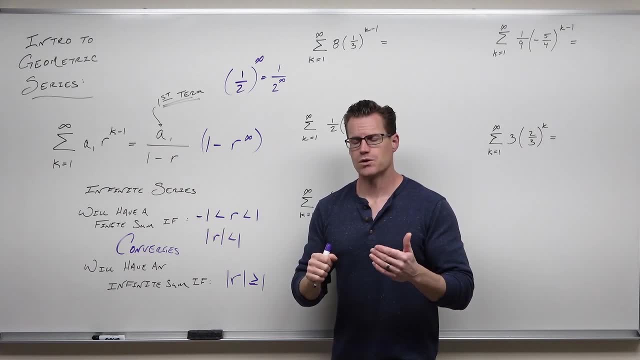 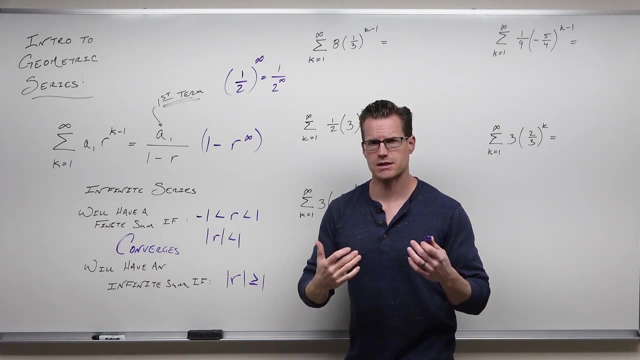 infinity, But you're not going to get a finite sum. So the long story that I just explained is important, but I hope that you understand this more concise wrap-up. If you have fractions between negative one and one, when you take them to the infinite power, you get zero. 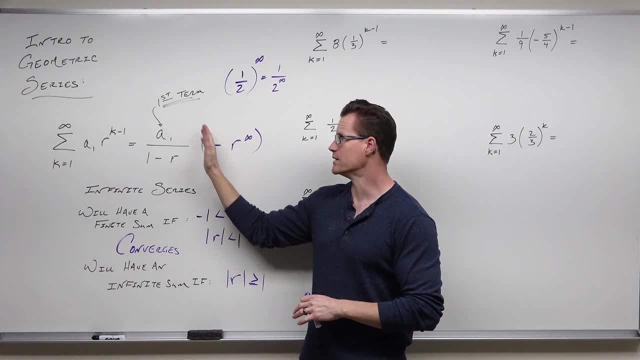 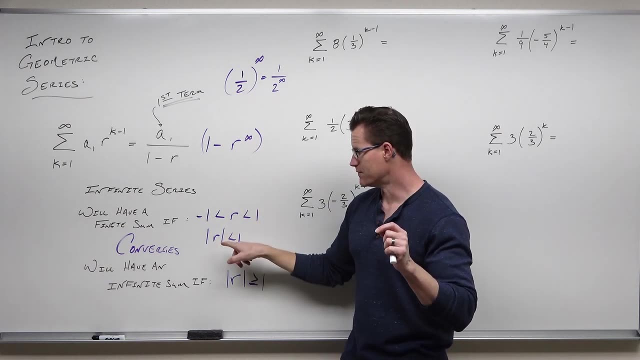 And that means that this part is gone and this would be your sum. It only works if that part goes to zero, And that part only goes to zero if this happens, If your common ratio in absolute value is less than one, or in other words between: 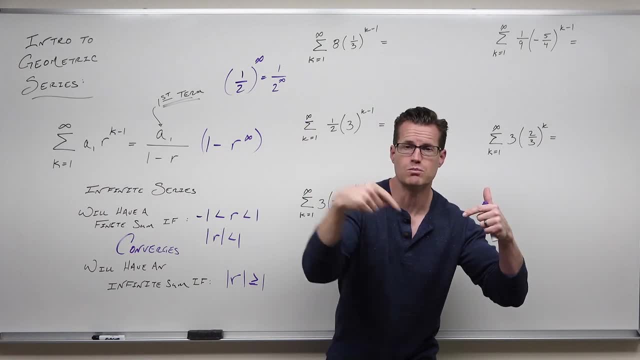 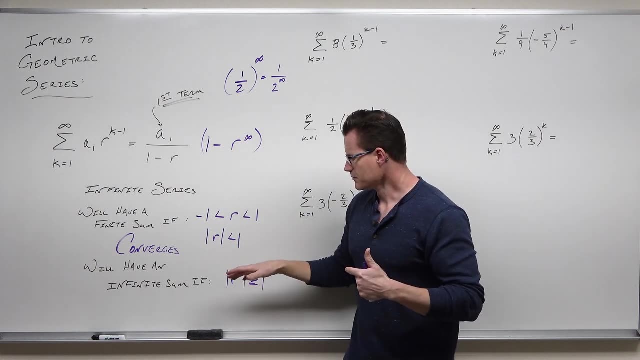 negative one and one A fraction less than one raised to a power gets smaller. That's what we needed to make that not be infinity. On the contrary, if your common ratio is more than one that keeps growing, This whole thing goes to infinity. And if your common ratio 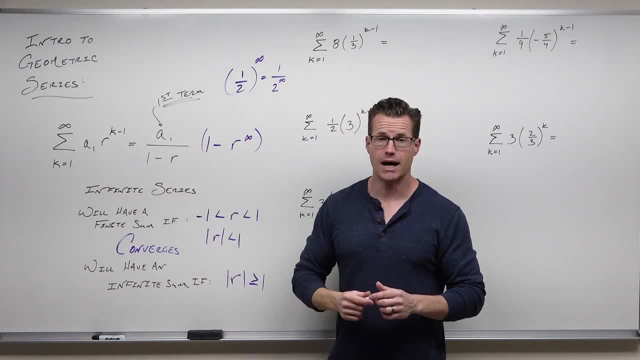 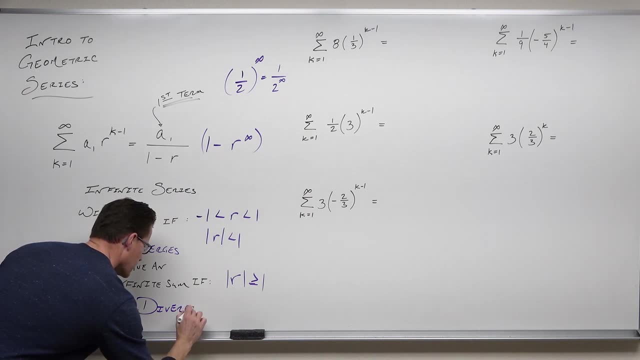 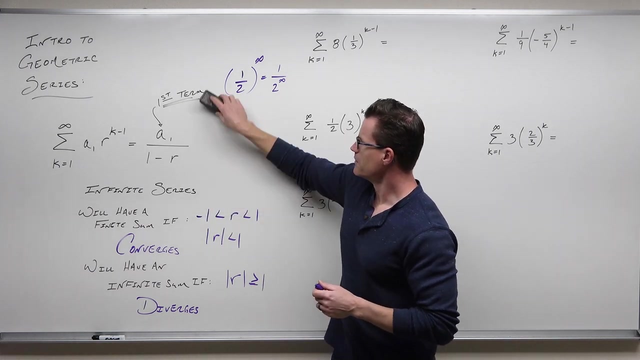 is more than one. that's what's going to happen Every single time we call that diverge Or diverges, we'd say divergent. You might have noticed something too. You might have noticed something. This is not even going to be here. This is the formula that's in your textbook. 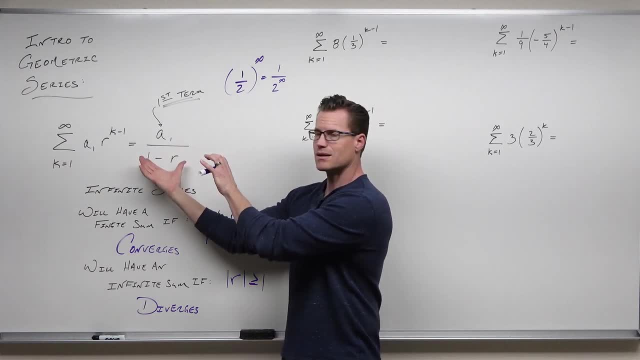 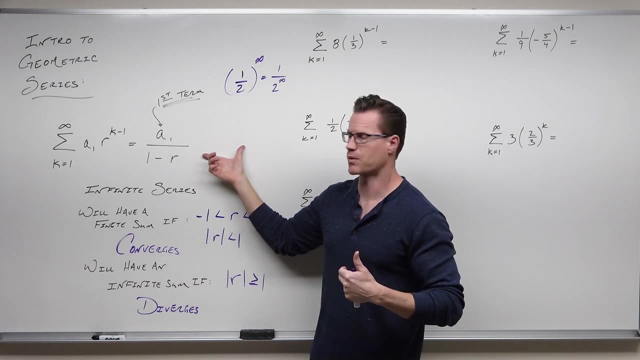 But I just showed you why that was So. why is this? Why did I write it that way? Why did I write it as a sub one over one minus r times some other piece, Instead of the way your textbook writes it as this? 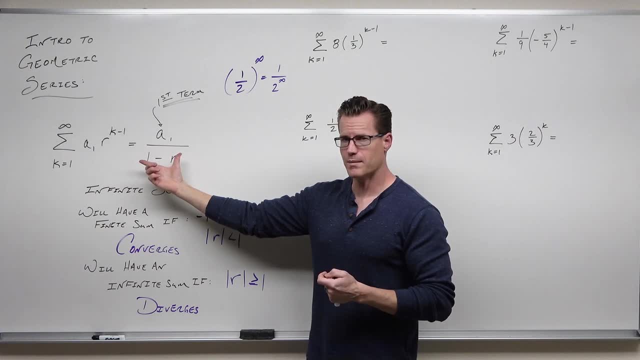 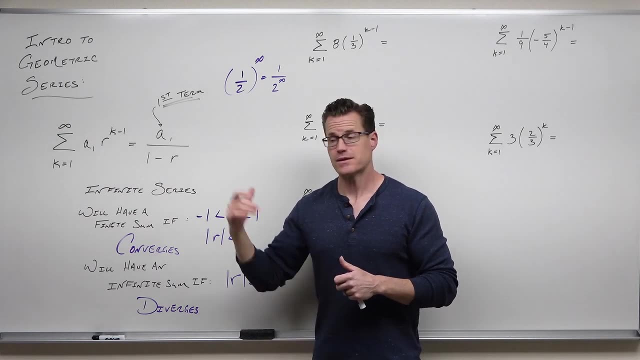 So this: they usually write it as what I have here: over one minus r. This shows you what happens with this. If r is less than one in absolute value, that's going to go to zero, And then one minus zero equals to one. That's great. This gives you the formula. 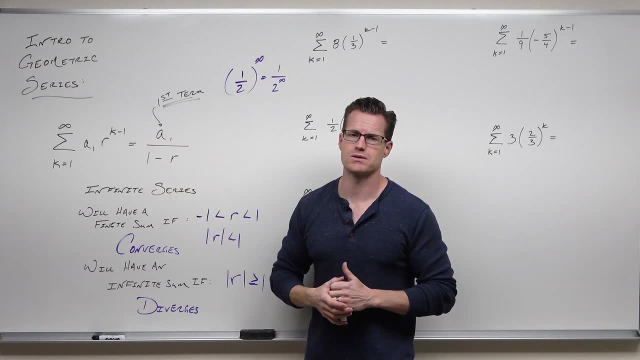 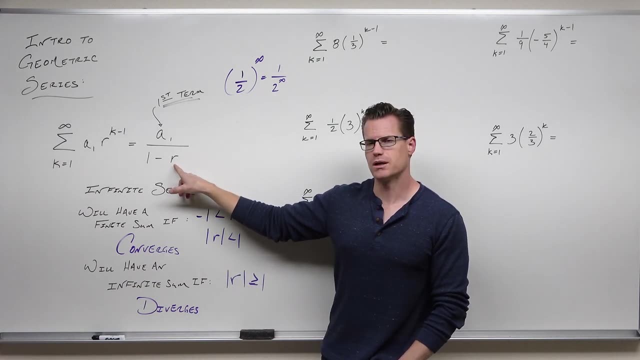 for an infinite series. This is exactly what the formula for an infinite geometric series is. That's where it comes from. But here's the thing You might have noticed: that, no matter what r is, you can still plug it in, couldn't you? You can still find out what. 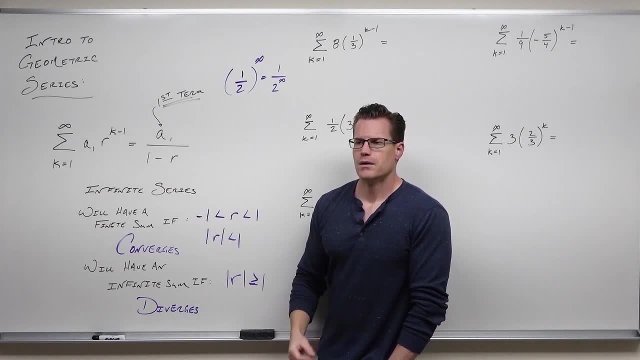 your first term is and you still plug in an R. this means that you're able to find some solutions that mean nothing if your R is more than 1 or equal to 1.. So don't can't equal 1, it's going to be 0. But don't be. 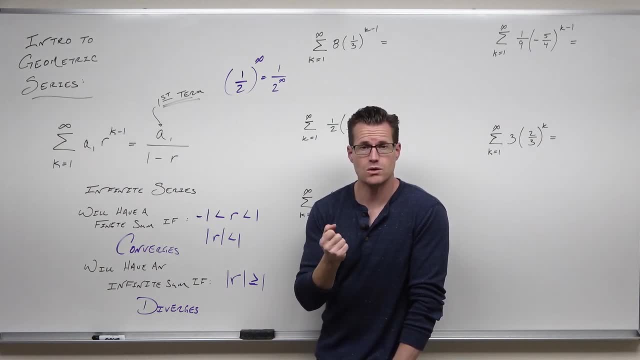 plugging in things if you know it's if it diverges. So here's the order of operations of figuring out your infinite series. Number one: find your common ratio. Number two: determine if it's in the range of numbers, that interval that allows this series to converge to a finite sum. 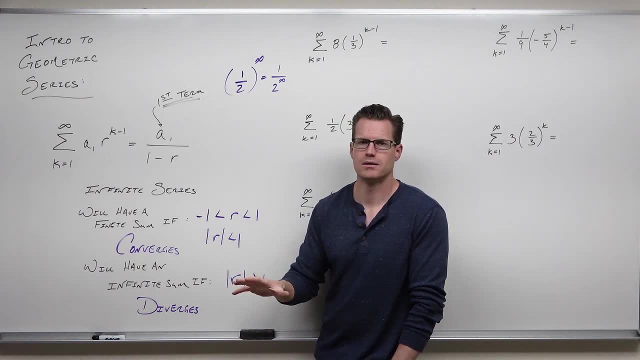 If it's not, just write diverges and you are done. Give me 30 problems that diverge. Probably think I'm tricking you. But write, just write, write, diverges if your common ratio is more than 1. You're done. Now, if it's not, then you find your first term, just plug in 1, whatever it is. 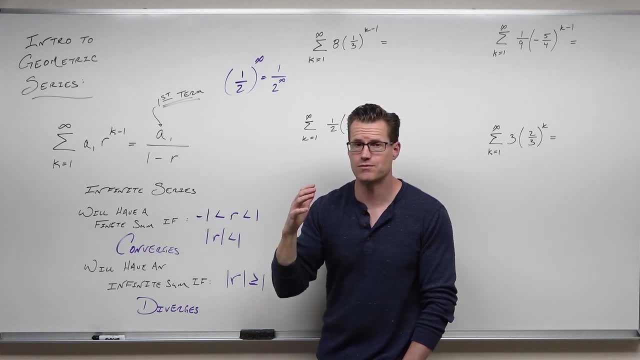 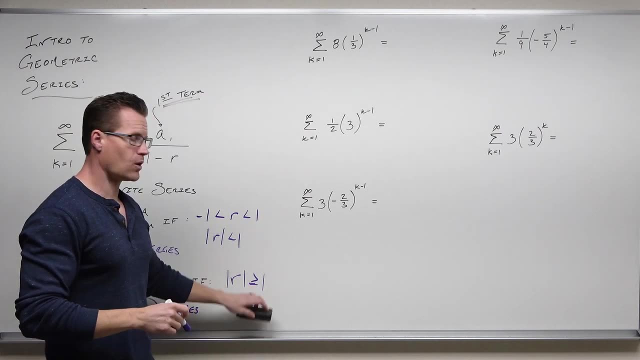 plug in your first term and then divide by 1 minus your common ratio, And it's very easy, It's not bad. So we're going to run through our five examples here. I'll reiterate this. I'll talk about how taking that partial sum and letting your n go to infinity is how we're. 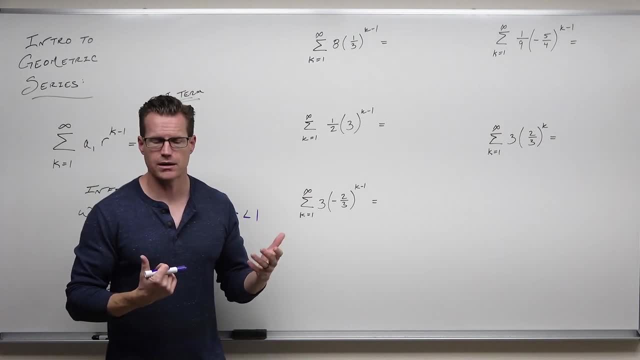 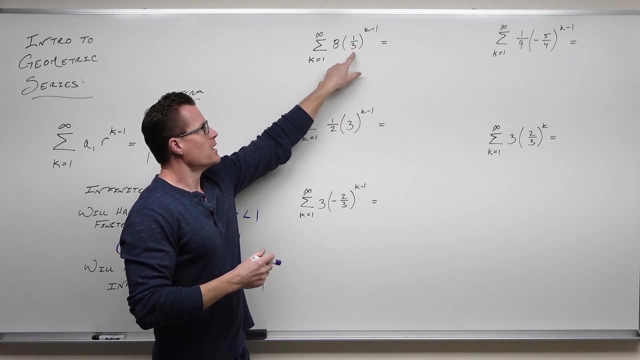 finding this and what would happen if your R is less than 1 in absolute value. So we take a look at it. Is that a geometric series? Well, yeah, it's got a, it's got a common ratio. It's being 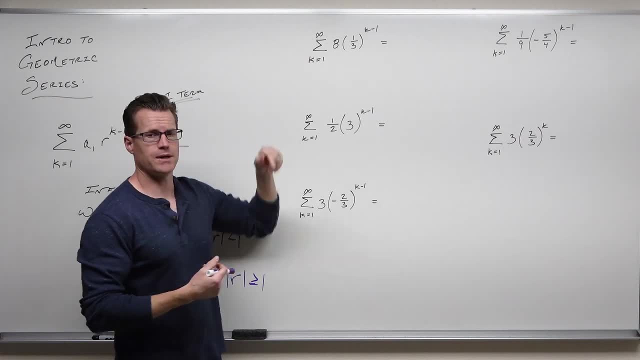 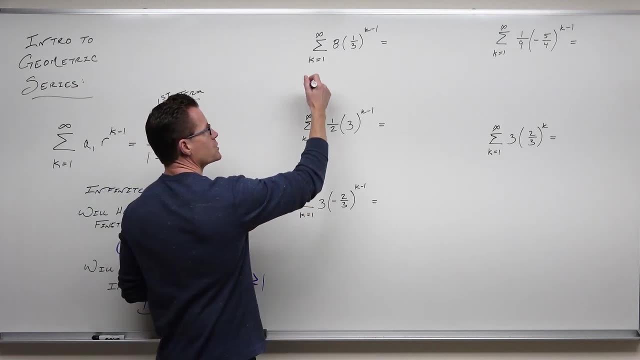 raised to an exponent. Is it an infinite series? Yeah, it's got infinity, So we're we're getting used to this. right now. The first thing we do is we identify what our common ratio is. So our common ratio is one third- It's always the thing in parentheses- being raised to the 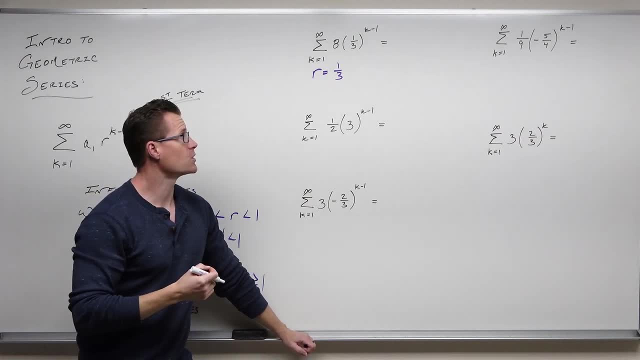 exponent In general, it's the thing being raised to the exponent. So our common ratio is one third. Now classify it. If our common ratio is between negative one and one, this infinite series will converge. And we talked about why. If I take one third to the second power, 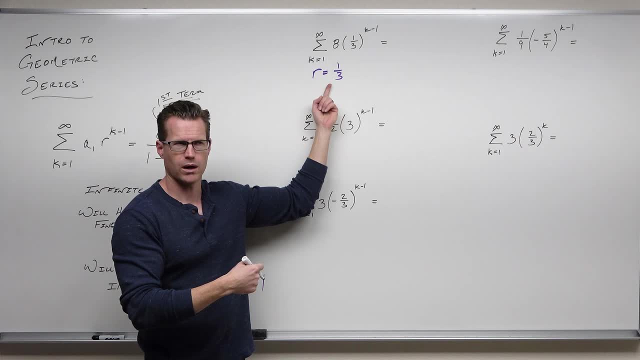 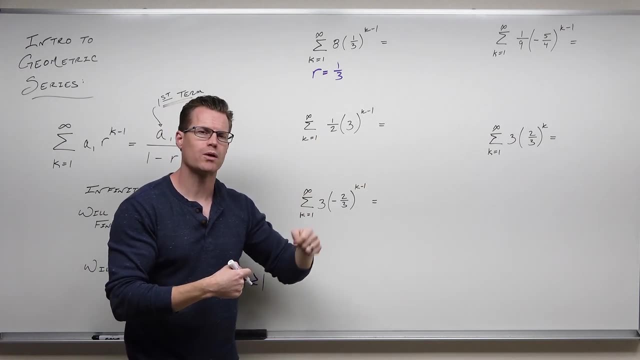 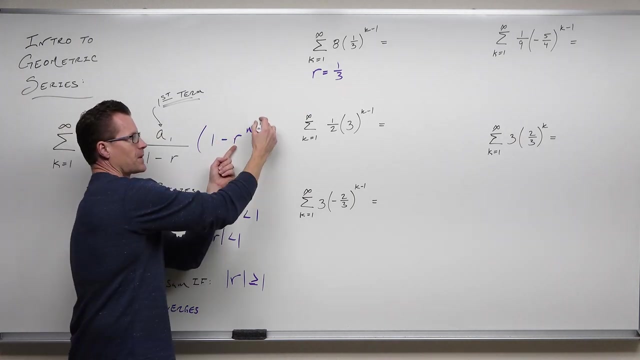 I'm going to get one ninth. How about to the hundredth power? Well, I'm going to get something really, really small, In fact, to the infinite power, so small it doesn't matter. So the formula we had before says: if my one third goes here and my n gets absurdly large, then this gets absurdly. 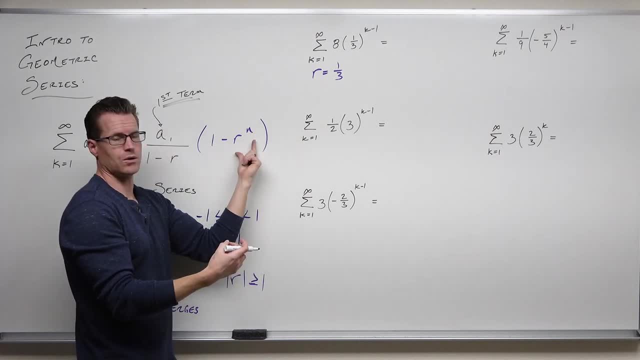 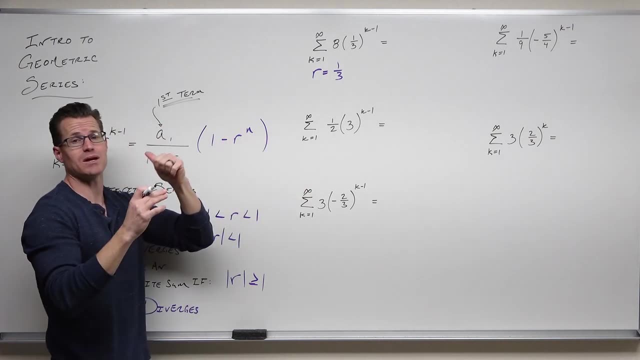 small, One third, to the infinity. it's going to be zero. One minus zero is one. That's why that sum actually works for an infinite series, because this disappears, but only if your fractions are between negative one and one. That's exciting. That's very interesting. We're using some pretty 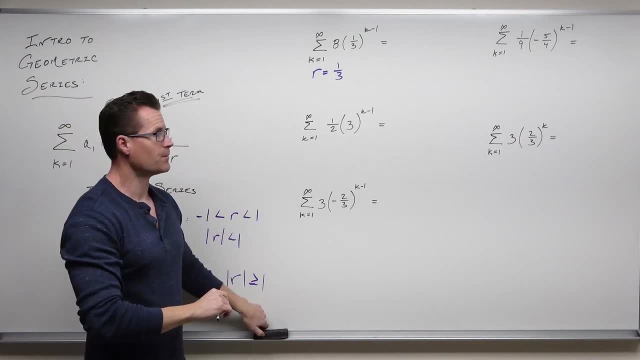 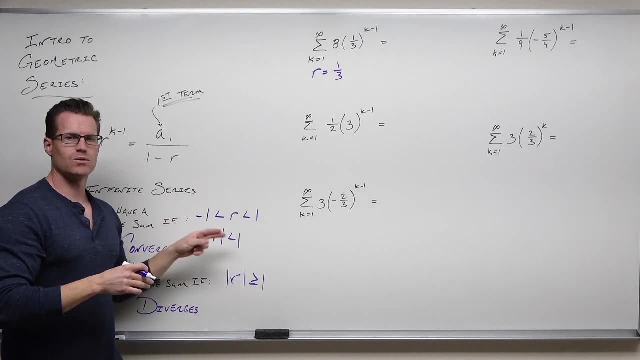 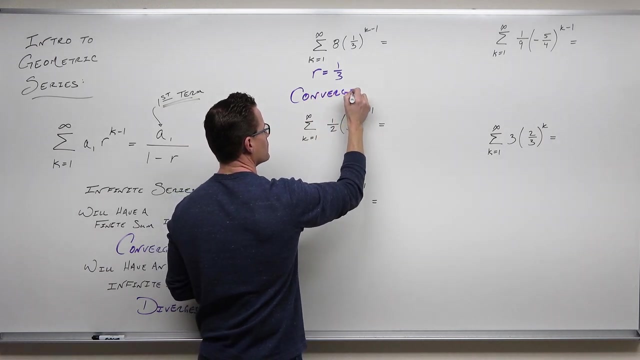 cool stuff here. Most people never get that. They never see that, ever. So we're going to determine our common ratio. We're going to say: this fits here. This is less than one in absolute value. That means that this series will converge. And now, after we've determined that it converges, 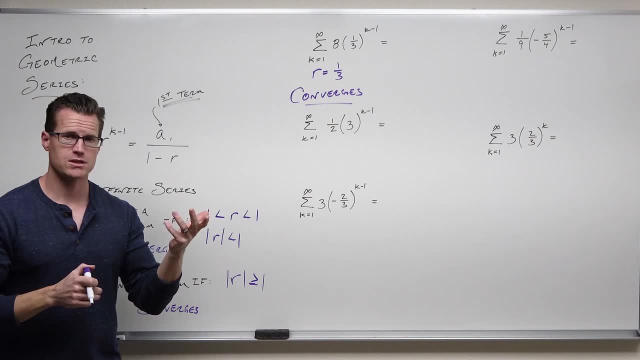 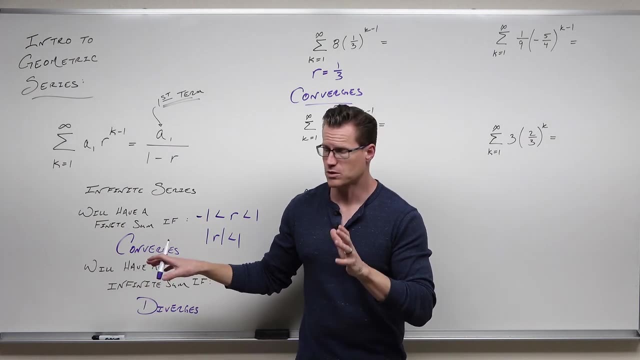 we're going to find the sum. You see, it's really pointless to say diverges and then try to find the sum. When you say that this diverges, you're saying the sum goes to infinity. That's what you're saying. So diverges says it doesn't go to. a number goes most of the time, goes to infinity. 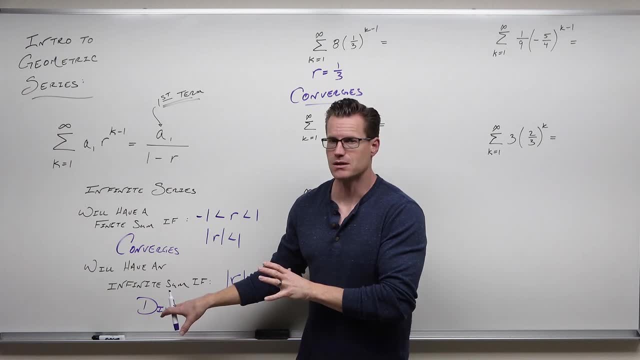 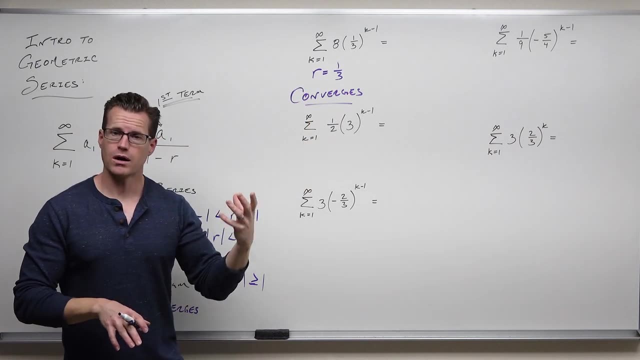 or negative infinity. So you're saying that right here, saying it doesn't have a sum. That's what diverges mean: It doesn't have a finite sum. Okay, So it doesn't have a finite sum, Why would you go and find it? if it diverges, If it converges, it's saying it does have a finite sum. Now, once we 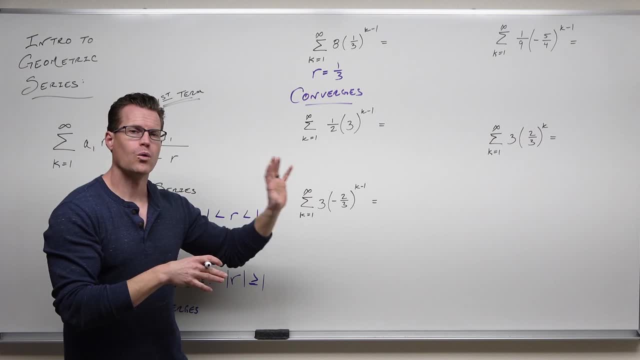 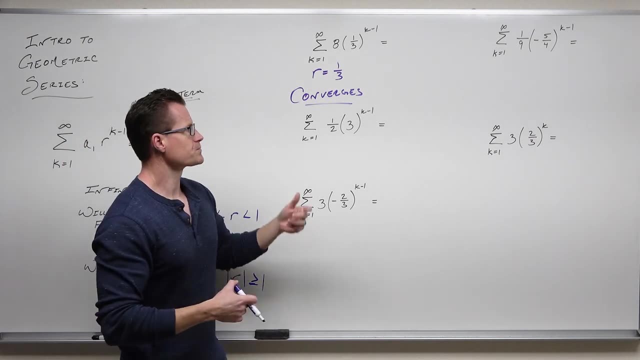 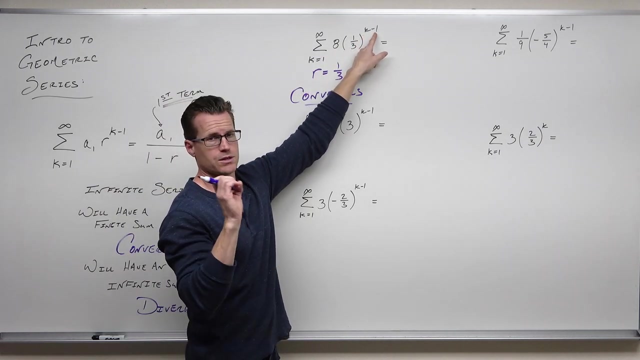 determine it converges. we find it How we always find the sum of a geometric series is: find your first term, then divide it by one minus your common ratio. So what I always do, I just plug in one. I don't care what form it is, It does not matter, Just plug in one. So one minus one is zero. 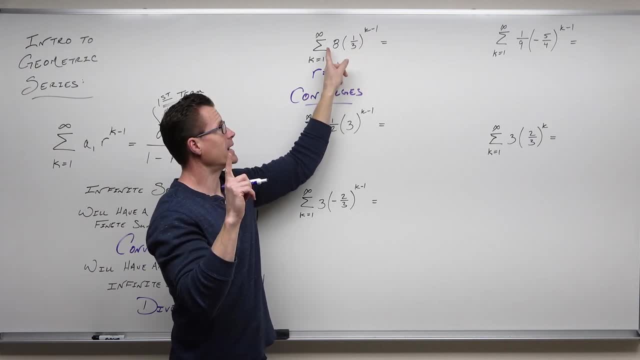 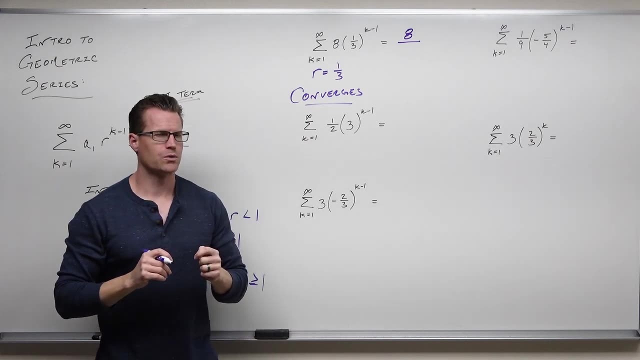 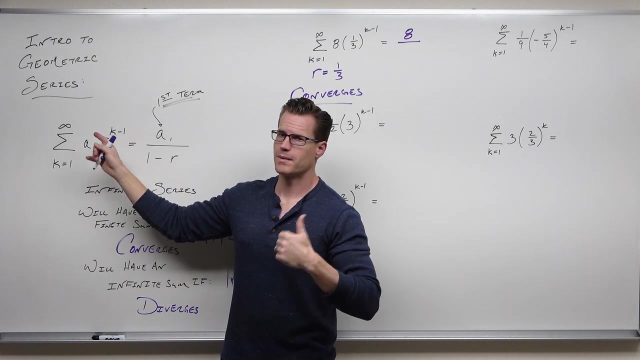 One third to the zero. power is one And eight times one is eight. What I walked you through that whole one minus one is zero thing. That's why this is written as first term here, Because if I plug in one, one minus one is always zero. Common ratio is zero, power is always one And one times this is. 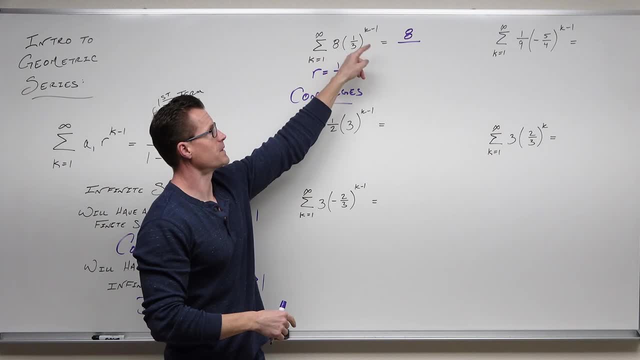 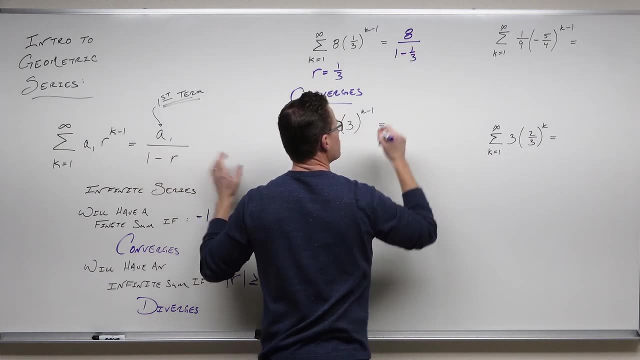 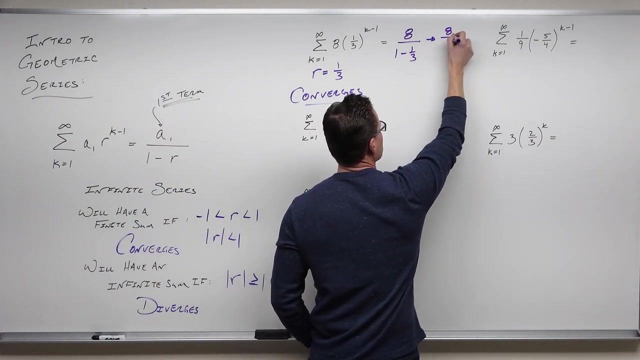 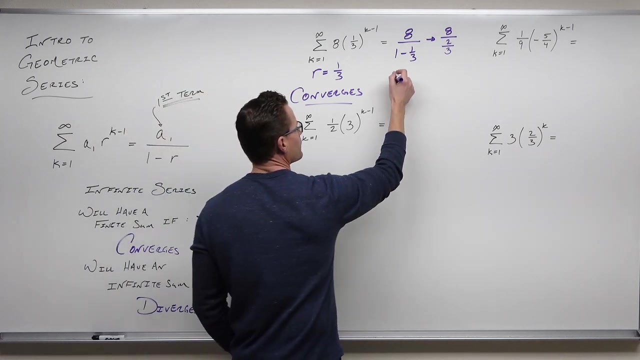 always going to be your first term, So that's why that's your first term. here is eight, Then divide by one minus your common ratio. Simplify it a little bit. So this is eight over two thirds. I think we get twelve out of that. 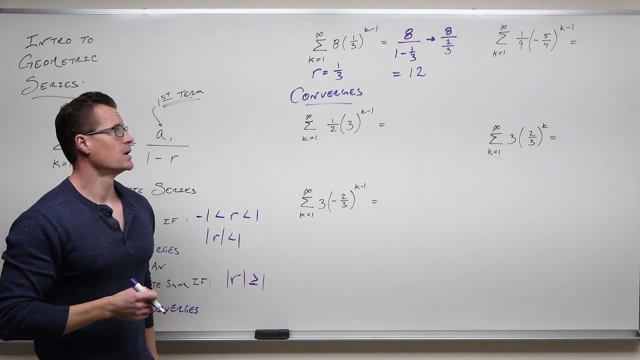 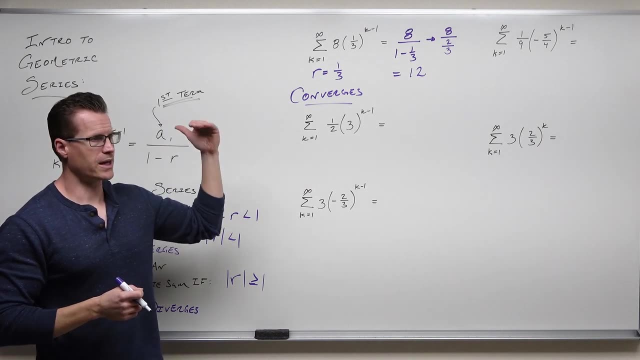 Number of ways you can do it Use your calculator. Eight divided by two thirds. You can do eight divided by two times three, And it would give us twelve. You could both, by both the numerator and denominator by three, and get twenty-four over two, Which would also give us twelve. Now I mean the 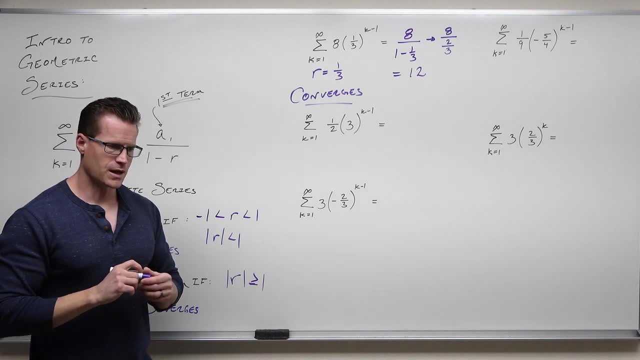 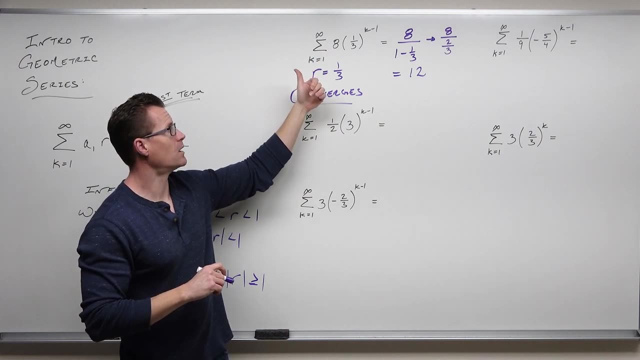 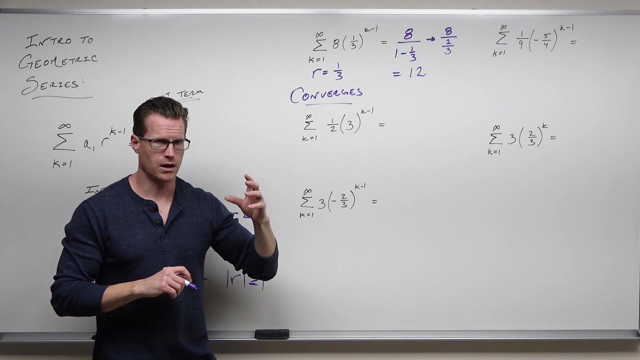 first time I saw this it kind of blew my mind, Like wait a minute, you're telling me that I can take this and I can start writing out my terms of my series, Like: plug-in one, you get eight. Plug-in two, you get eight over three. Plug-in three, you get eight over nine. And I can do that forever. 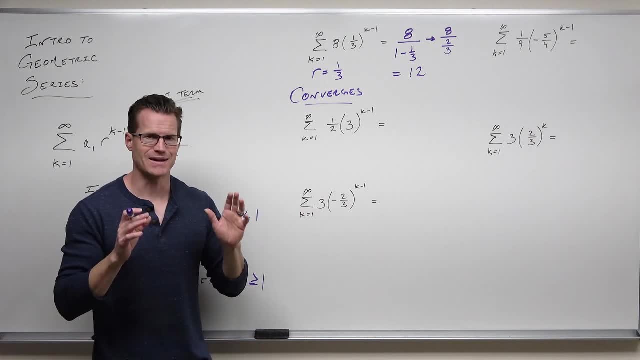 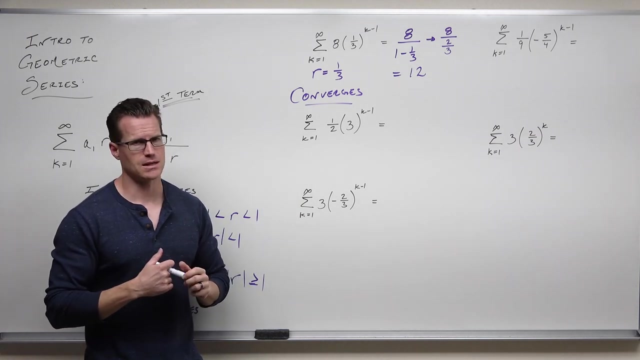 and then add them all up and it's going to equal 12.. Like, exactly, Yeah, that's exactly what this means. Why? It's because that fraction being between negative one and one, when I take that to very, very large terms, ends up being zero. It all matches up to give you 12.. It's a fascinating. 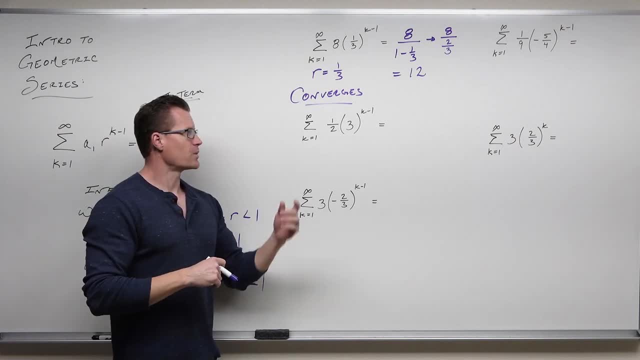 piece of math. Let's move on a little bit. So we have another geometric series. We know. oh, can you identify your common ratio? Can you right now look at this and say: common ratio is the thing that's being raised to the power? It's not one half, it's three. Can you identify your? 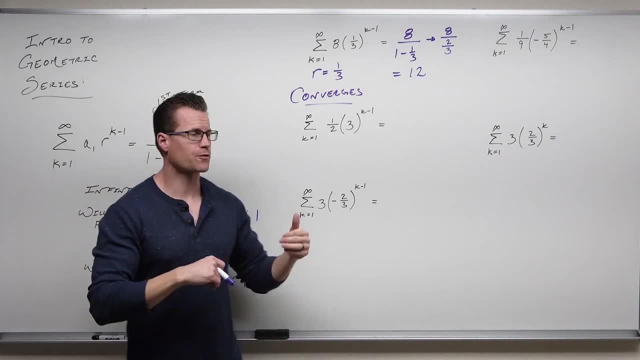 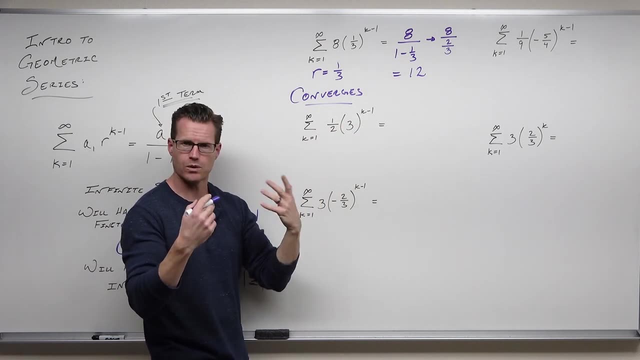 first term, if you had to. Well, it fits our form, and so our first term would be one half, Or plug in one. One minus one is zero. Three to the zero power is one. One times one half is one half. Now, before we find any sort of sum, we need to identify the 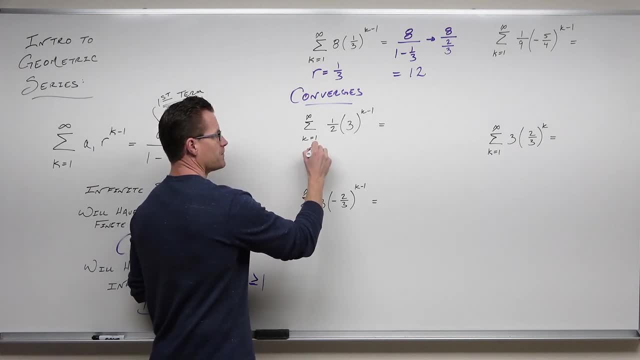 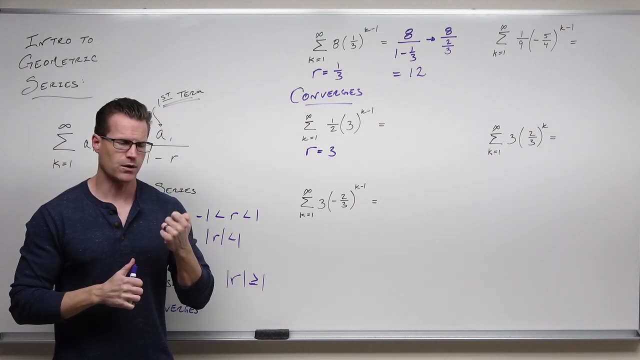 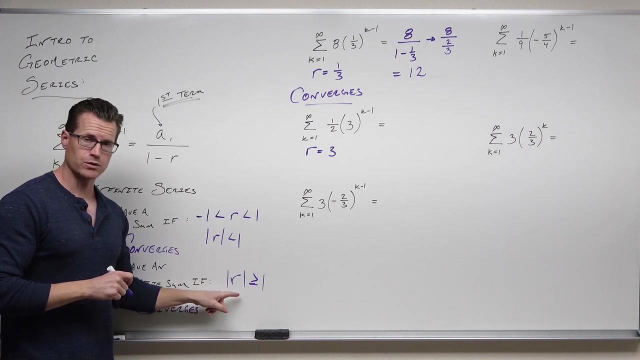 two things that are very, very important. Number one we already did: R is three. So if R is three, think about what that means. If our common ratio is three, three is not less than one. Three is more than, greater than or equal to one. Now why would that make a difference? 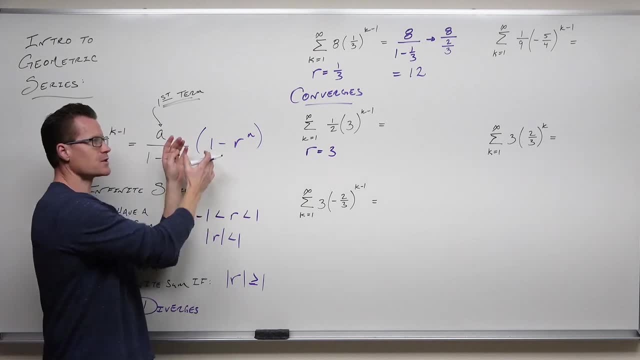 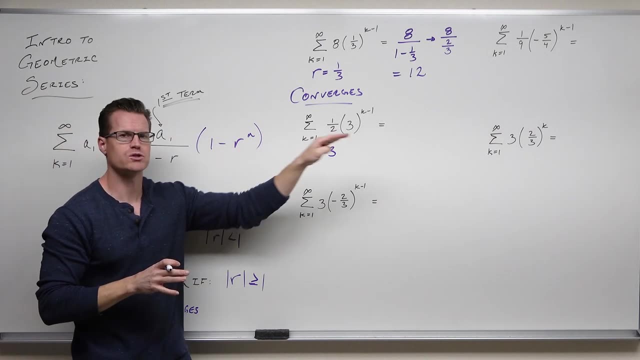 Imagine plugging in one Three here. Think about this. This is the formula for a partial sum. We're just letting this go to infinity. It's only part of this that can change, because we're the only part we're letting go to. 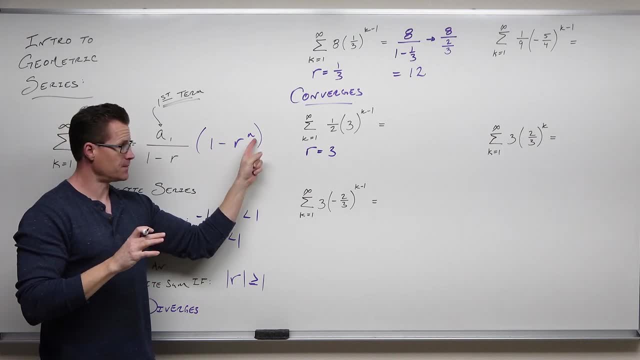 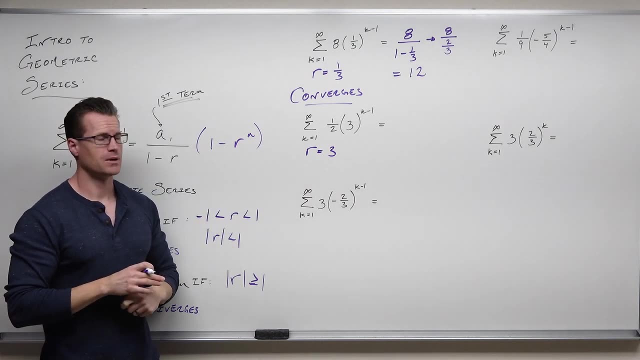 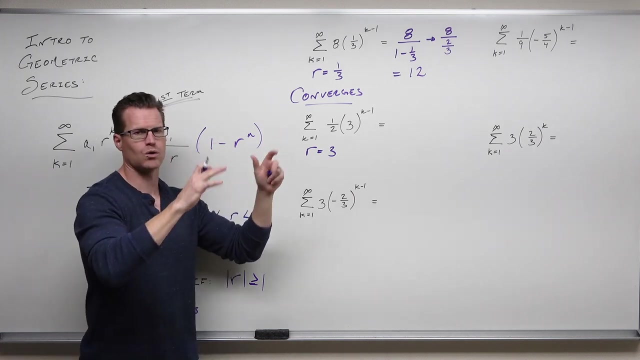 infinity. So if this goes to infinity, then three to the infinity is enormous. One minus that is really negative, And that's our first term of one half. This is going to negative infinity. There's no way that this could ever go to zero, because three to the infinity is enormous, So this would 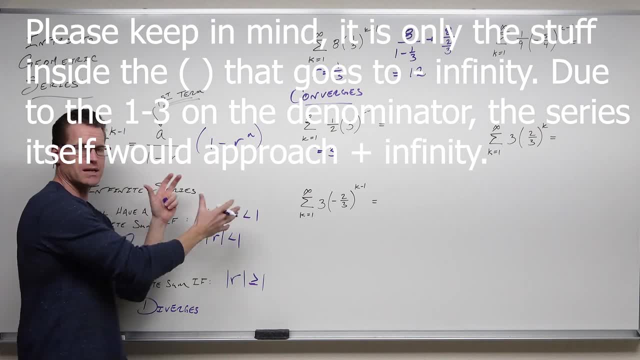 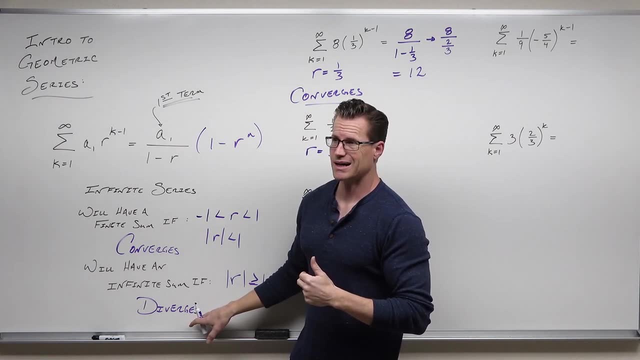 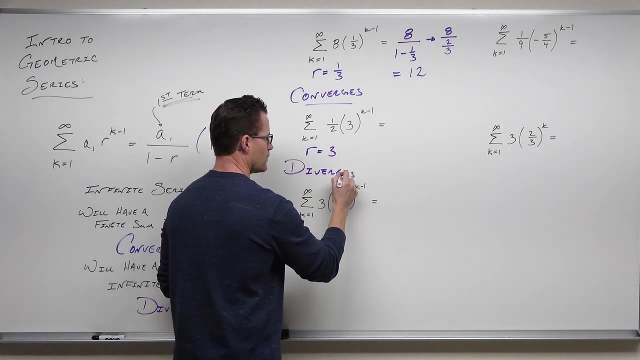 diverge, And that's why I'm trying to walk you through why this makes sense again and again, so that it'll stick with you. So this says, yeah, your common ratio is more than one in absolute value. It's going to diverge for the reasons we just talked about. So would it benefit you? 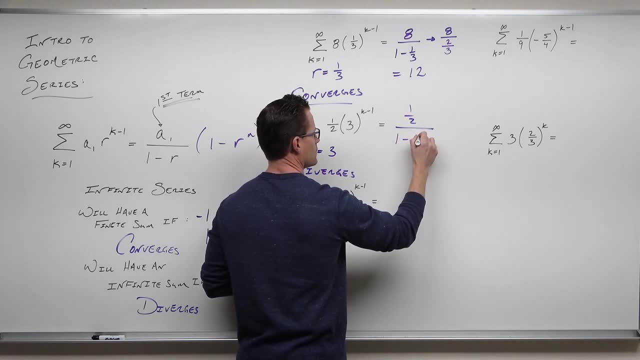 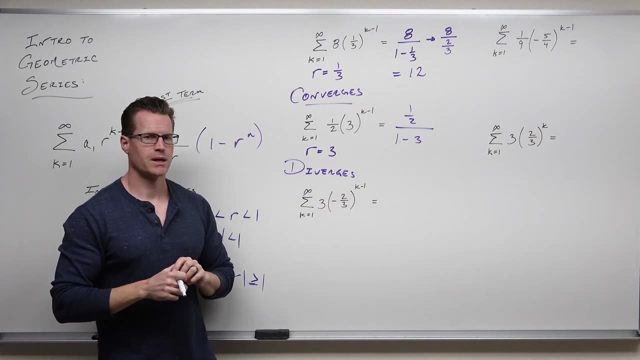 to do that. Would it benefit you to take your first term divide by one minus your common ratio? Would it benefit you to take your first term divide by one minus your common ratio, One minus three? Notice how you can get an answer, but notice that we already said it's going to. 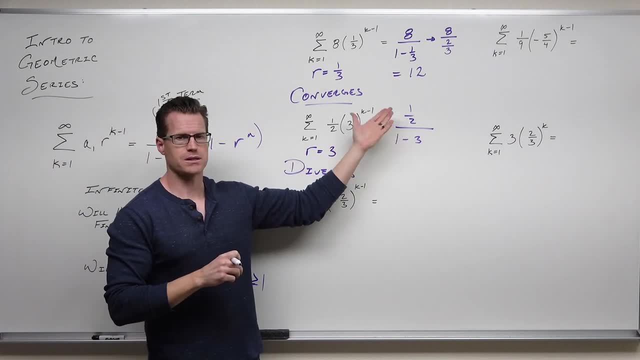 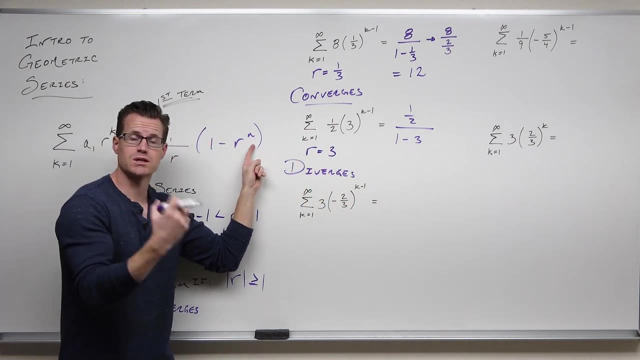 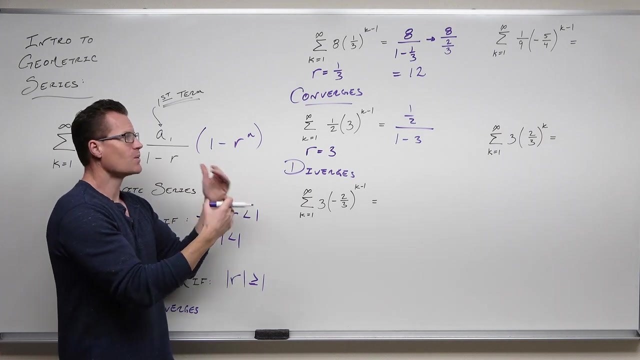 negative infinity. I showed you that right here. This is nonsense. It's absolutely useless. This only works if this thing goes to zero. This thing only goes to zero if your common ratio is less than one in absolute value. It's the only way it works. So if you, just if you- go well, I mean. 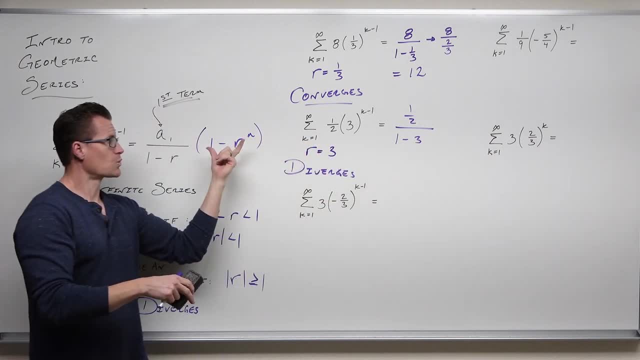 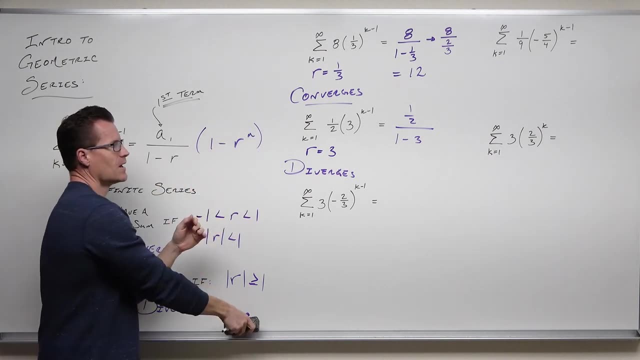 I'm just taking this piece of it. Look what you're missing. You're really really missing this. This is the formula. This only disappears if r is less than one. So this is the formula with this here, And you start eliminating this piece The only way you can. 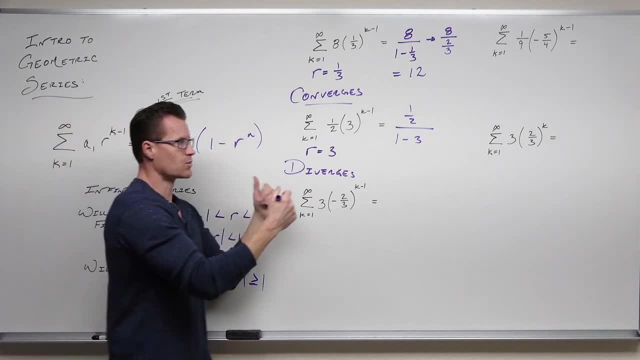 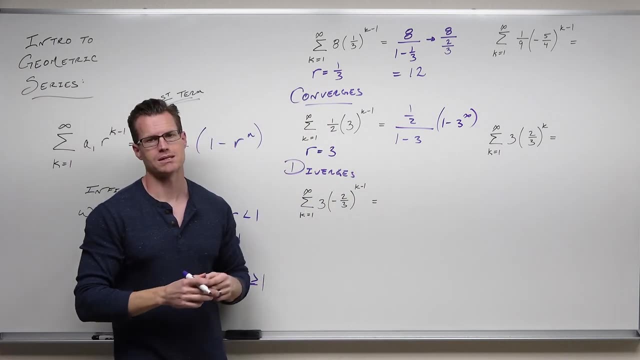 eliminate it is if your r is less than one. If your r is three, then really what you would have here is the missing piece that you're taking for granted that works, even though it doesn't. It's not going to work for diverges. If you write diverges, that's going to negative infinity in. 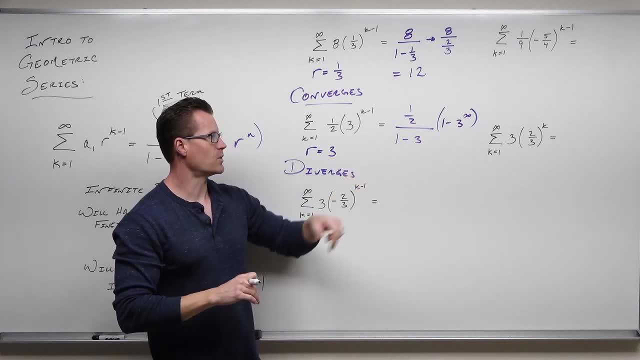 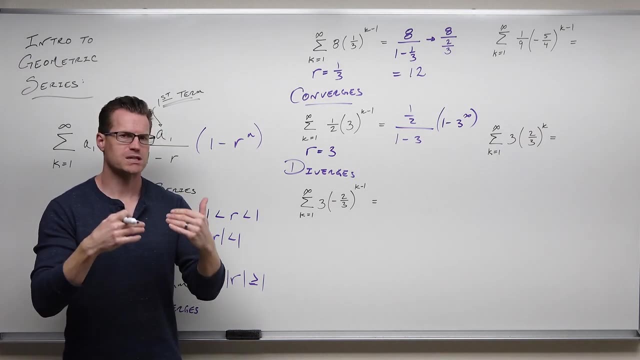 this case. No, I should pause and think, because that right there would give you a negative, So that would go to infinity and you cannot add this up. It's impossible. Here's what I hope you're seeing right now. I hope you're seeing that the only reason this disappeared- 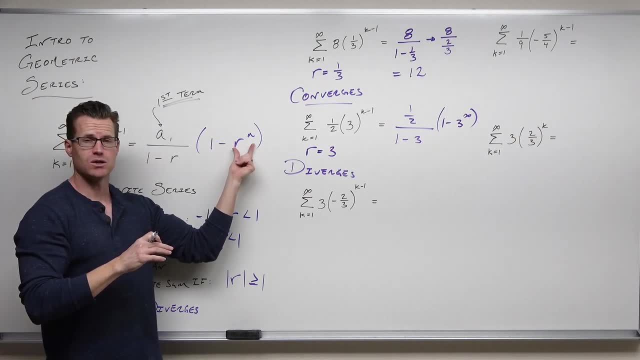 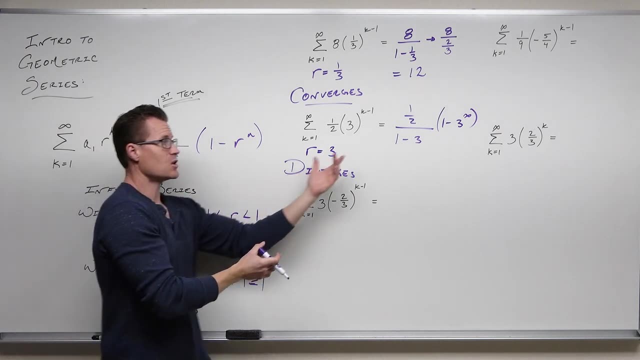 from our partial sum to our infinite sum is because that piece goes to zero in certain cases. If that piece is not going to zero because it does not qualify for those certain cases, you basically can't eliminate it, And then this does not work without that piece And with that. 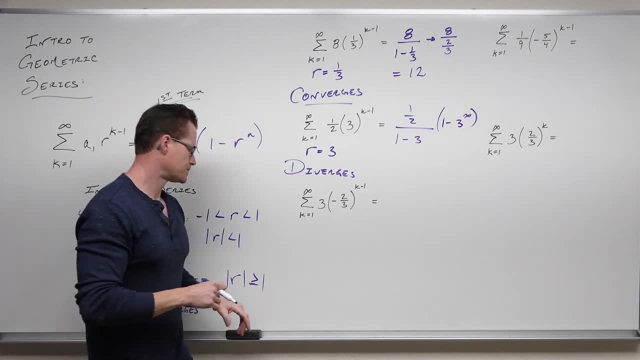 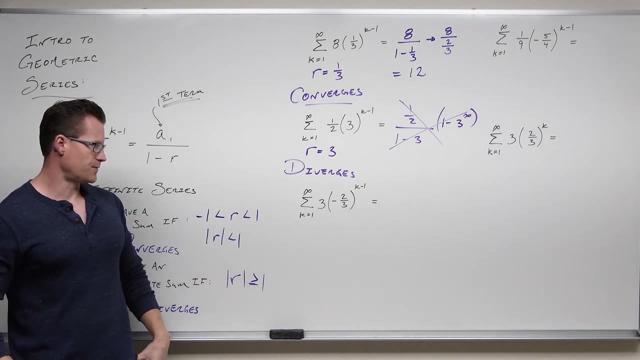 piece, it goes to infinity. That's the idea. So we don't want to show that, Let's move on to this guy. So we have a series of, from k equals one to infinity, of three to the negative two-thirds to the k, minus one Negative two-thirds to the k. 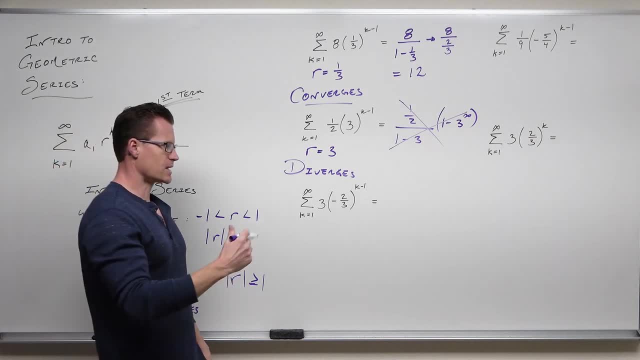 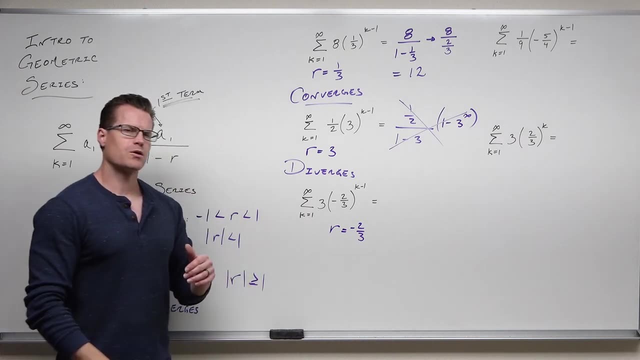 minus one. First thing we always do: we identify what the common ratio is. In our case, the common ratio- the thing being raised to the power- is negative two-thirds. We look back over here. we think about it. Just thinking about it is enough. Think about how your partial sum was. 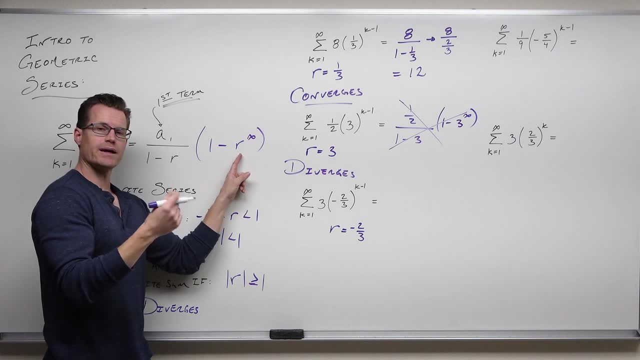 and now I'm trying to plug in negative two-thirds, That's a fraction less than one, Fractions less than one, between negative one and one. raised to infinite powers, or raised to any powers, gets smaller and smaller and smaller. This thing, if I raise it to the infinity, is going to be. 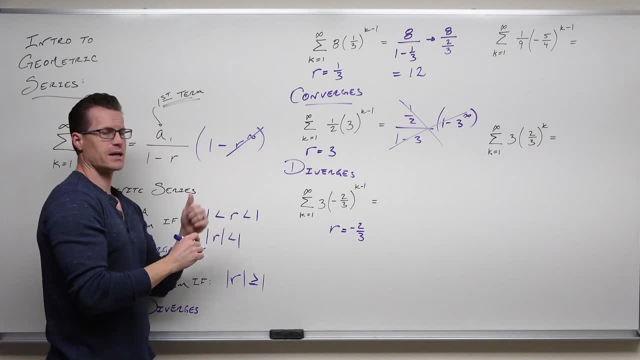 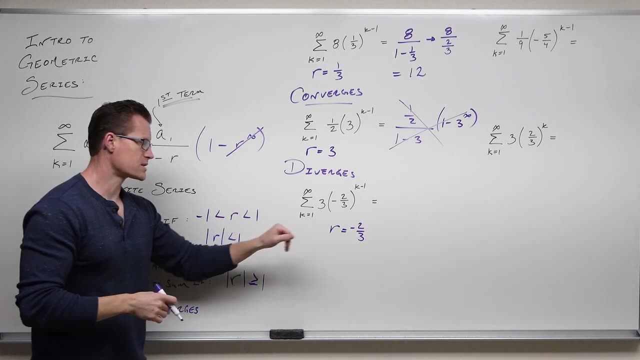 close to zero, That disappears. One minus zero is one. I get this, I get that sum out of it, and that's why this is so valuable. So I know that, because of that, because my common ratio is between negative one and one, this will converge. 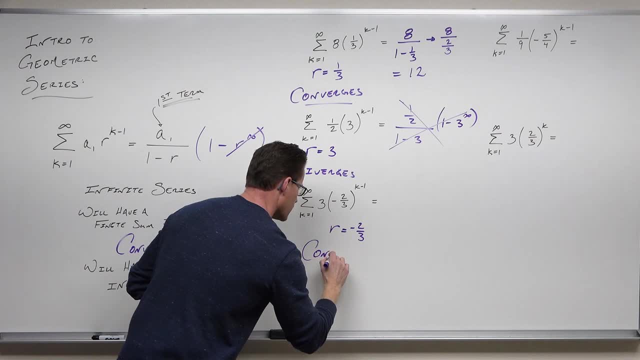 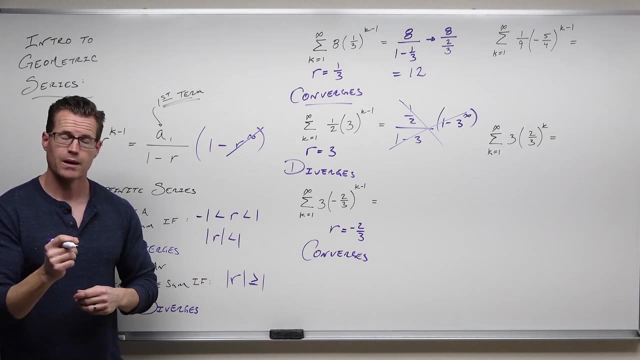 It will go to a finite sum. All right, if it converges, we need to find out what it converges to. So let's find our first term, because we know that's going to work. Let's find our first term. 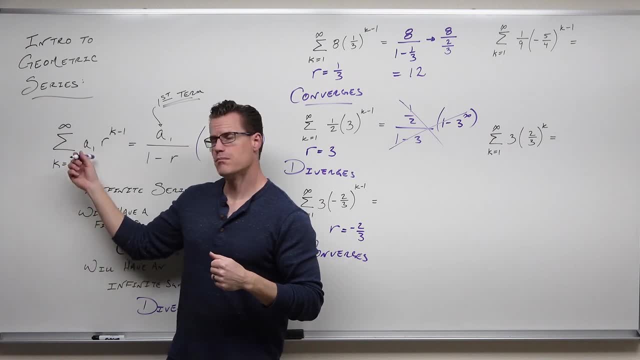 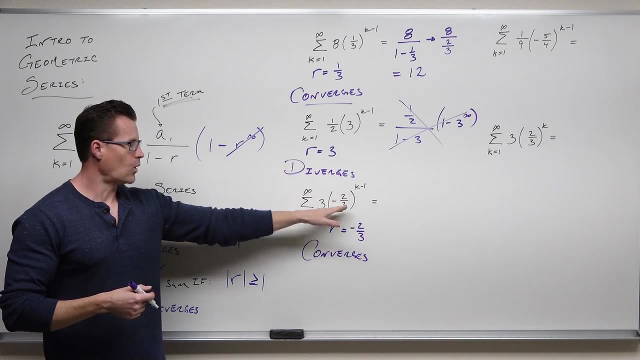 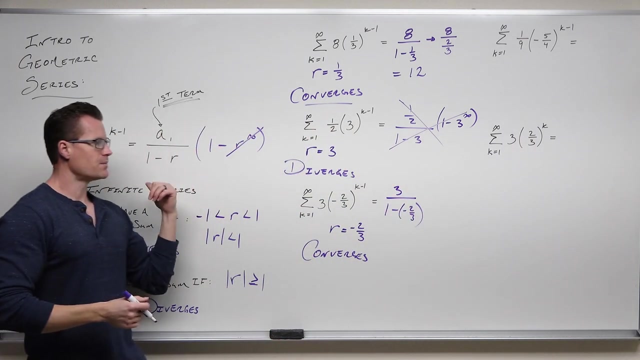 either plug in one or, if it fits your model perfectly, take your first term. It's going to be three. One minus one is zero. Negative two-thirds to the zero powers: one and one times three is three Divided by one minus my common ratio of negative two-thirds. Just be careful on your signs. You. 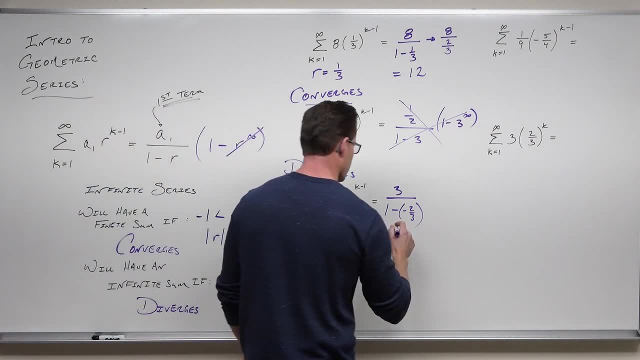 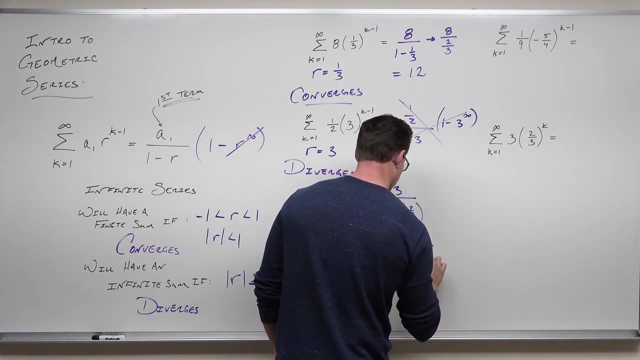 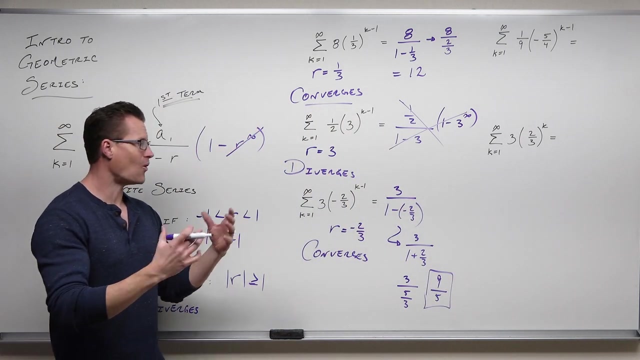 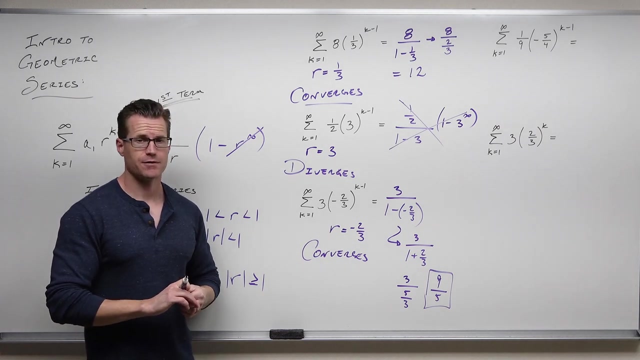 are subtracting a negative, so you're going to be adding that. So let's see, Three-thirds plus two-thirds is five-thirds, That's going to be nine-fifths. So if I add all the terms from here to infinity, from three to infinity, you're going to get a sum of nine-fifths. 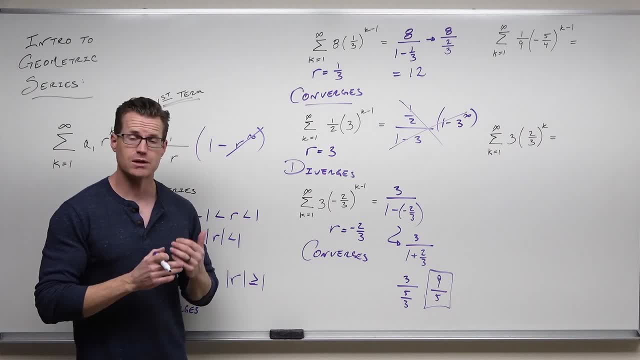 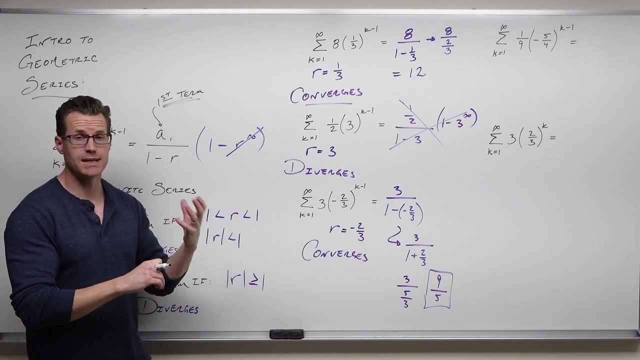 Really, really cool stuff. I hope I'm making it make sense, that you're seeing why this piece goes disappears if r is between negative one and one- I hope you're seeing that- and why it doesn't if r is greater than one in absolute value. 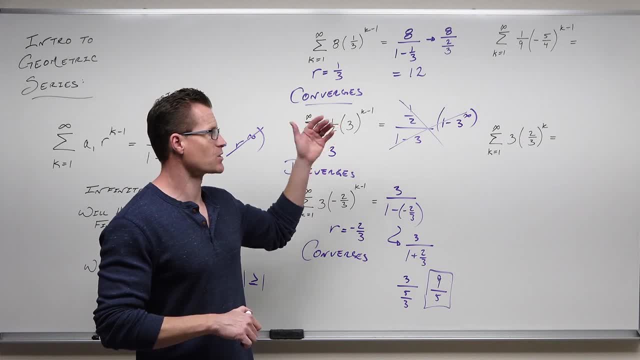 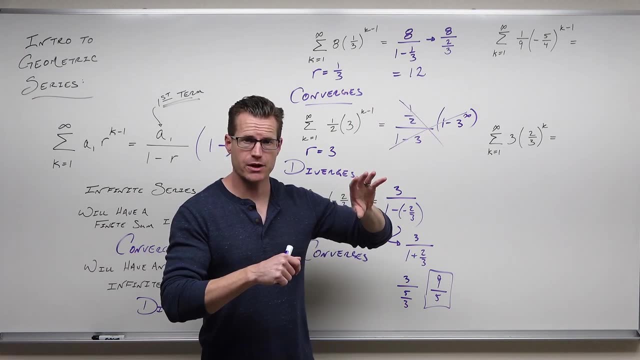 Okay, just two more. So we're taking a look at this. We're going to move a little bit quicker on these things. This next one: we have an infinite series, from one to infinity. We're identifying what our common ratio is. 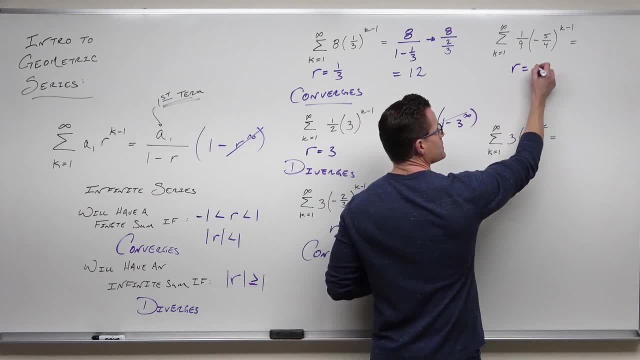 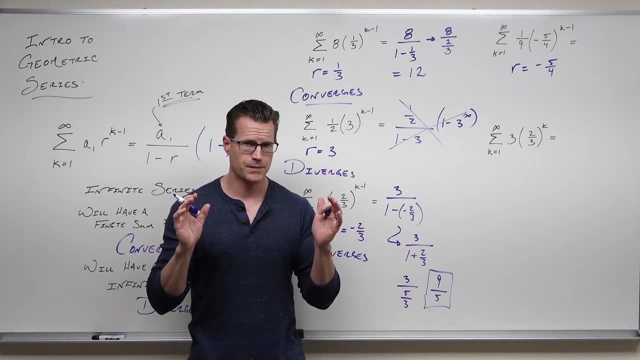 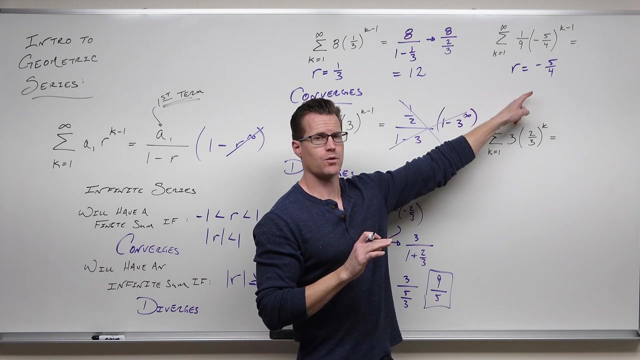 the thing being raised to the exponent. We identify that first, always. Then we classify it. Is this common ratio between negative one and one, or is it outside negative one and one? In other words, is the absolute value less than one or not? Well, the absolute value of this is five-fourths. 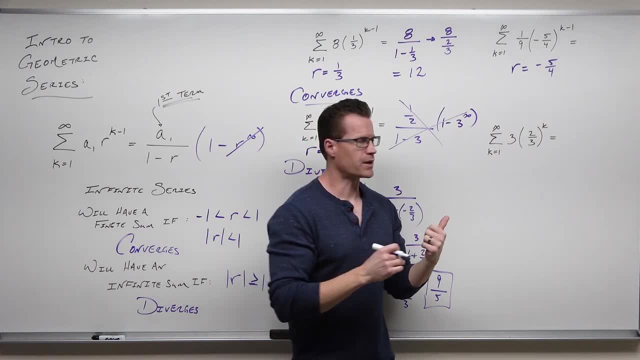 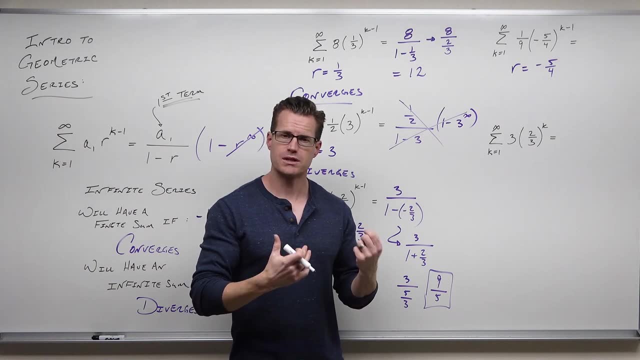 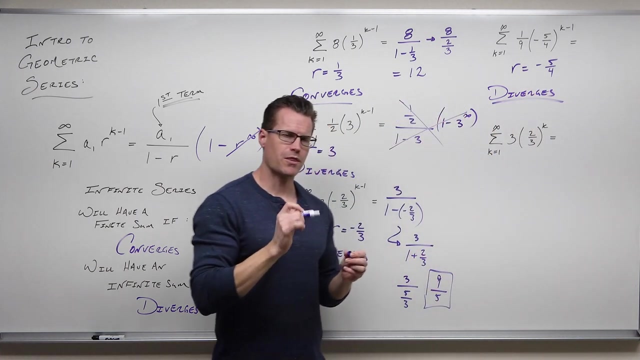 Five-fourths is one, Five-fourths is one and one-fourth. This is greater than one in absolute value, or it fails to be in our interval from negative one to one. This is not going to converge. This diverges. We always determine that before we find the sum. 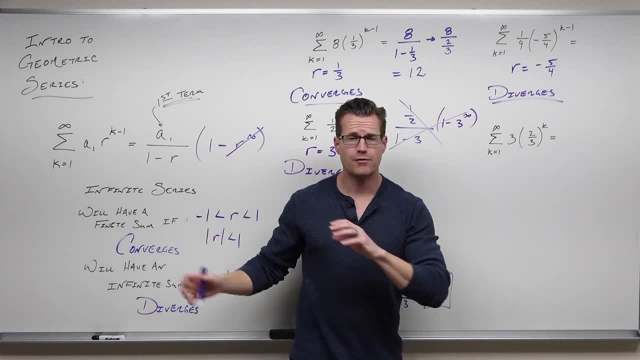 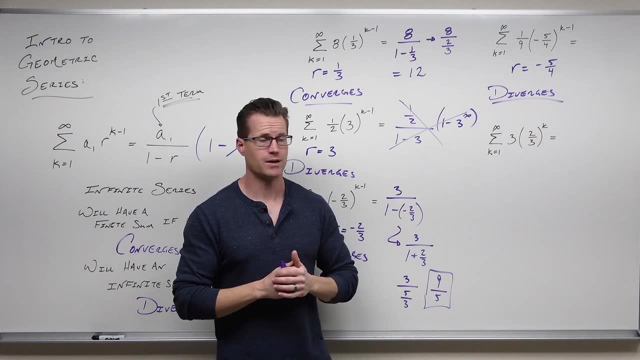 So at this point, here's what this says: If your common ratio does not fit a convergent model and it diverges, then we say there's no sense in finding the sum, because this is either going to be positive or negative infinity. 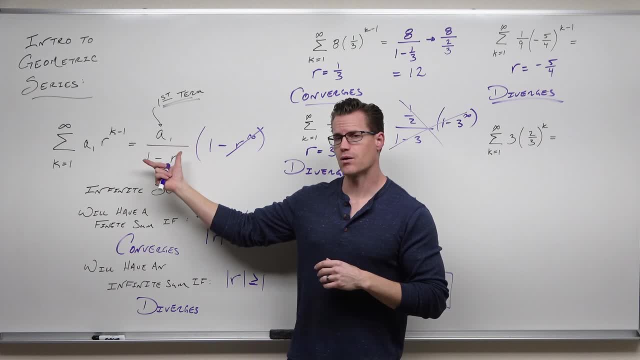 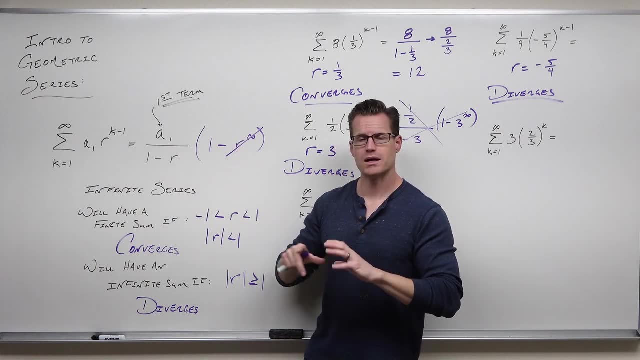 This is not going to add up to a finite number. Therefore, this formula does not work, because we'd be missing this piece and this piece would go to infinity. That's what happens when r is greater than one and you take it to an infinity. 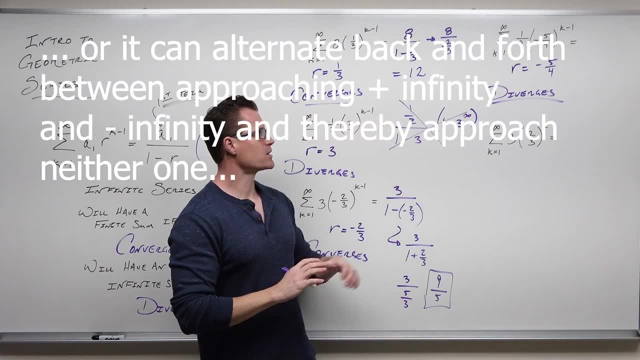 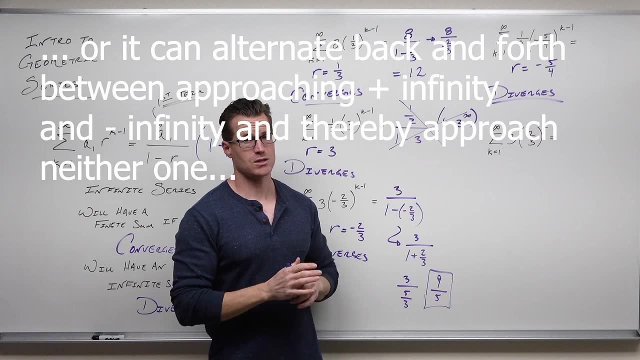 It goes to infinity as well, either positive or negative, And so this says: nah, we're not going to get there. That diverges. Don't go any further. Don't use this formula, because it doesn't make sense to do without that piece, and that piece says infinity. 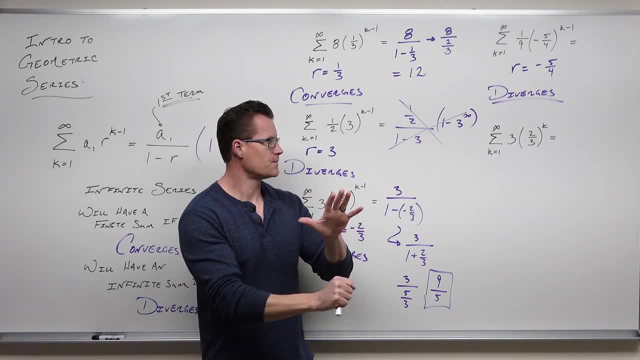 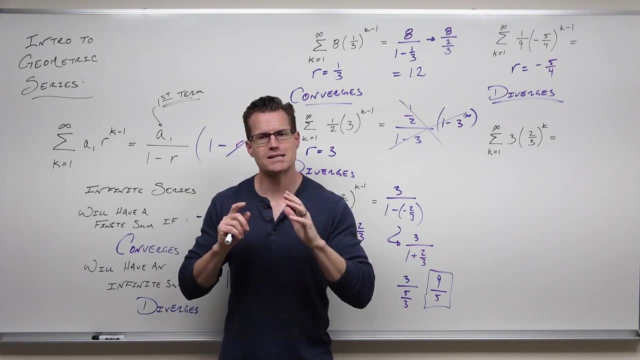 Last one, So the sum from one to infinity, of three times two-thirds to the k. Let's identify our common ratio first. Notice it doesn't have to look exactly like that. Our common ratio is just the thing that's being raised to the exponent. 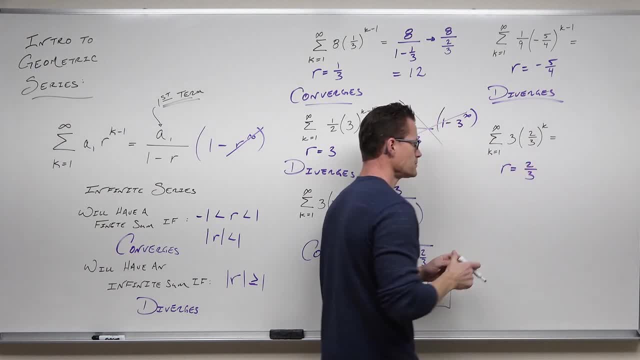 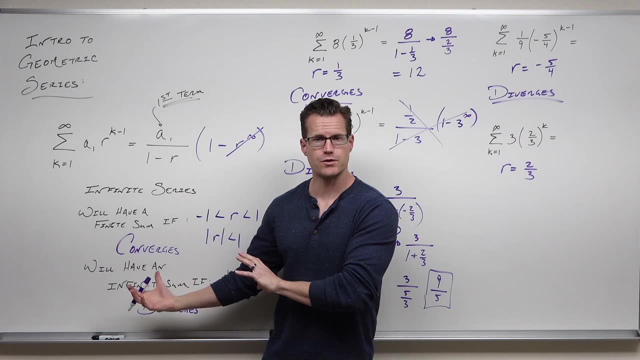 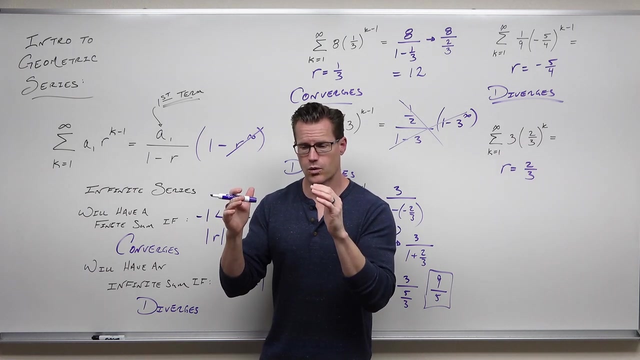 It's two-thirds. Well, let's classify that. Does that fit in converges or diverges? Think about it If two-thirds is our common ratio and that's between negative one and one, or that's a fraction less than one in absolute value. 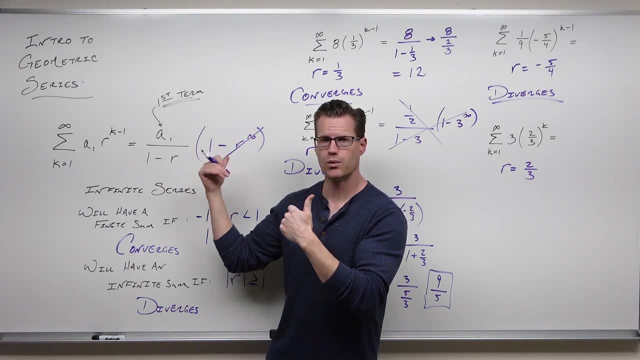 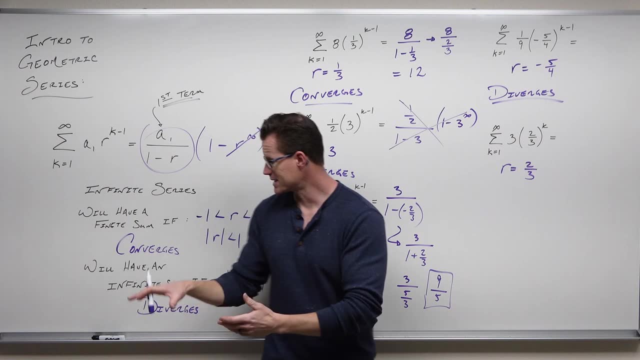 then when I take it to infinity, it's going to go to zero. One minus zero is one. This falls out. I get this as my formula. That's exactly what we're looking for. So we say, yes, this does converge. 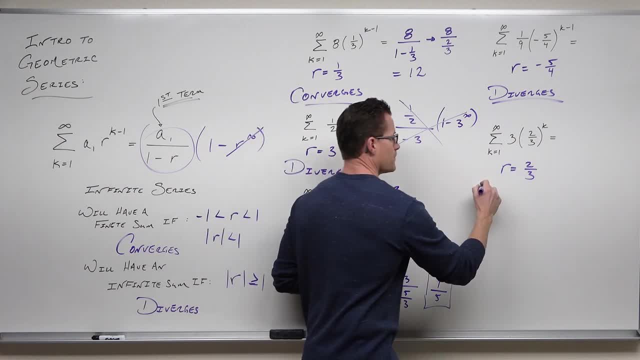 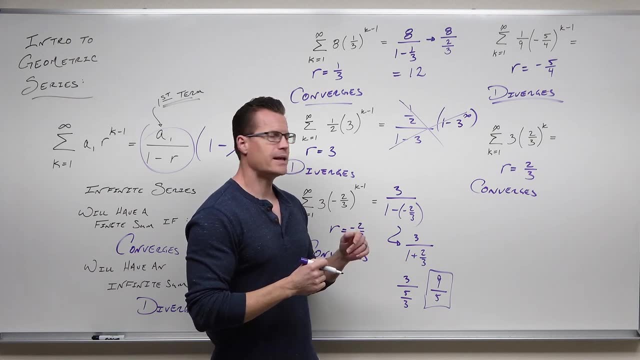 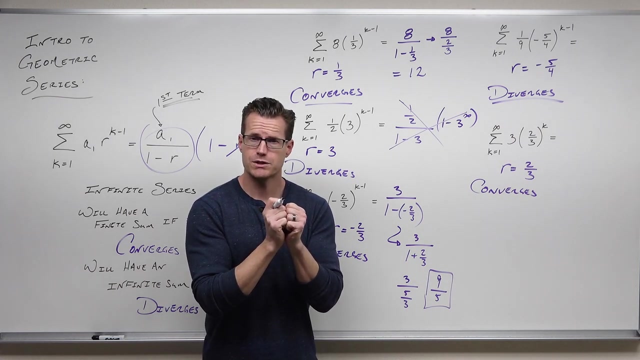 That's exactly what this says. Our common ratio in absolute value is less than one. It is going to add up to a finite sum. That's really cool, And now we can find it. All we have to remember is that when you're adding this up, you need to find your first term and put it on your numerator. 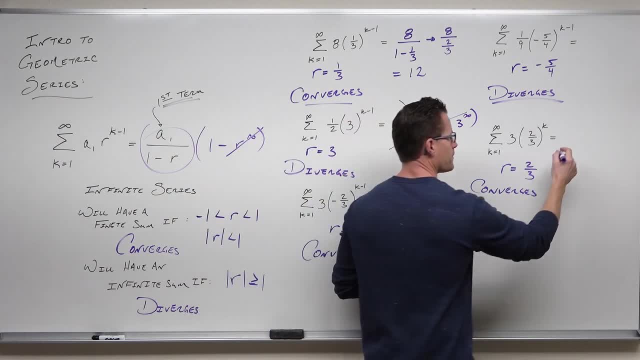 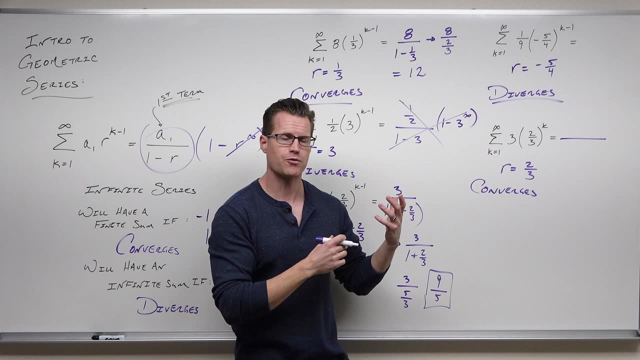 That's what that says. That's why I put first term there. So your first term is not three. Now, I've been prefacing this with every example we've actually found a sum for. but I always do this: I take one and I plug it in. 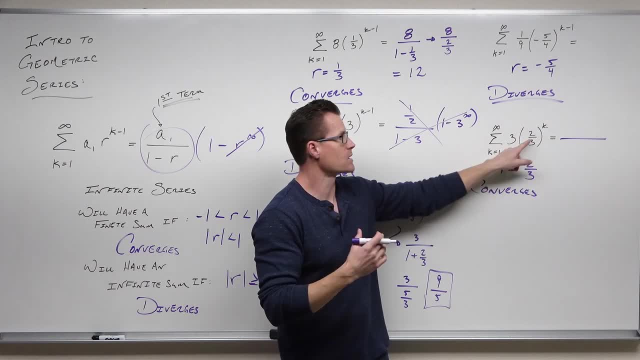 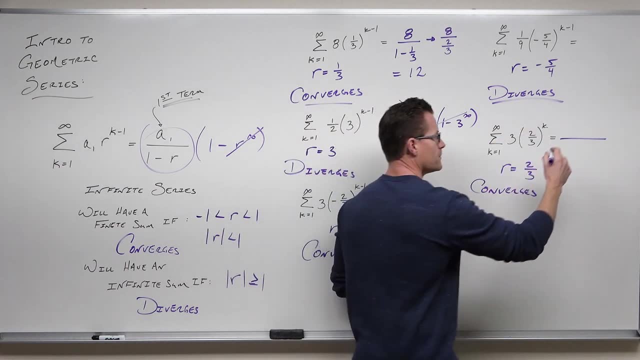 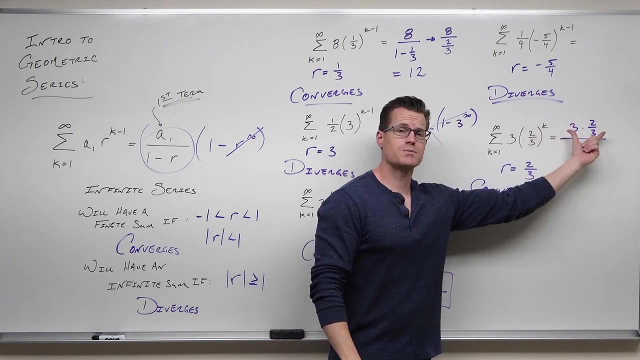 Whatever you get is your first term. That's what the one means. So if I plug in one, I get two-thirds to the first power. Ah, not zero, Zero power. I get two-thirds to the first power times three. So this, when I plug in one, is my first term. 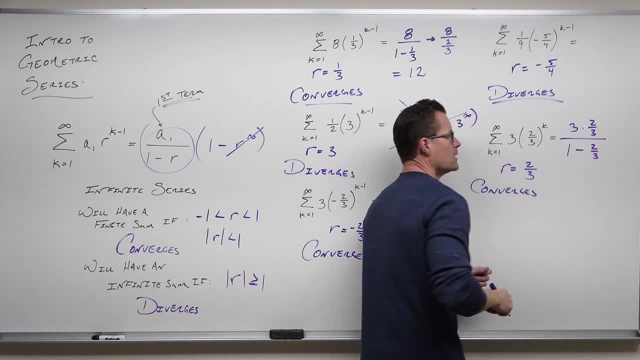 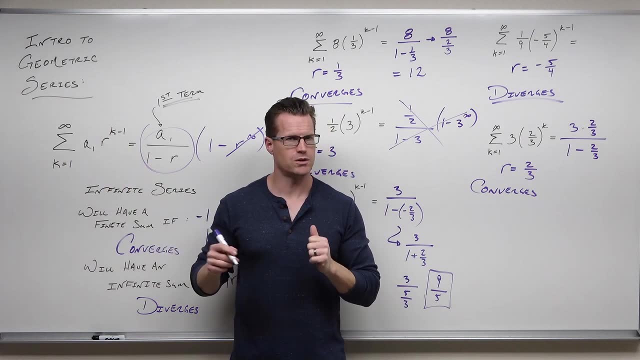 And then one minus r. Could you take the time to manipulate this to make it fit that model exactly? Yes, and I showed you how to do that in the previous example. I'm not going to do that. I really am not this time. 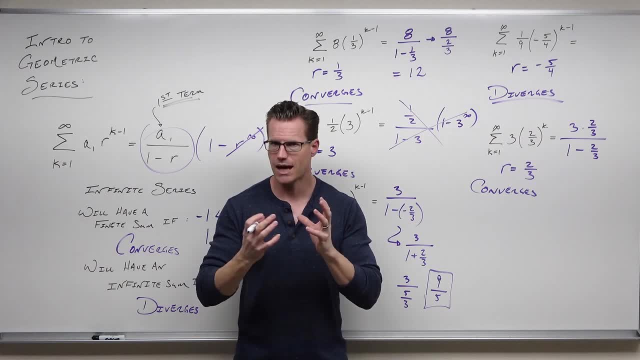 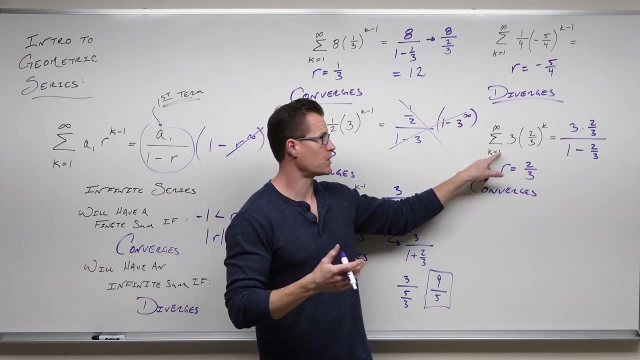 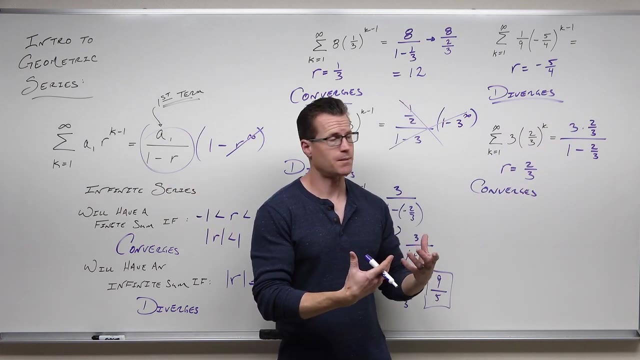 Because it's a lot easier. So let's understand what this is talking about. What this is talking about is take your first term, whatever it is. How do you find your first term? Plug in that number. So if I plug in that number and take that on my numerator, divide by one minus your common ratio, take that on my denominator and then simplify it. 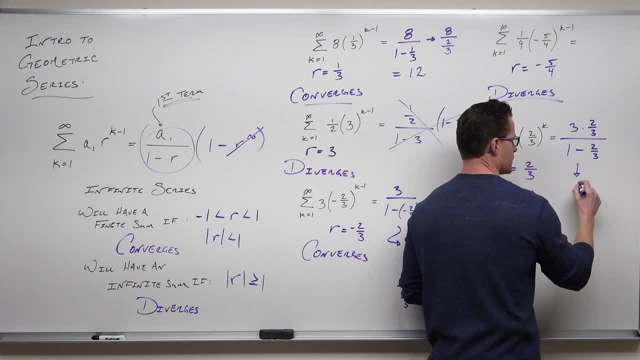 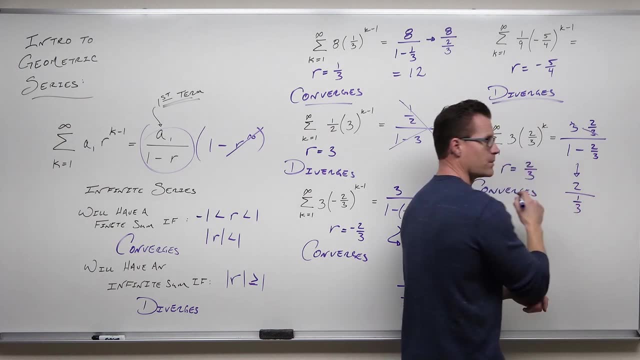 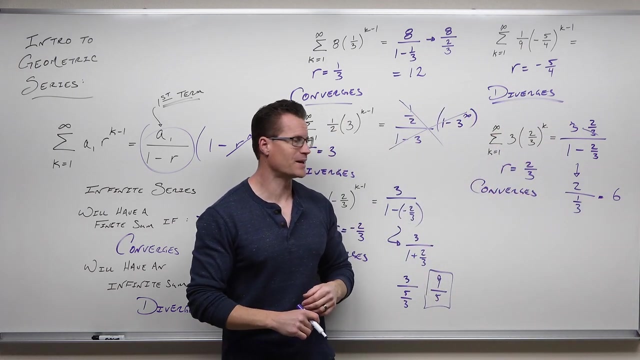 So three times two-thirds is two over one-third. One minus two-thirds is one-third. That's going to give me six. So if I add up all the terms from one to infinity, I'm going to get exactly six. I hope that you had a little. I hope you had fun. 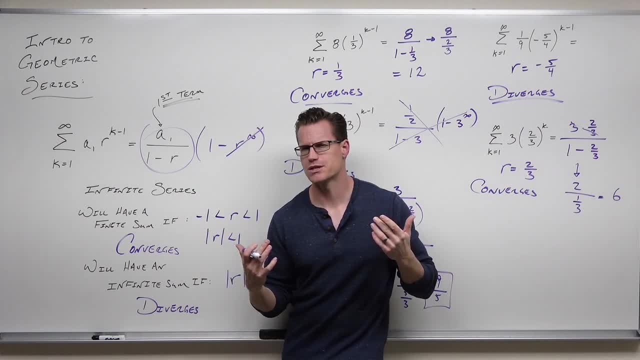 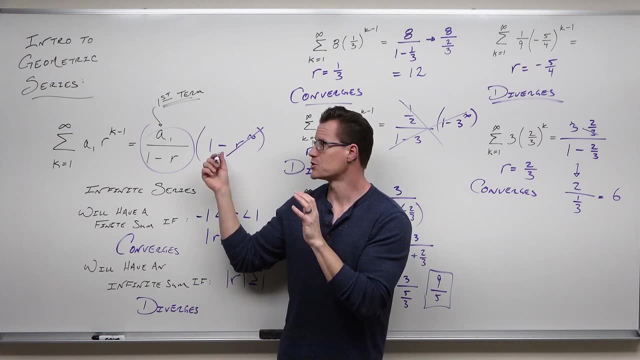 I hope you enjoyed thinking about the infinity and when that would go to zero and when it wouldn't, And how that affects going from a partial sum, where that is, to an infinite sum, where this either goes to infinity or it goes to zero, depending on what your common ratio is. 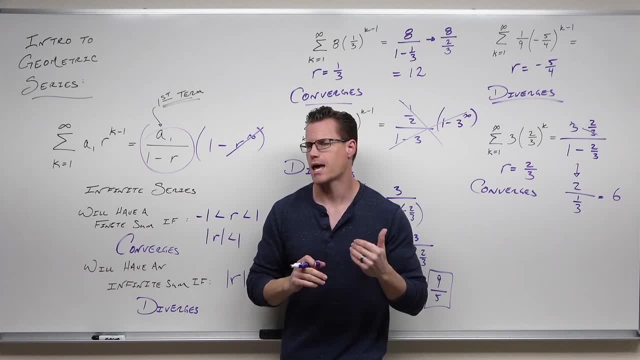 I hope it made that make sense that you really really see it. If you can, then this, this really: if you've taken calculus two, you will understand how this idea will really help you there, Or probably would have helped you if you would have known that before taking calculus two. 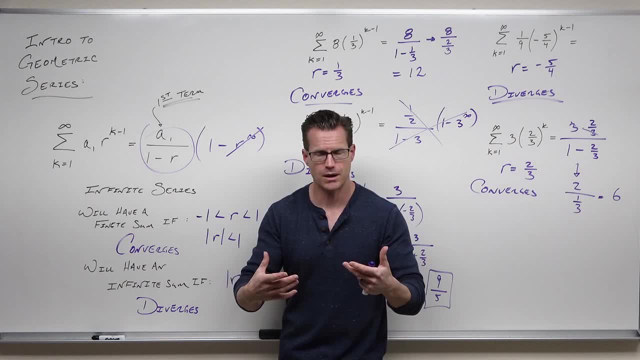 So if you're, you're going to get there eventually. When you get there, this idea of understanding how infinity works with fractions can be very, very, very valuable, which is why I'm teaching it to you now. So hopefully I've explained it in such a way that you understand what's going on with that, that formula. 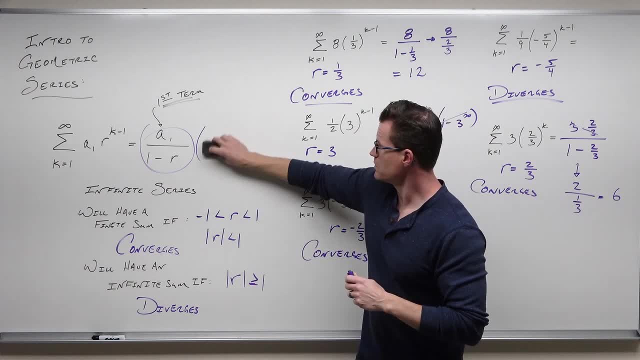 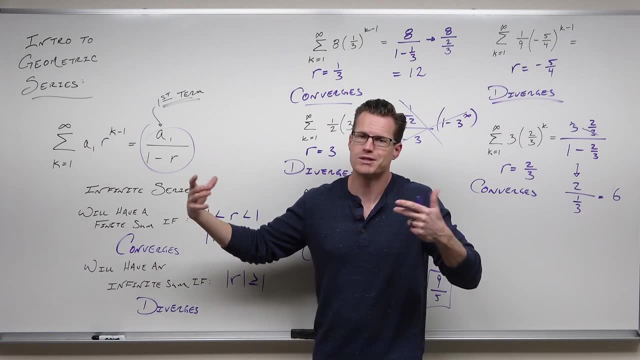 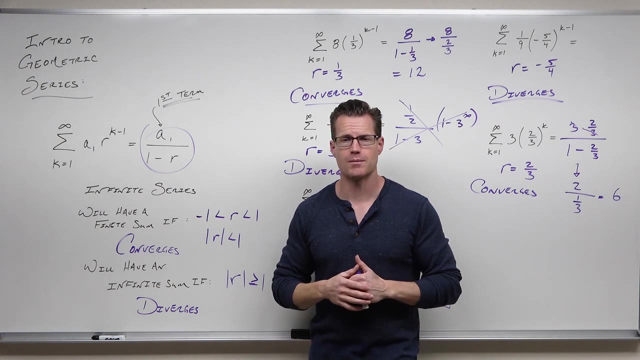 I know that your textbook will not show this to you for an infinite series. I did so that you understand where it's coming from in relationship to a partial sum which they show a little bit differently, So I hope you enjoyed it. I hope that you got the concept and I want to see you for the next video when we talk about proofs with mathematical induction. 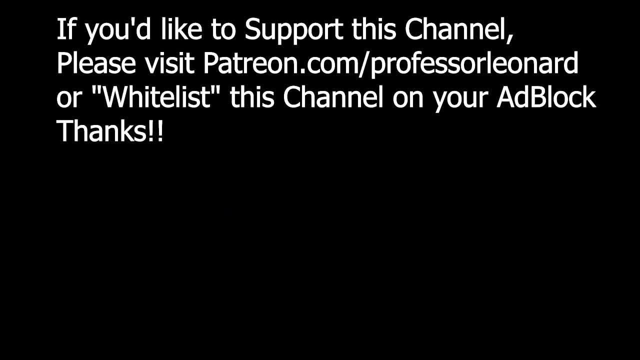 Have a good day, Thank you. 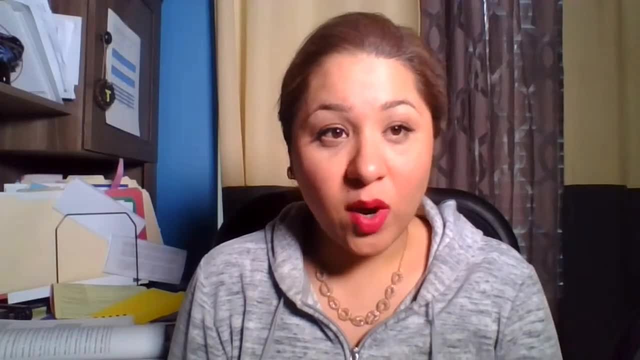 Hi, I hope you guys are doing well. Welcome to my one minute PMP. Today I'm going to talk about the difference between parametric estimating and analogous estimating. So what is the difference? A, you want to understand that they're both forms of estimating. So anytime you see it, 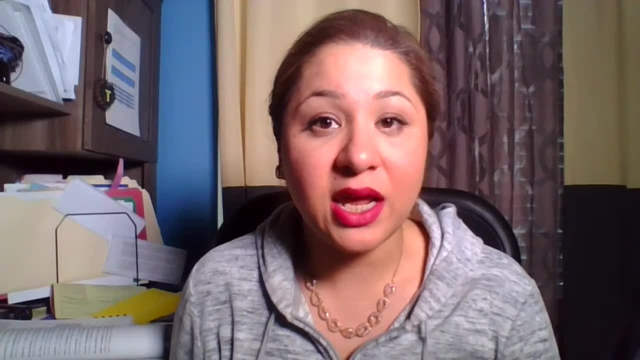 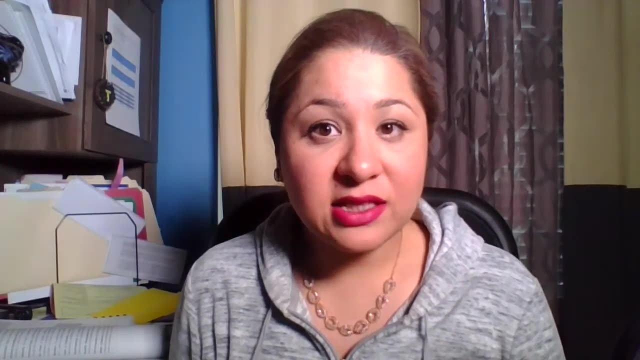 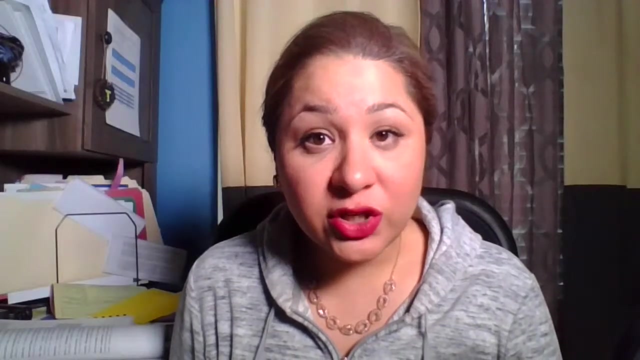 and you're going to see it in resource estimating, cost estimating, schedule estimating. So it's a common tool that is used And the definition doesn't change, no matter which process you're talking about. So it is a form of estimating. Parametric estimating is a form of estimating. 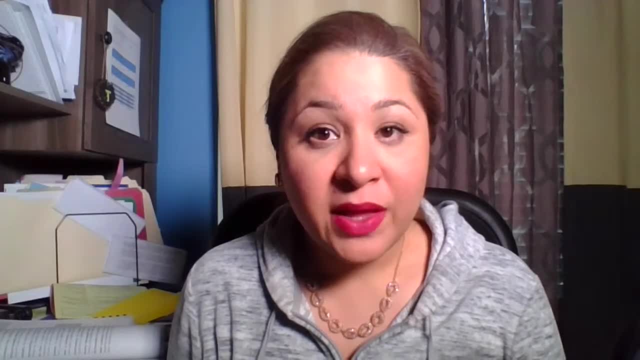 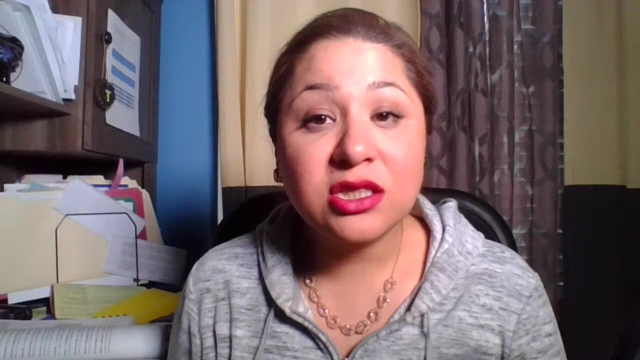 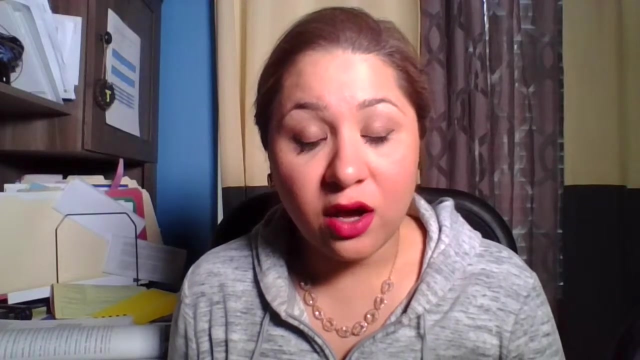 where you're using historical data. It's a data driven form of estimating, very accurate. It takes a long time And it does cost a lot of money to do it. However, it gives you a lot of accuracy- The other way of knowing what parametric estimating is. it's also known as form of